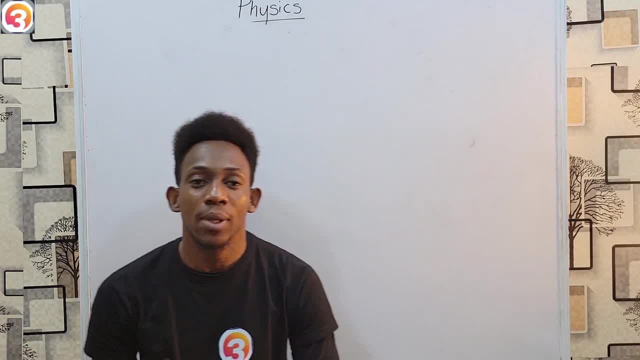 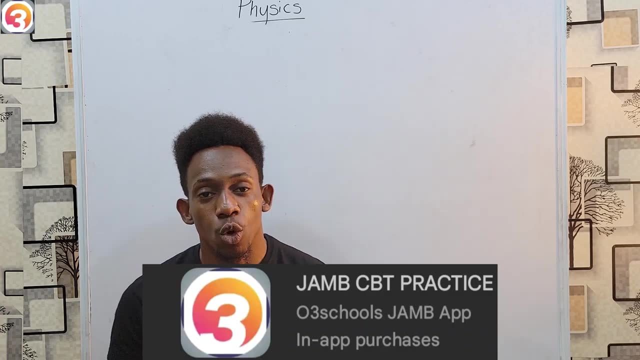 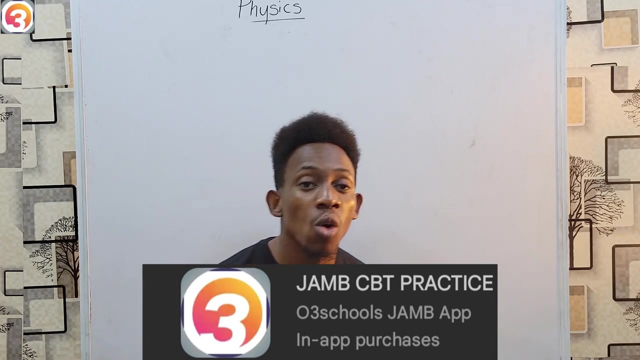 Well, hello again there. Welcome to today's Jamf class, presented to you courtesy of all three schools Jamf app, the only app you require preparing for your Jamf. The app has a wide range of features designed to ensure you get the best possible score. that. 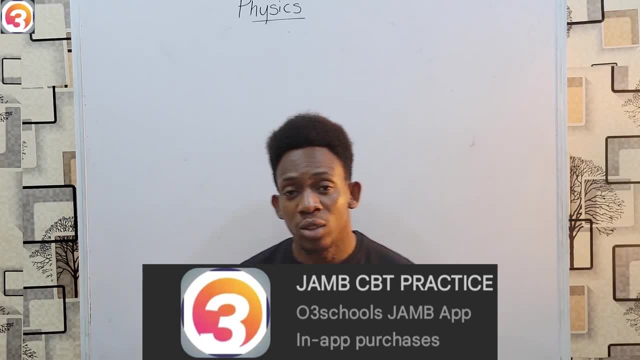 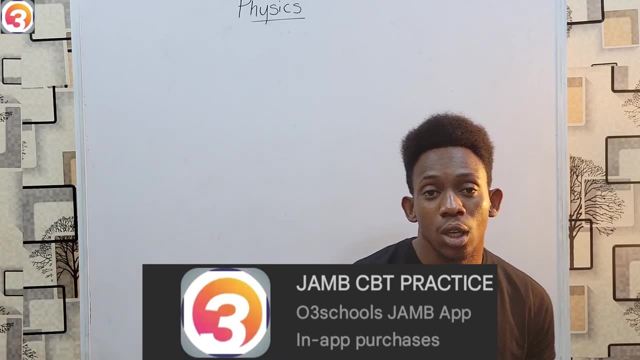 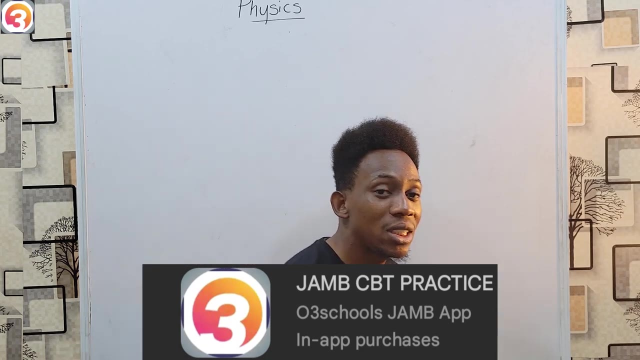 you can get in your examination Now. all you have to do simply download your app on either your android phones or your windows laptop, install this application and if you install it, you notice first of all that your options, what you can do, this app is limited, but then you have. 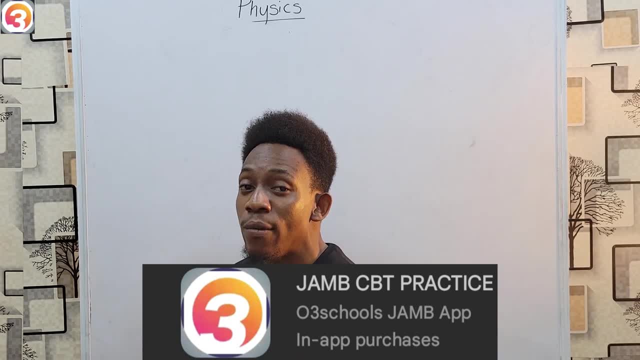 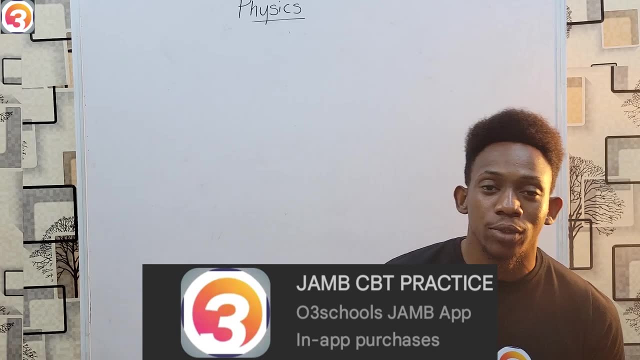 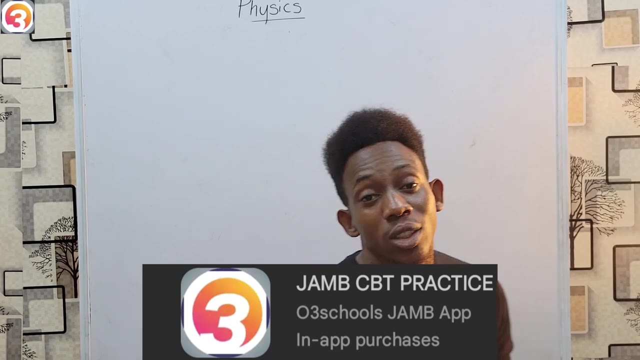 to activate this app. Activation costs 2500 naira only, no more. and once you activate this app, you shall get access to all the features as provided in this app. There is information there: advice on how to choose your schools, the courses offered by the schools, the subjects you require for those courses. You also have 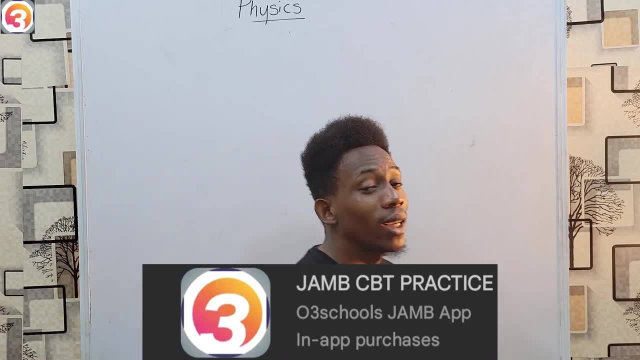 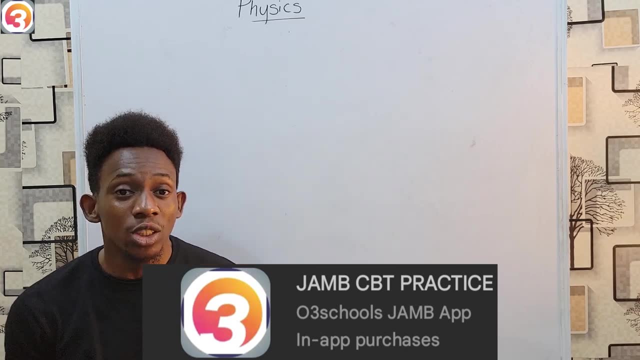 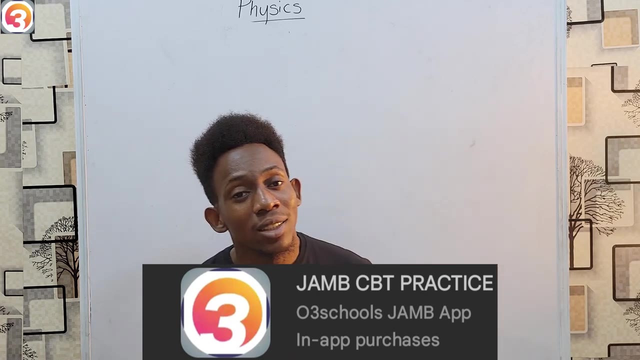 obviously your past questions. You can do it in mock exam mode. There's even a feature to search for questions per topic in each subject, such that as you read or as you learn anything, you still have to search for that particular question on your old three schools Jamf app and then answer. 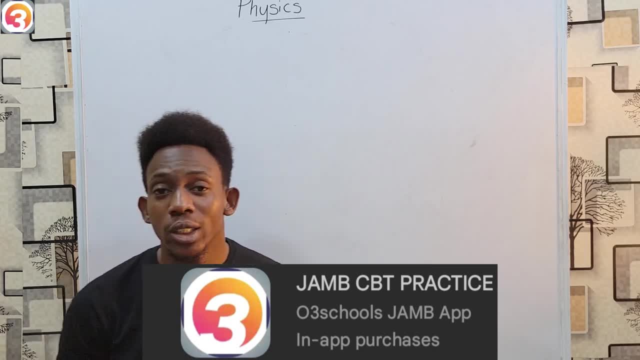 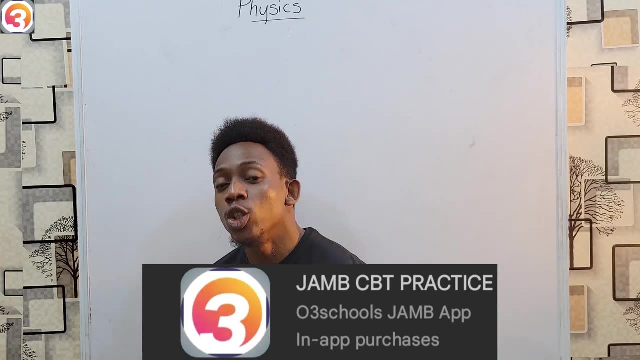 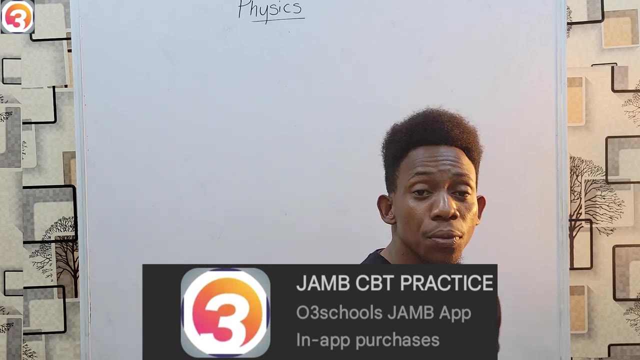 the questions in that topic. once you can answer all you know, you're ready. If you can't know, for that reason it might be necessary. See, the app has many useful features which will benefit you, and the activation is very simple. Simply follow the steps as you can see on the app. um, there's no reason to fear. 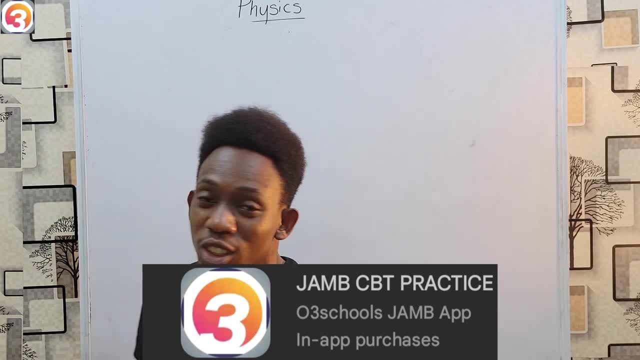 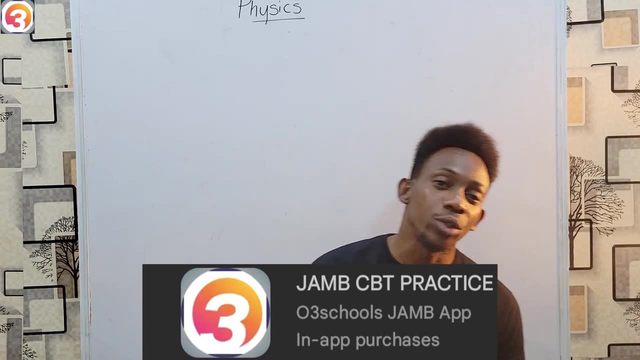 like some people would say that, uh, what if the peer and their money doesn't, you know, get used on the guest comes? I'm assuring you. yet I know this app is not like that. you've had negative experience Here. you shall have a positive experience. O3 school Jamf app is the way. 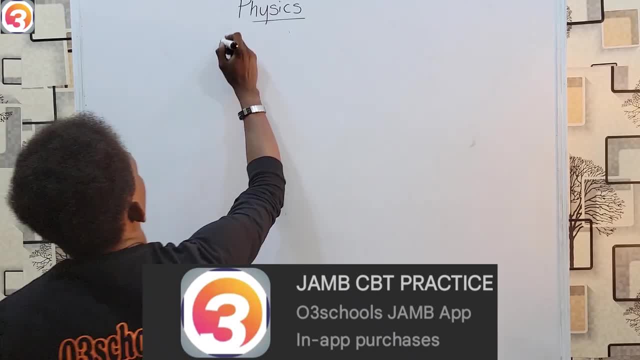 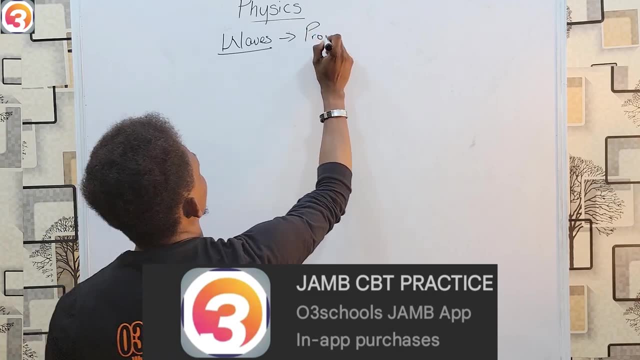 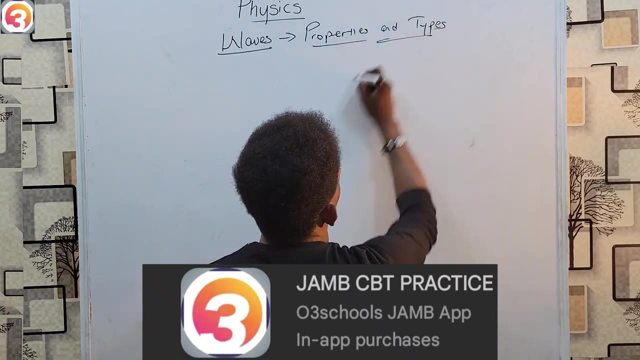 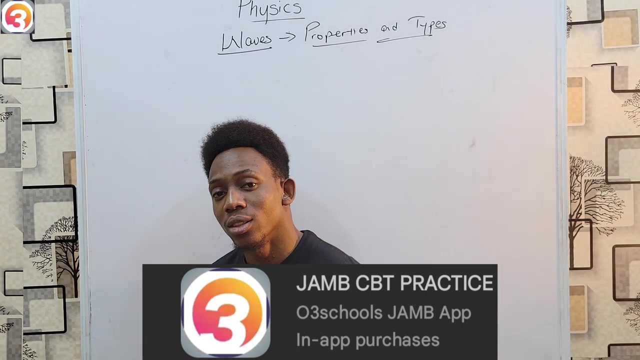 and with that let's just start this class. we shall be looking at waves, and in this class you'll be studying properties and types of waves. okay, now, first of all, what is a wave? a wave is a disturbance which travels through a medium propagating energy without 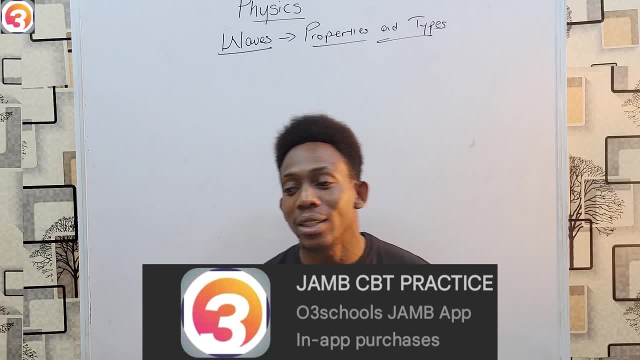 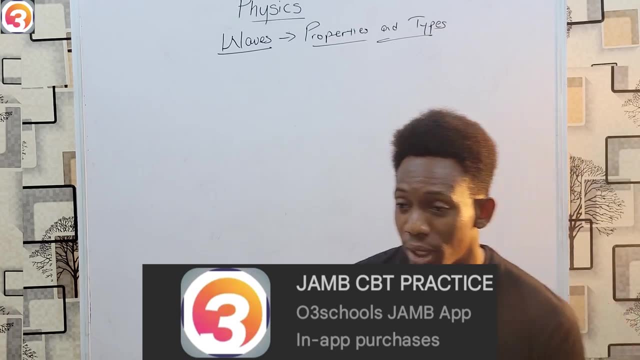 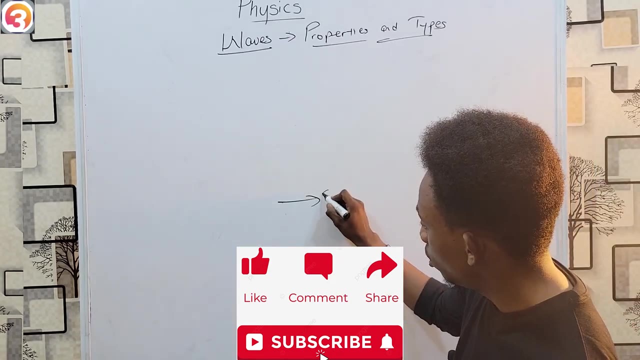 causing a permanent displacement of the particles of that medium. now this might sound like grammar. what is a wave? simply, in the simplest manner, you simply have a disturbance, a shake, if you will. that then moves through a medium and as it moves it is transferring energy. but what makes it special is that, once it transfers its 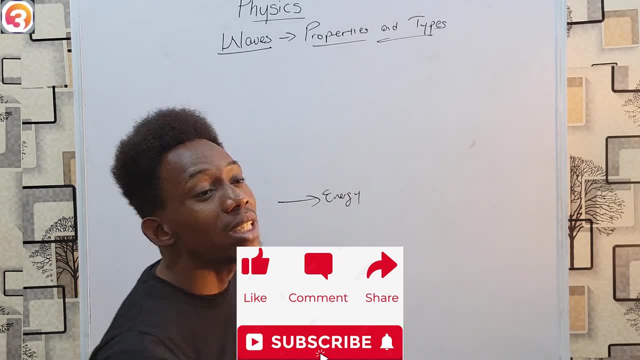 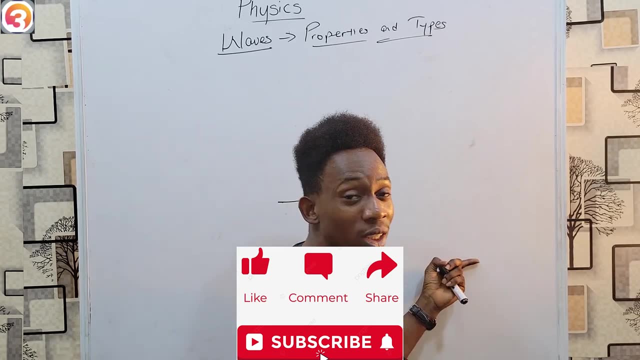 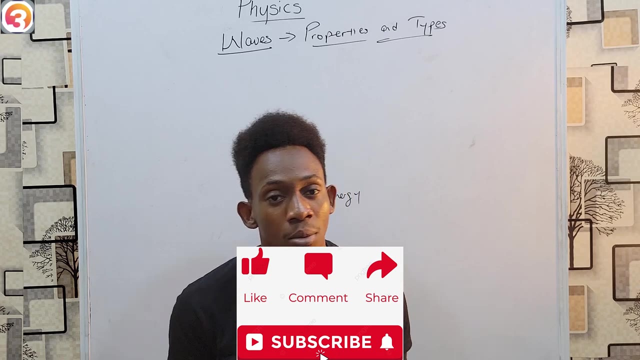 energy through the medium. it doesn't cause any permanent displacement of the particles of that medium. if I use a wood, A piece of wood, to heat someone, for example, imagine I transfer energy. yes, kinetic energy from my hand is hitting him. before that motion, he moved. I transfer the kinetic energy from the stick to him. however, my stick was no longer where it was to transfer the energy. it has moved. 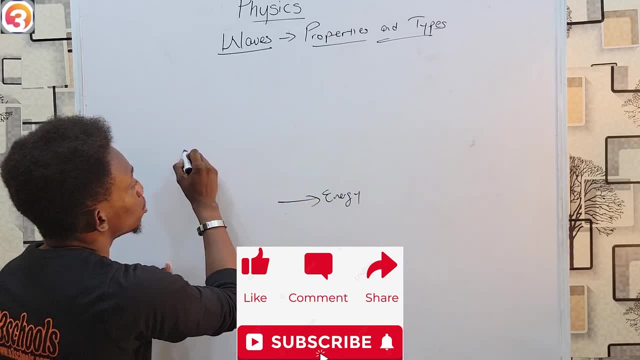 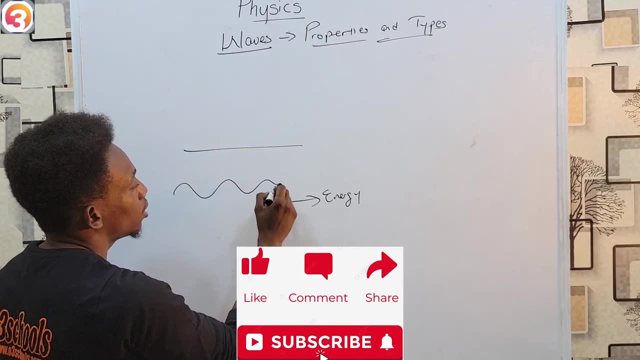 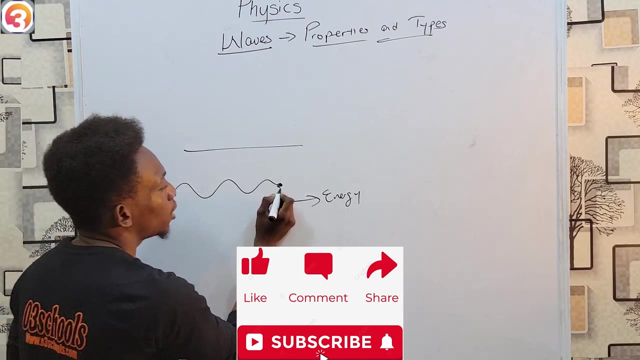 but in a wave, for example. imagine you take a rope and then you know you create free pulls in this rope by shaking the rope. if I have something here, that thing is going to flare, it's going to fall off. how cause energy was transferred from this point down there, but did my rope itself fully go anywhere? 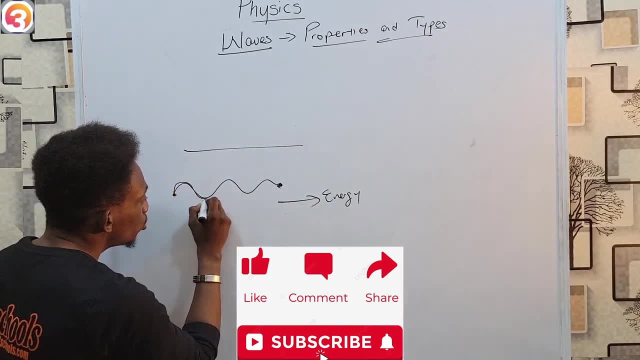 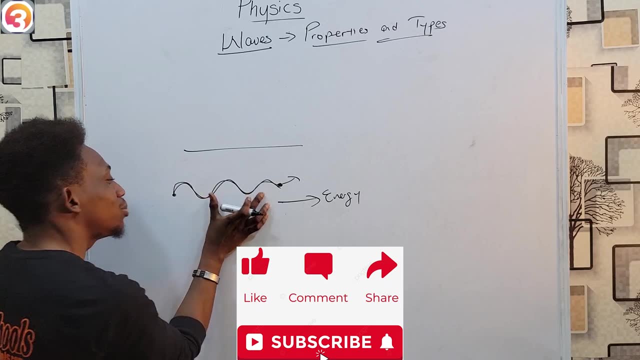 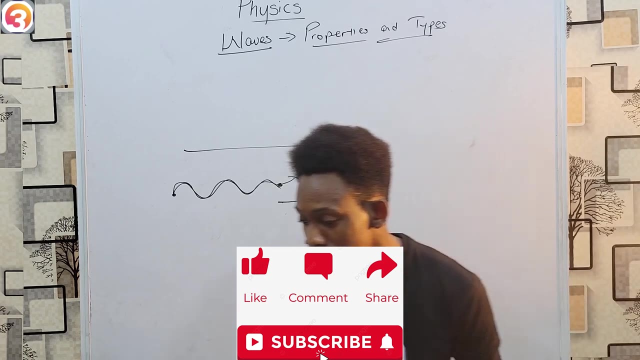 no now. energies traveled through the rope until it came here and moved. this energy was transferred without any permanent displacement of the molecules which make up this rope. see, and that is basically what a wave is now to study wave, obviously, the first thing you ask yourself is types of waves. but then, before you can, 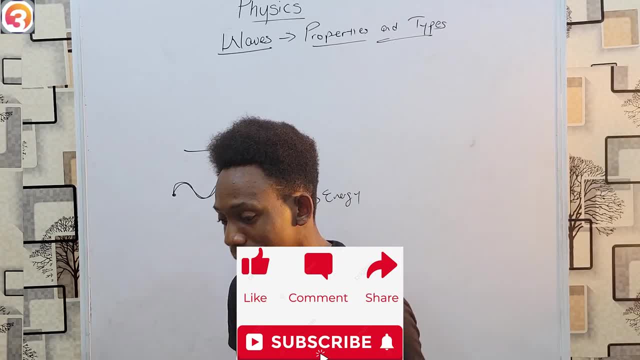 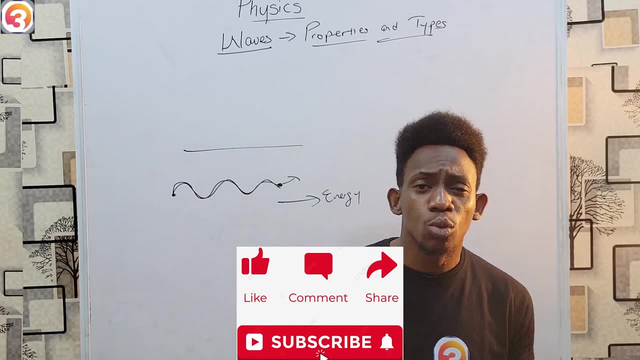 analyze this. lets ask yourself: what are their types? based on what? and in this case, as an example, is human beings. if I ask you types of human beings, you have to ask me: based on what? based on religion? now, you can have your christians, your muslims. 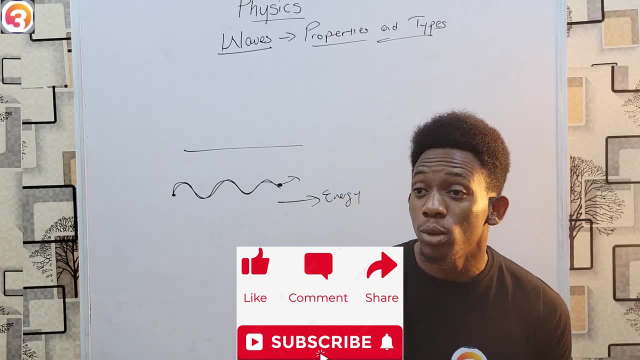 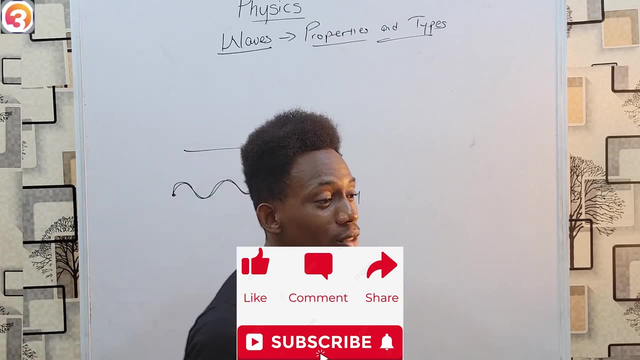 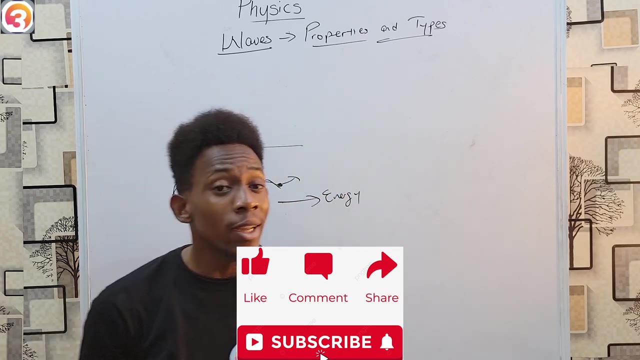 traditional worshippers based on color you mentioned, I like to say we have black. those are colors based on race. we have the ingo, the House, high European, all the other tribes based on gender and race. we have the white and the black and the red than male and female. and therefore, you see, before you can talk about type, let's ask yourself: 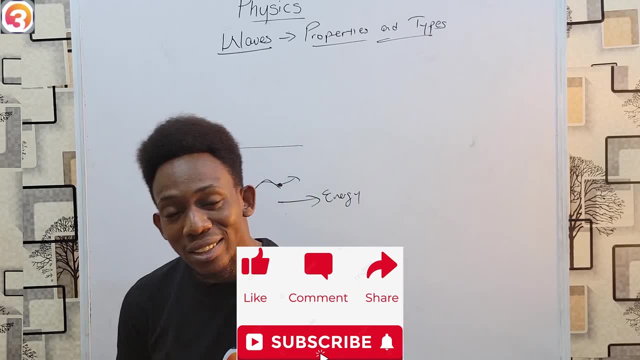 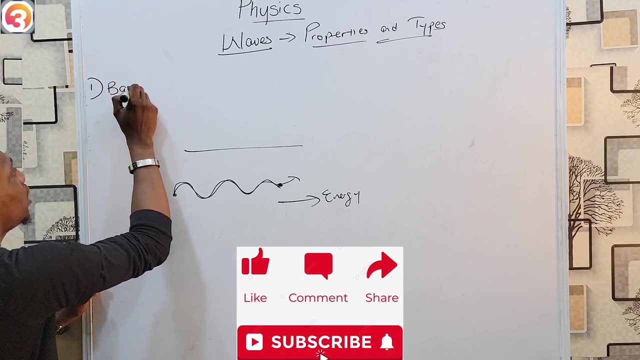 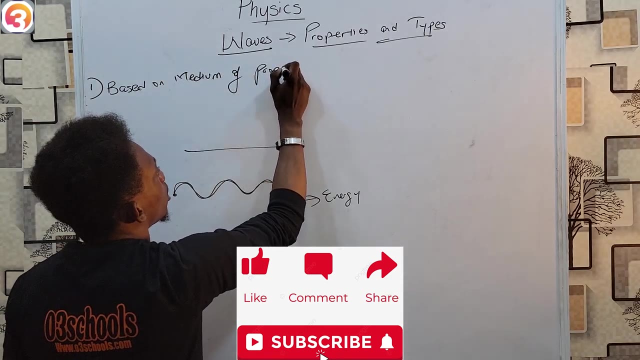 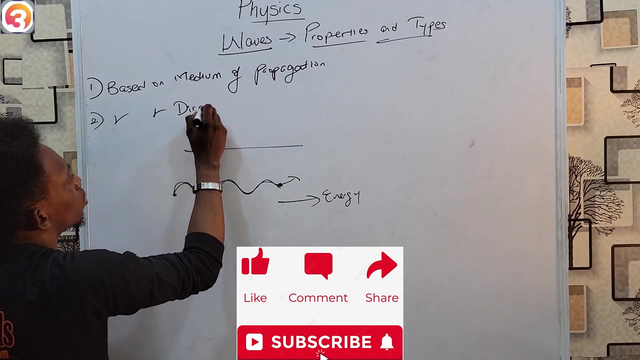 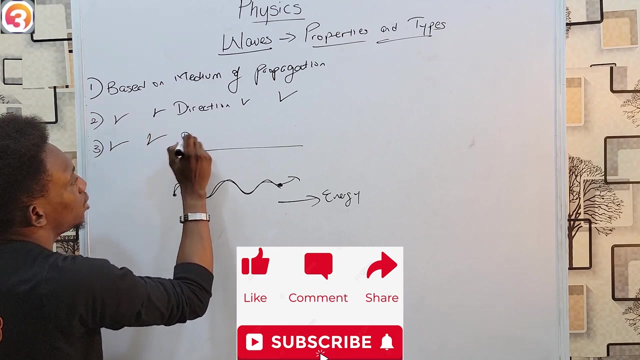 on what criteria am i basing these types- and in this case we also have that now- based on type. can i have one based on medium of propagation? that's the first classification, then two can also have based on direction of propagation and thirdly, we can also have based on distance being traveled. 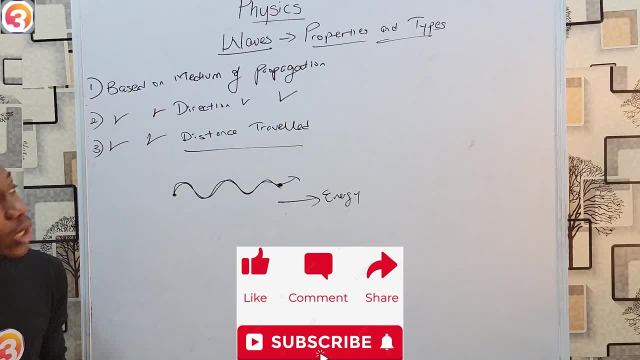 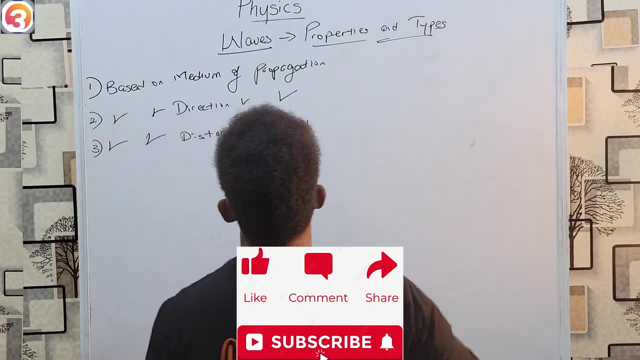 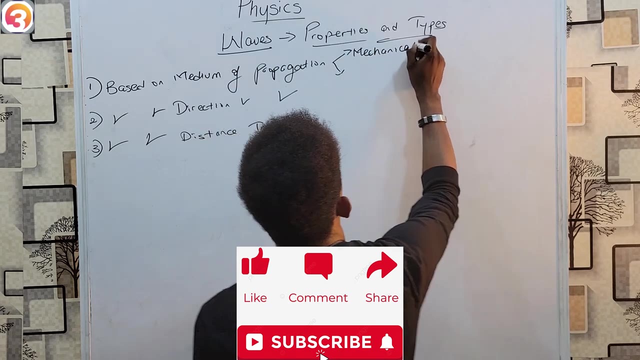 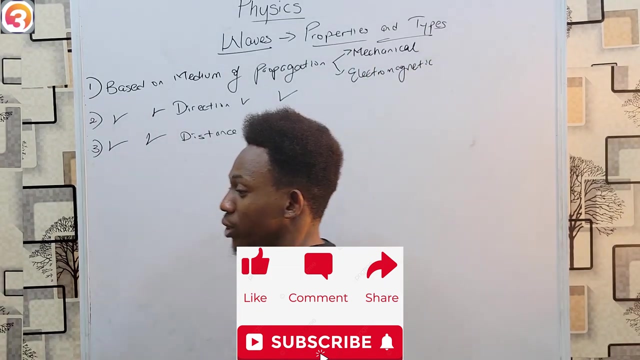 so those are the three criteria we look at when analyzing the types of waves. now, looking at the first step, based on medium of propagation, over here we have what is known as mechanical and the electromagnetic wave. now, what are the differences? a mechanical wave requires material medium. mechanical wave cannot. 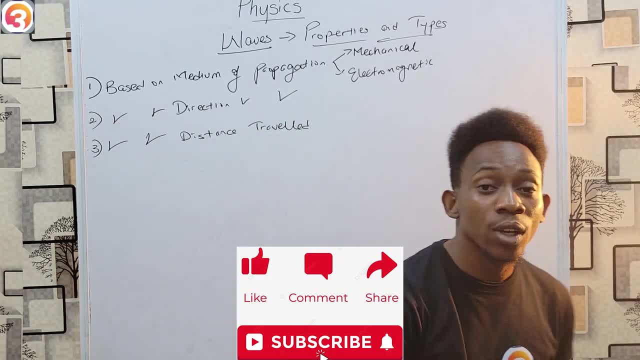 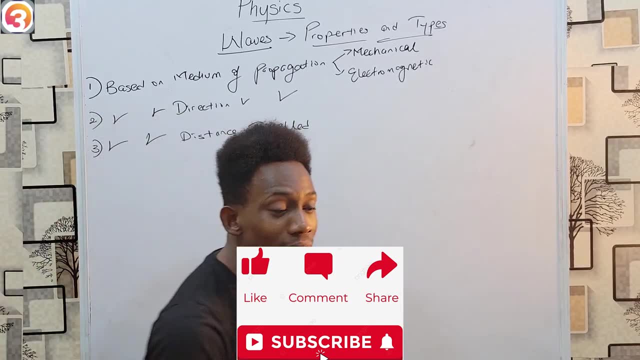 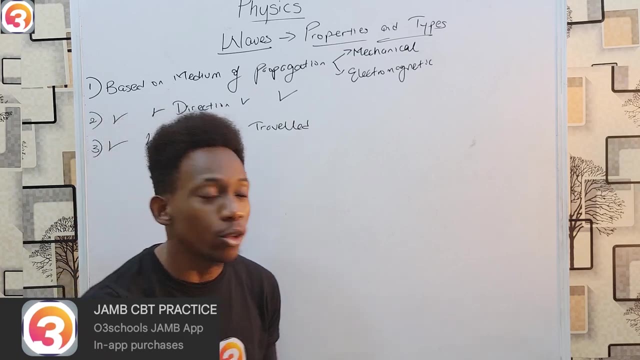 travel even if there is nothing for it to travel on. while electromagnetic waves do not require any material medium whatsoever, they're able to move without any object, without a roof, to travel on, in the manner of speaking, so mechanical waves. there are many examples: we have sound wave. 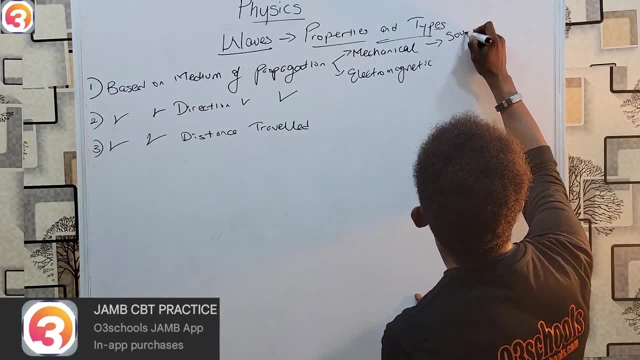 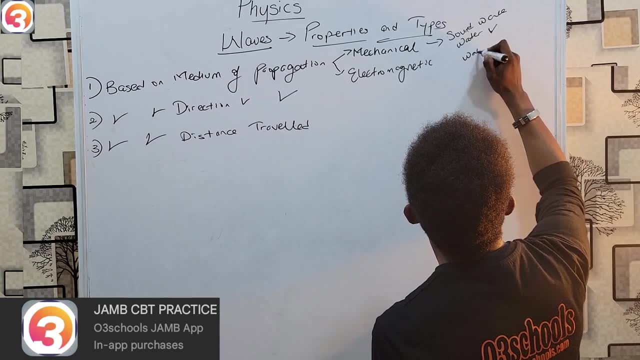 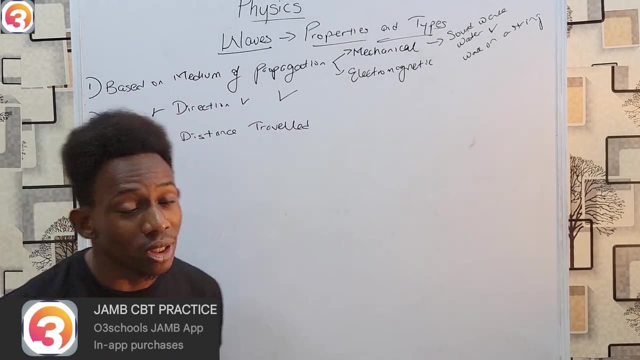 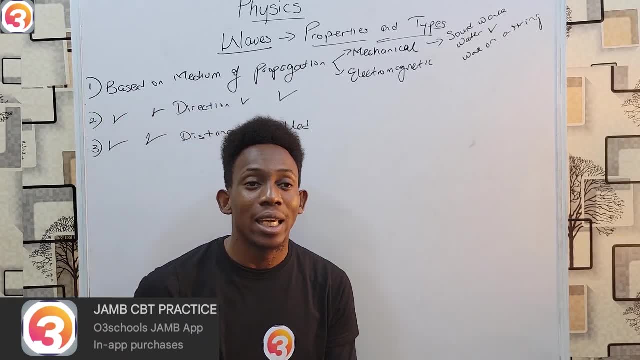 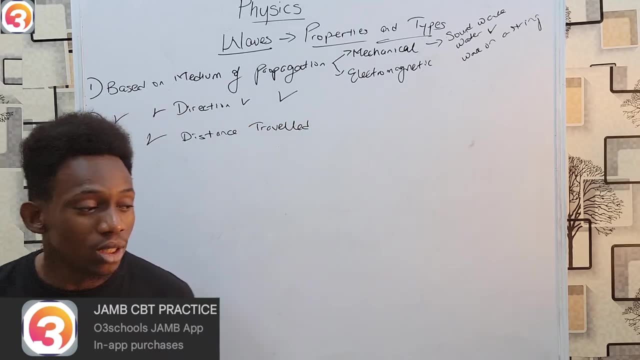 air around us, but sounds actually travels through the air, or through solid or through liquid must travel through something. if there was no area, then there should be no sound. therefore, in space there is no sound, unlike some of the movies we watch, where you can see this explosion in space. 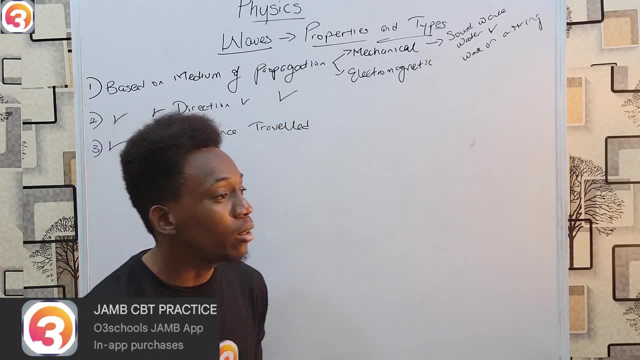 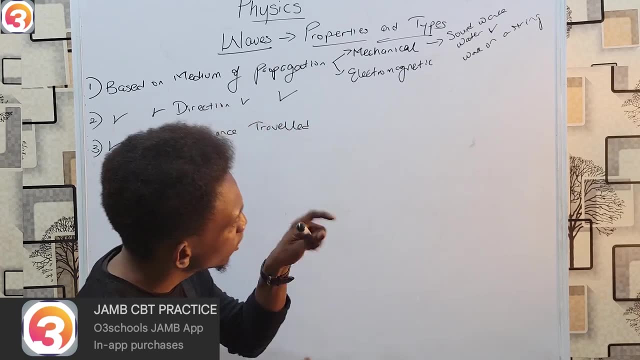 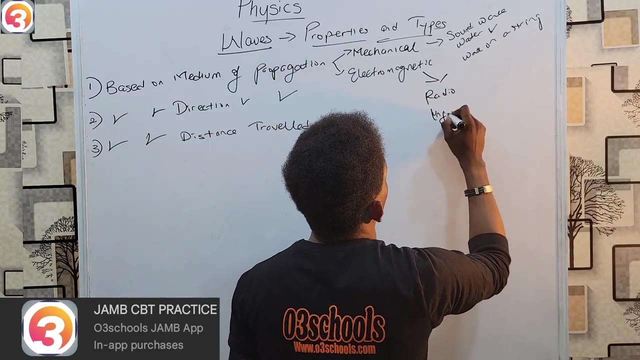 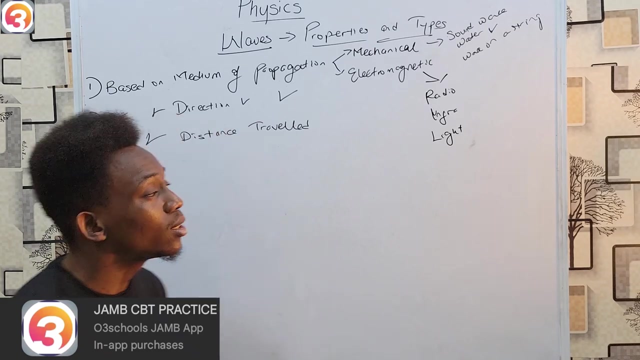 and you can hear sounds in natural space. there is no sound. everything is quiet because there is no particle or no material for this sound to travel through. while electromagnetic waves are quite many: there is radio wave, infrared wave, ultraviolet, your light wave, there's also x-ray and there's gamma rays. 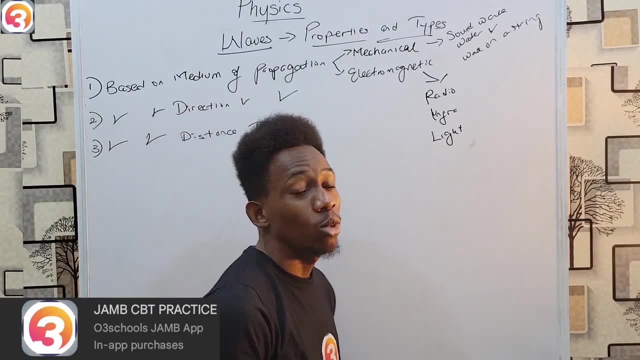 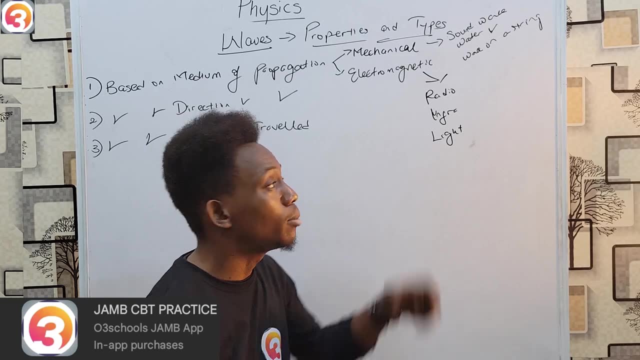 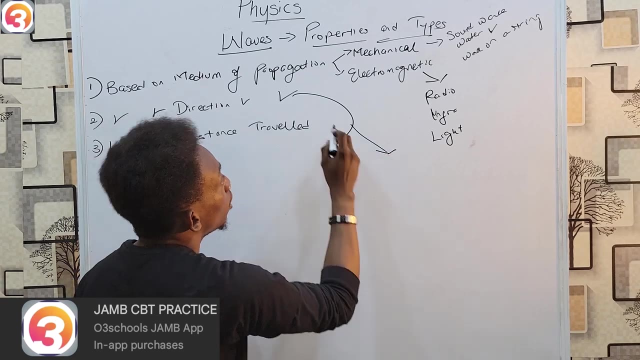 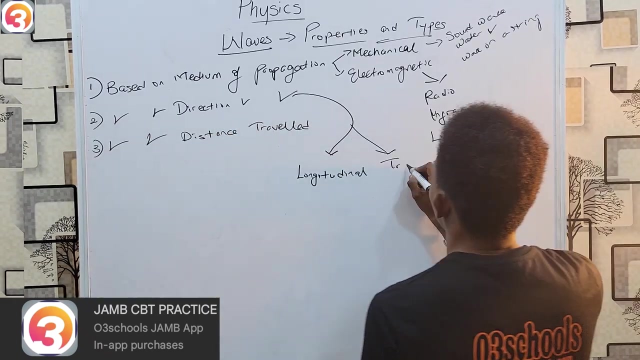 electromagnetic waves. this one does not require material medium whatsoever. for example, the light from the sun coming to it passes through space. where there's nothing doesn't require material medium. those are the difference. then, based on direction of travel, we now have the two types, which are longitudinal waves, only two dinner waves and your transverse waves. 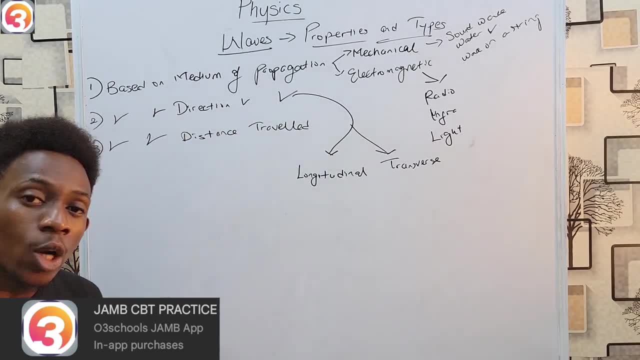 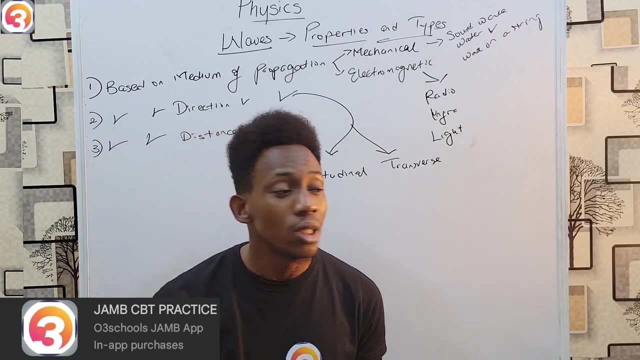 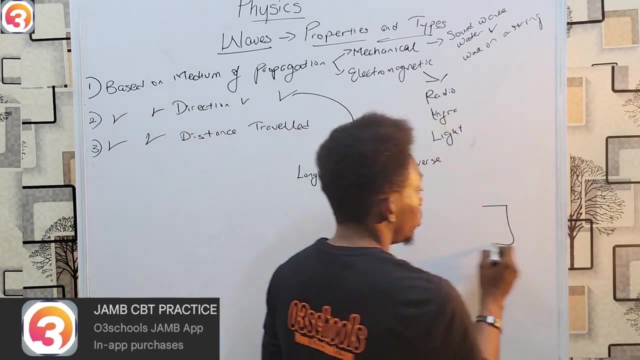 okay, again we look at the differences. now longer to the now wave travels parallel to the distortion which is causing it, for example, sound waves. if you have a speaker and the speaker is making sound, you hear the sound. basically, you put your ear, this is your speaker, you put your ear here, you hear the sound. 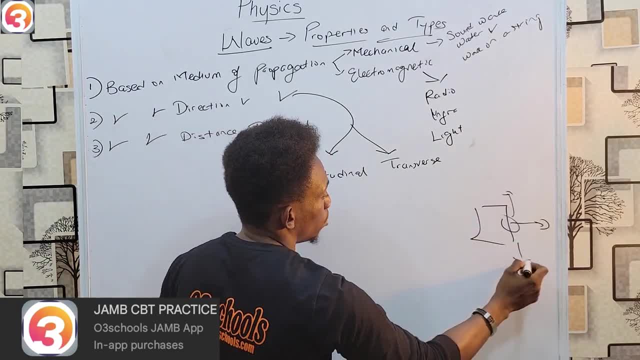 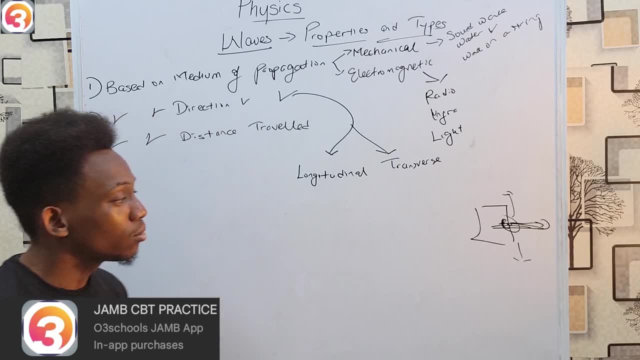 clearest in front of it than above it, or delete, because the wave is simply traveling parallel to the disturbance because i just speak out is causing it, because the wave is simply travelling parallel to the disturbance beside the speaker which is causing it, but the disturbance is causing it. 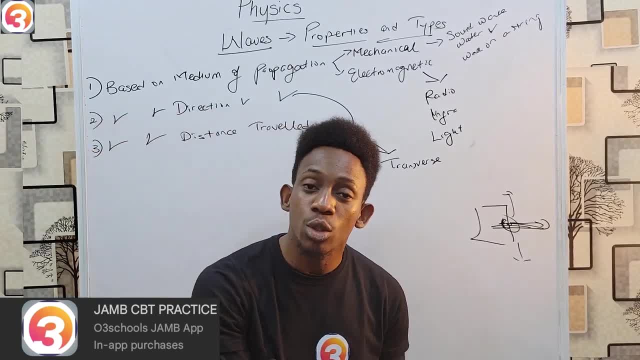 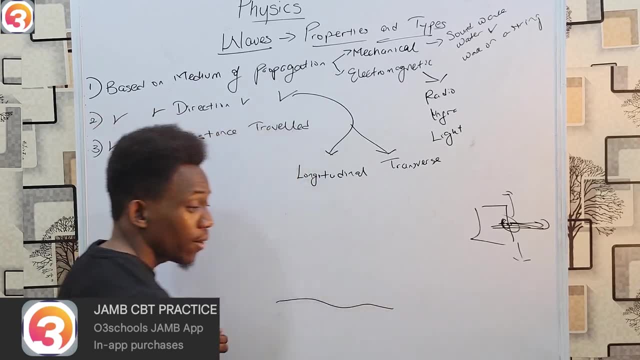 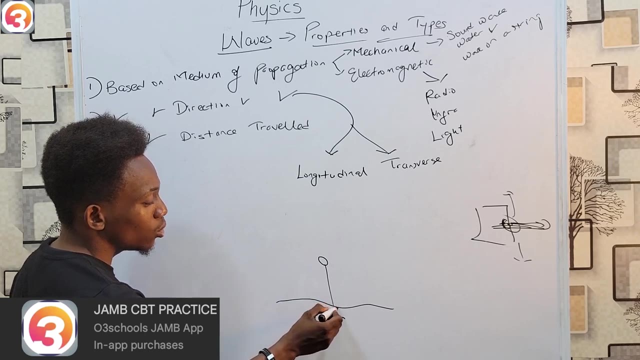 Transverse waves, on the other hand, travel in a direction perpendicular to the disturbance which caused them. A good example, which you cannot picture, is your water wave. If I have water here, if I drop a stone into this water, as the stone goes straight down, ripples are created in the water. 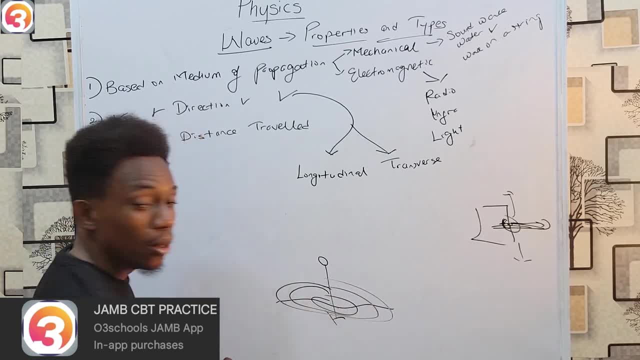 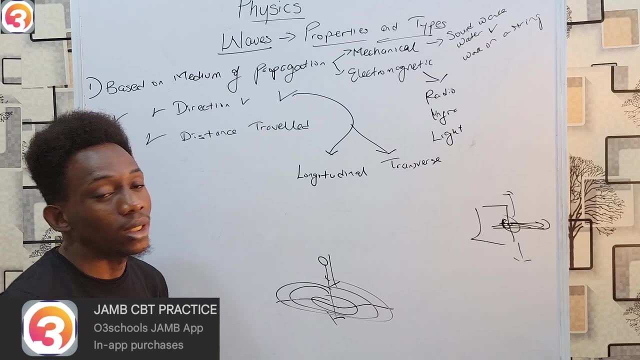 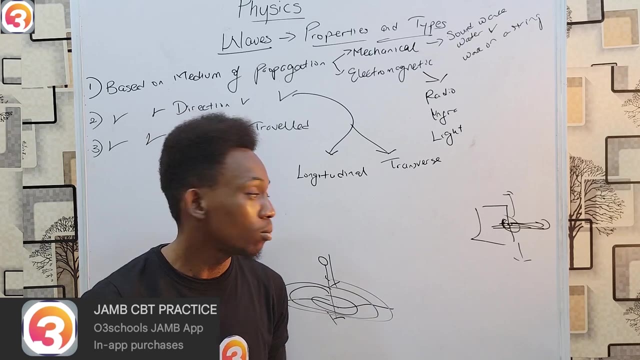 And where do they go Outwards like this? Therefore, the direction causing this was going down, while the waves were going perpendicular to it. So that's the difference: When digital waves travel parallel to the disturbance, transverse travel perpendicular to this disturbance. 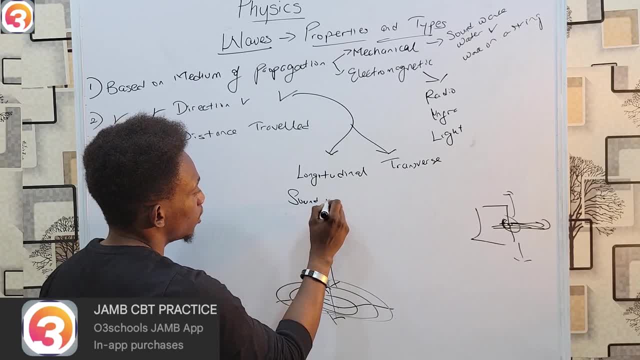 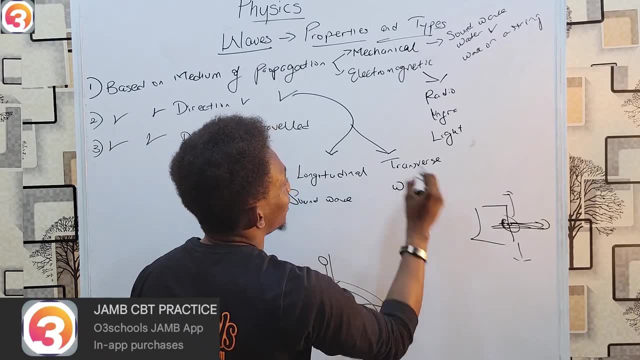 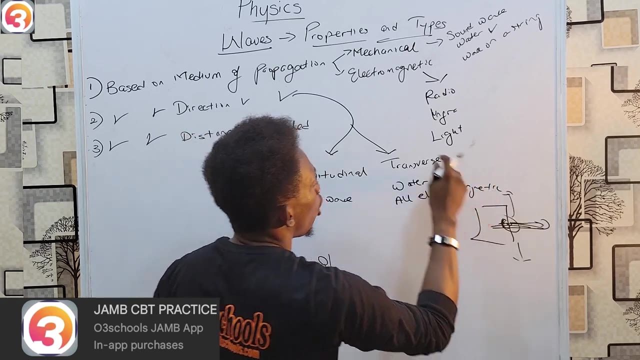 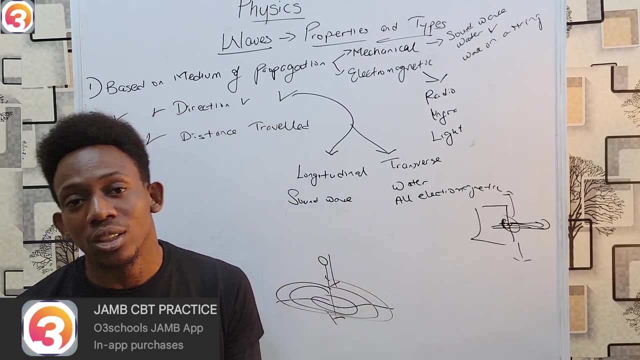 An example of a digital wave is sound wave. One good example of a transverse wave is water wave and simply all electromagnetic waves. So that's one thing to note. All electromagnetic waves are transverse, But not all transverse. All houses, like non-oags waves, are electromagnetic. 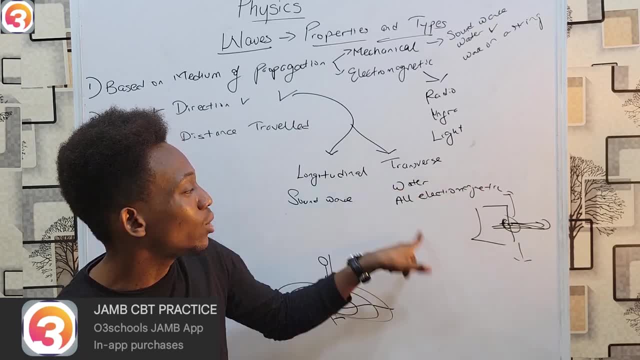 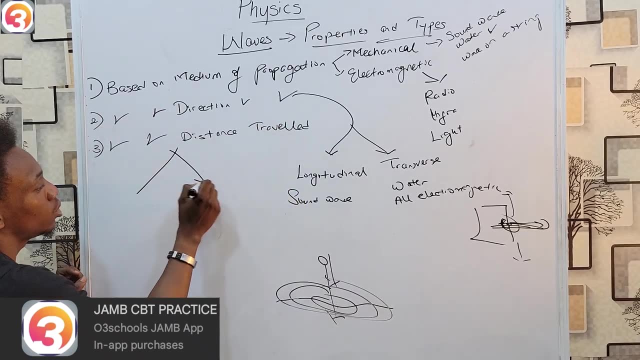 So that means everything that's electromagnetic falls under this group, But it's not the same that everything that is good can also fall under electromagnetic. But last but not least, this distance traveled, They have stationary or, before some phrases, standing waves. I also have progressive weave. 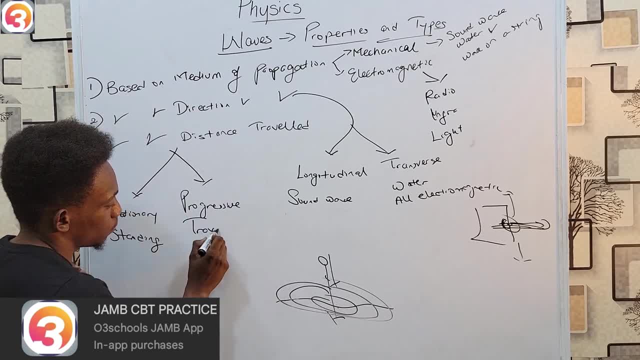 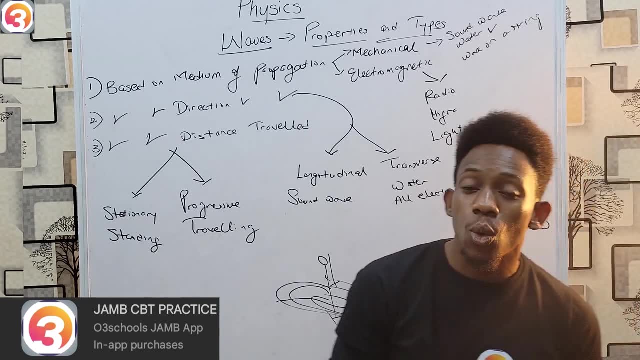 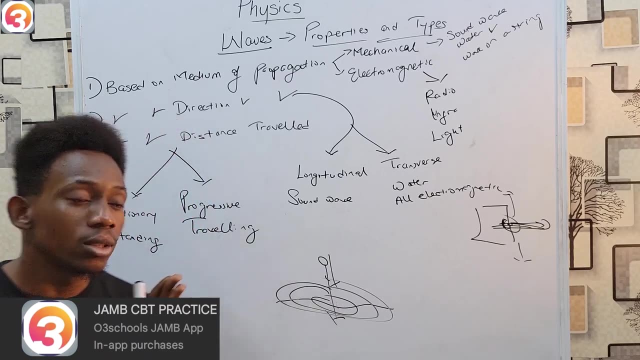 Or traveling weave. Now this is not all. realizes are related in your analysis, Children. Now what is the difference? A stationary wave simply doesn't really move anywhere. A wave on a string is a good example. Once it gets to the end of the string, your wave terminates. It can't pass there. It has a boundary. 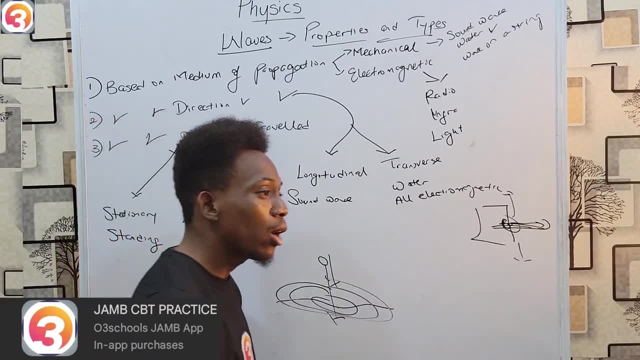 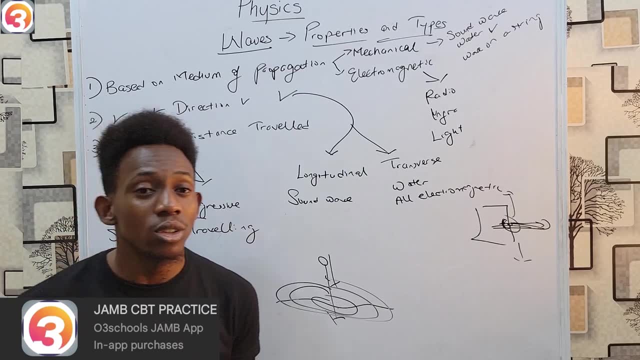 A progressive wave, on the other hand, doesn't really have a boundary. It can only stop when the energy power in it has been exhausted. Therefore, if I was to shout, the wave doesn't terminate once it comes out of my mouth, No. 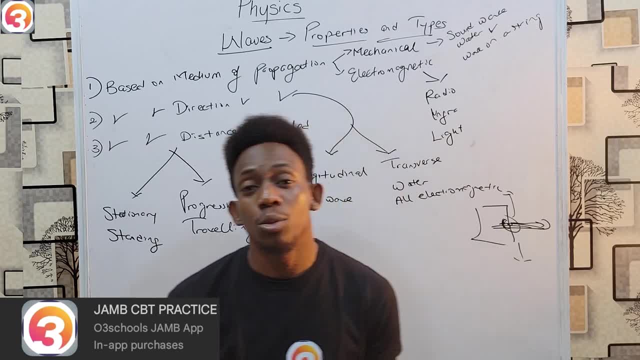 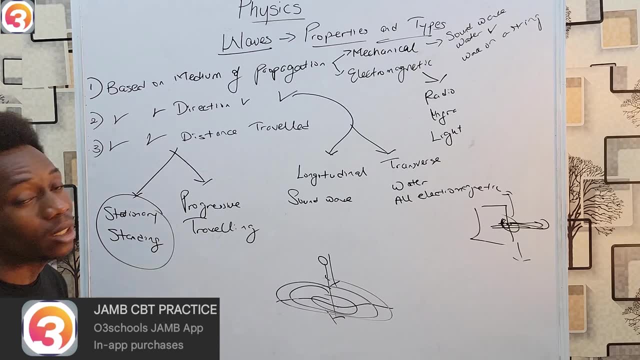 It keeps on going, but the wave decays until it gets to the place where you can no longer hear that sound. That's the difference. Stationary waves have a boundary, They cannot exit, They cannot pass there, like your wave on a string rather. 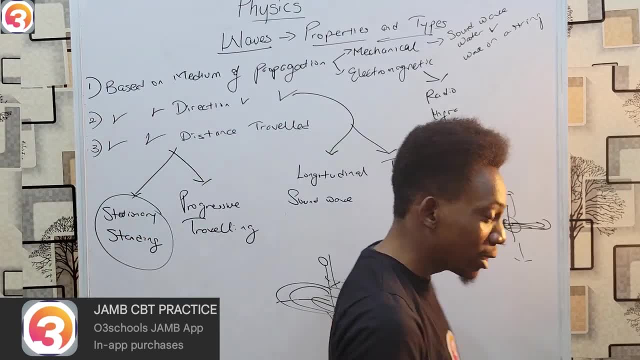 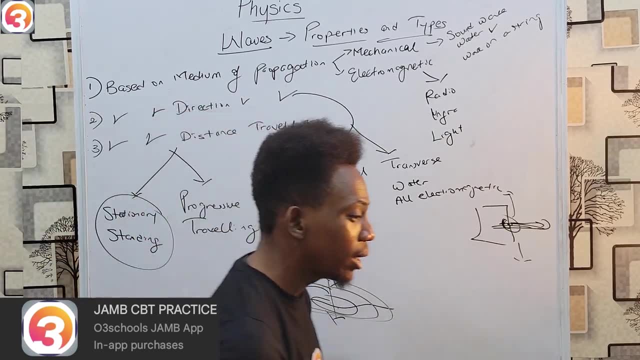 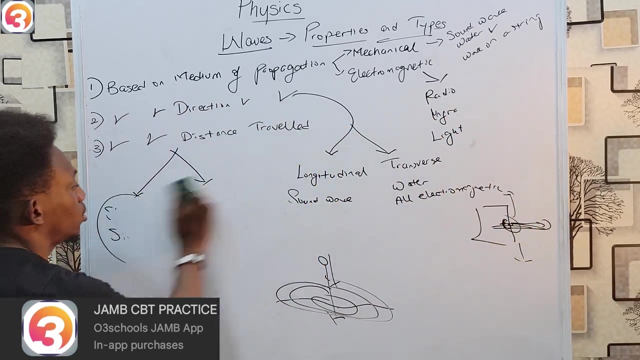 My progressive waves can actually travel. Now, those are types of waves based on the following criteria: The next two which I did look at are the pro-paxes of waves. We've talked about types. What about pro-paxes? How do I know that any material I'm looking at is actually a wave? 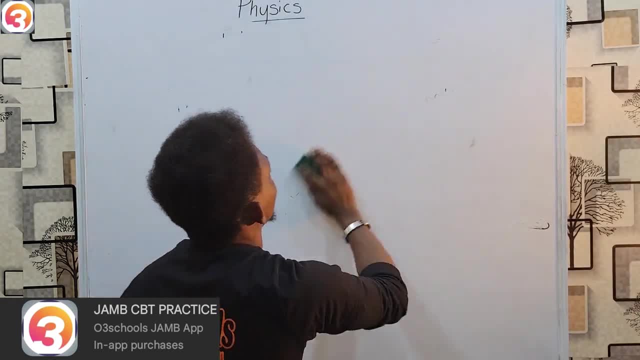 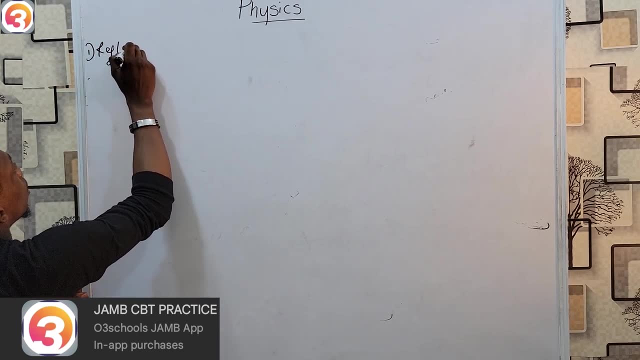 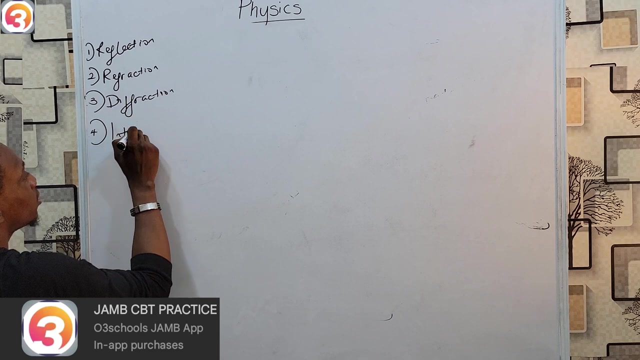 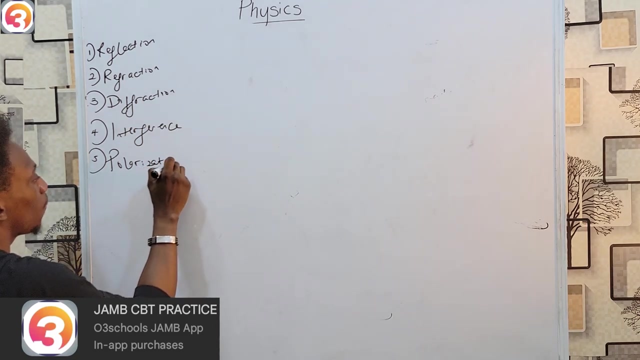 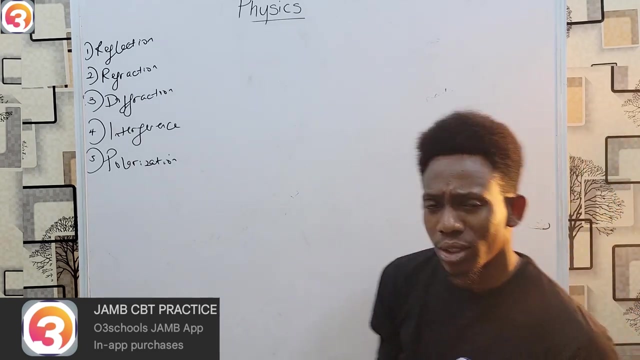 Now we have about five pro-paxes of waves that we look at. Five pro-paxes: Number one is reflection, Number two is refraction, Number three is diffraction, Number four is interference, While number five is polarization. So to identify that something is a wave, it must possess at least four of these pro-paxes. 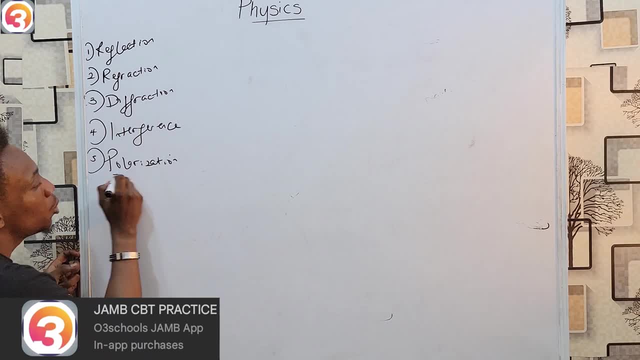 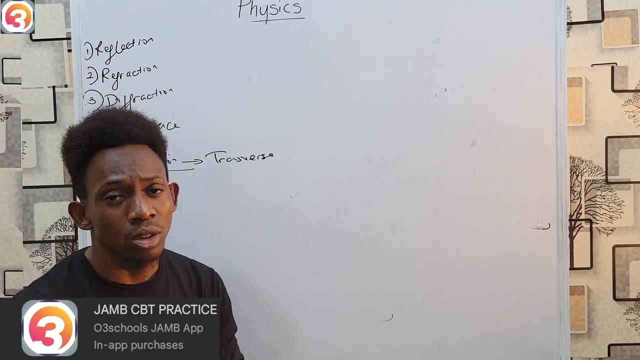 And why do I say four and not five? That's because this last one here, polarization- only works for transverse waves. That's the difference. Every single wave can undergo this four, but only transverse waves can undergo polarization. What is polarization? 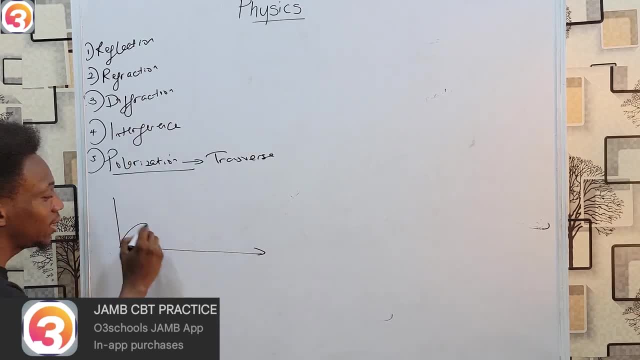 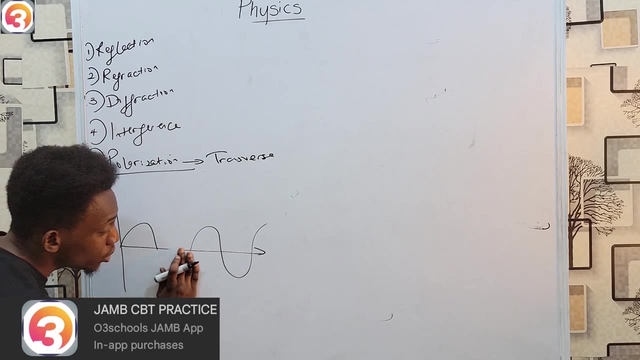 It's simply: if you have a normal wave, it moves like this. Polarization is a process by which we make sure that this wave's vibration exists in only one plane. Therefore, it's like we are clearing the bottom and the wave can only exist above. 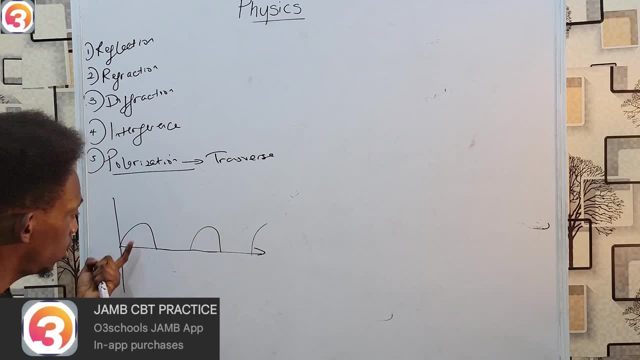 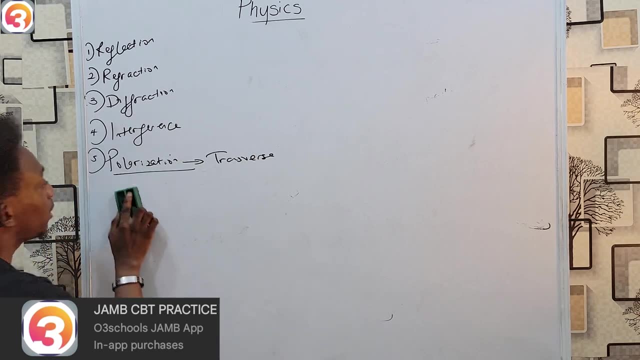 This is polarization, And it can only work for four. It can only work for the transverse waves, That's that. So now let's go and start from the top. I'll talk about polarization. We have reflection. What is reflection? 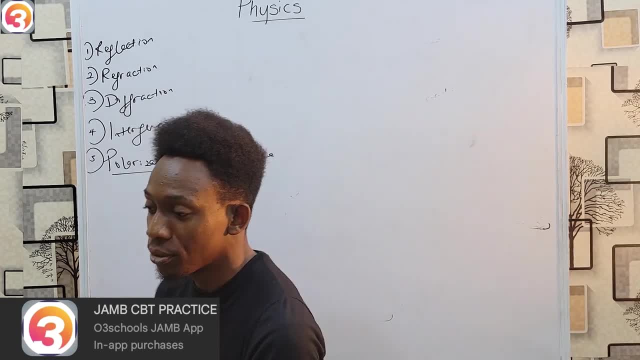 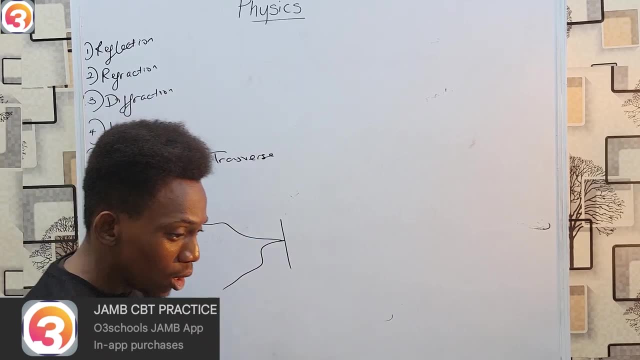 Reflection is the bouncing back of the wave when it hits an obstacle. So the wave goes forward, hits an obstacle it cannot pass through and bounces back. We'll treat expansion, or rather we'll treat reflection of waves, in a different video. 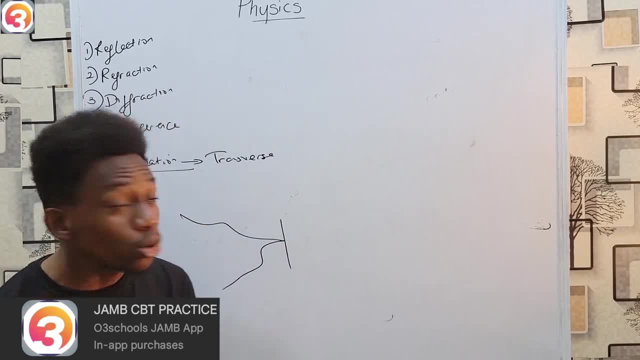 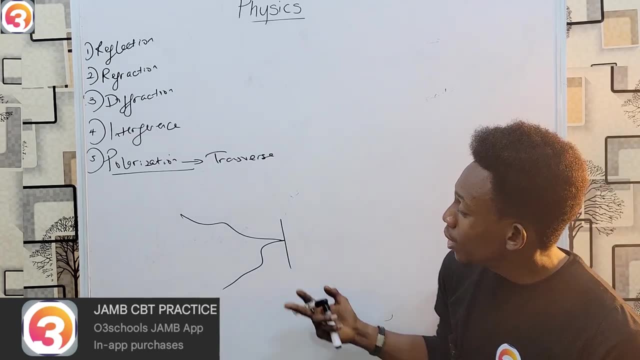 In a different video which you can check on the channel. you'll see the video there. we'll treat reflection as a topic on its own, So there's no need for too much explanation over here. Just know that it's the bouncing back of waves, eg with a mirror. 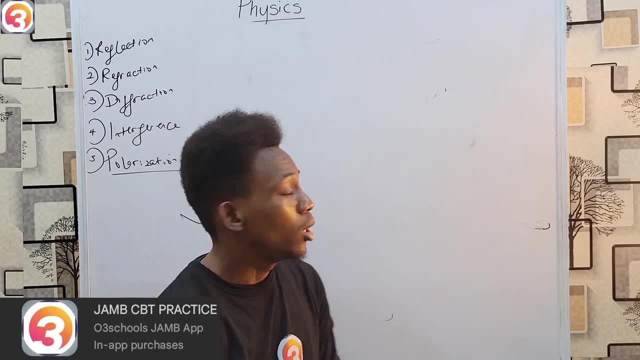 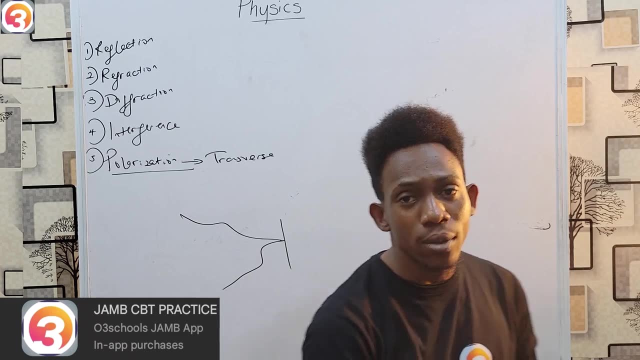 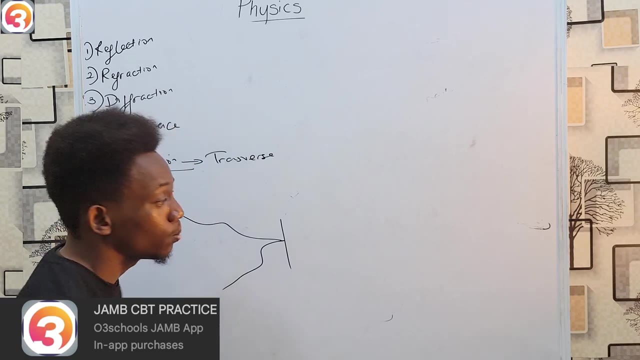 A light hits the mirror and bounces back. That's reflection. Then there's refraction. Refraction is simply the bending of the wave as it crosses the boundary between two media of different densities. Reflection was for when it cannot pass through. What if it can pass through? 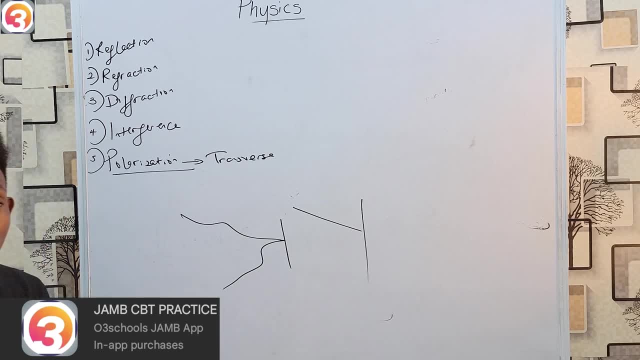 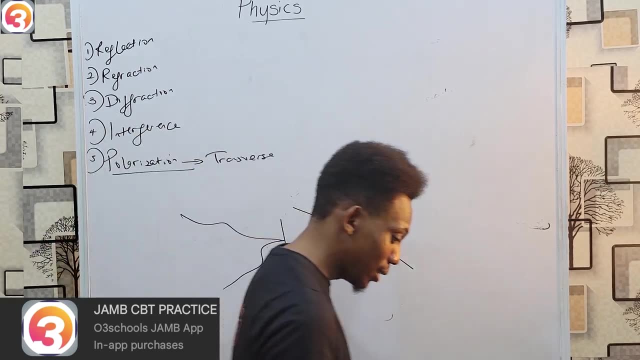 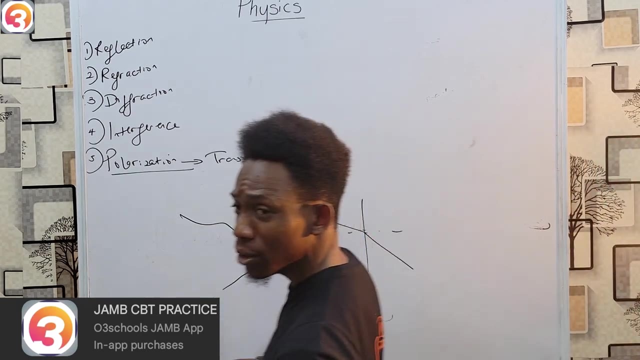 When it passes through, instead of passing through and coming out of the way it entered, there's usually a change in the wave, A change in the velocity, wavelength and the direction. This is what we refer to as refraction, And, just like reflection, we also treated refraction as a topic on its own in a separate video. 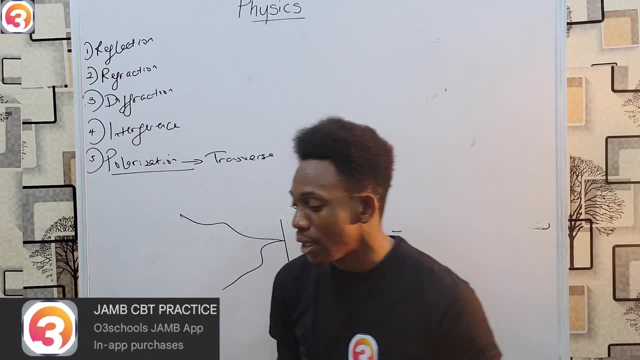 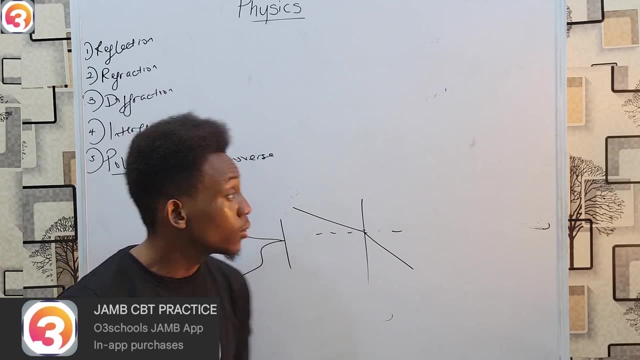 So I don't have to go too far into it. We did refractive index and a lot of other things. So please again check the channel and you can see the video for refraction. Now diffraction: We have not even treated diffraction in a separate video. 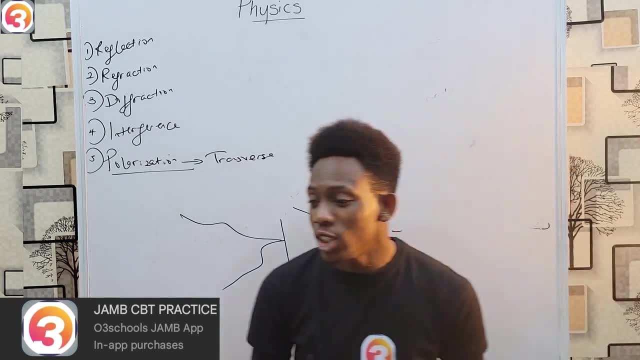 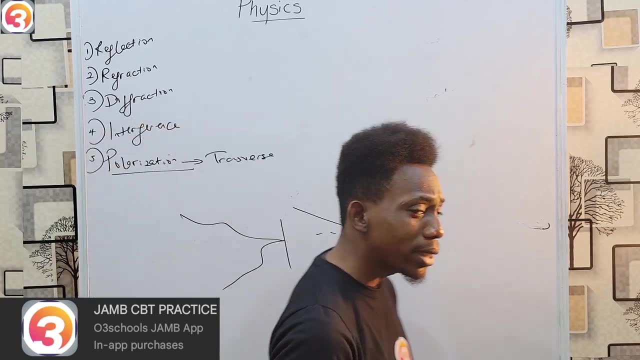 What is diffraction? Diffraction is the spreading of the wave as it passes a tiny boundary. Say, for example, if you ever play music and you open your door just a little bit, the sound you hear outside doesn't seem commiserate. 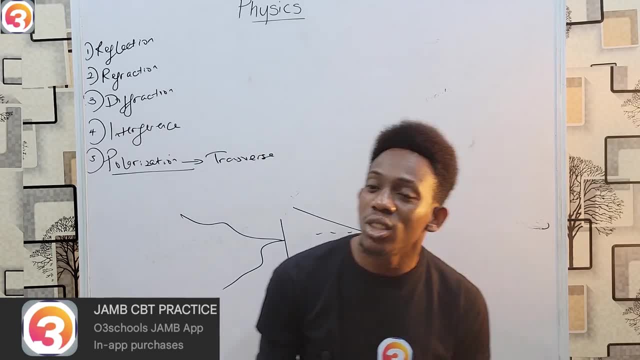 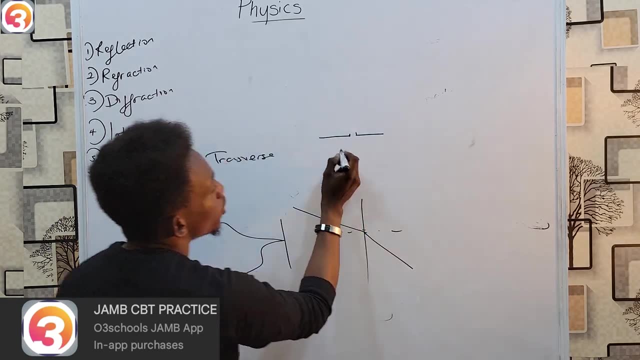 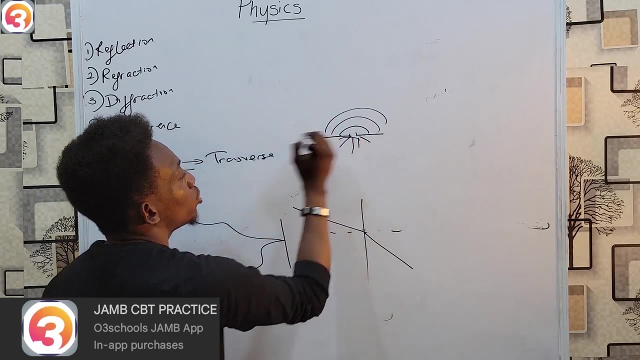 With the size to which you opened your door, You can expect to hear just a little sound. But the thing is that as you have a small boundary and your wave is passing through, when it comes out it begins to actually spread out as it comes through this hole. 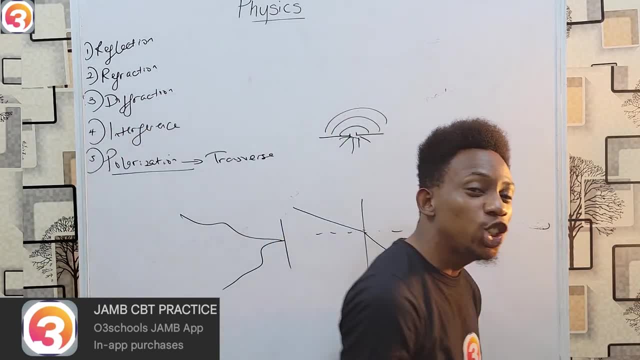 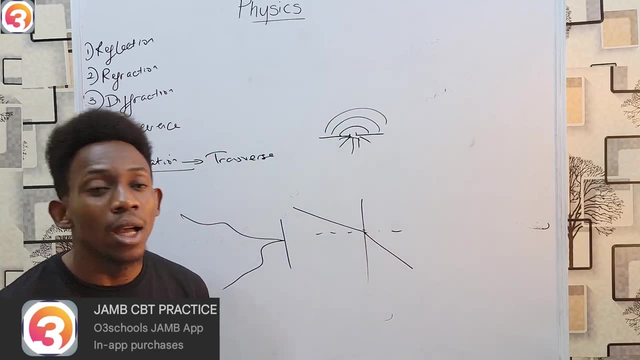 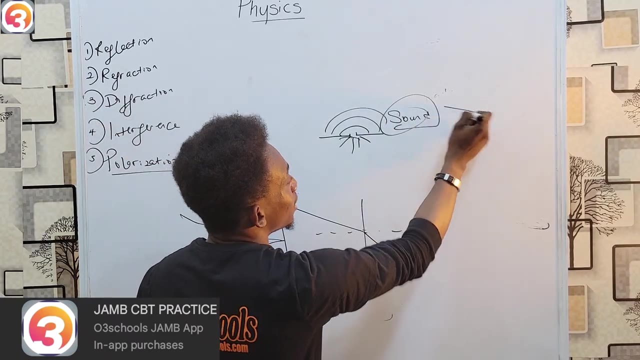 And the bigger the wavelength, the more the diffraction effects. So a wave with a big wavelength can diffract more than a wave with a smaller wavelength, And for that reason sound which has a big wavelength experiences a greater diffraction than light, which has a much smaller wavelength. 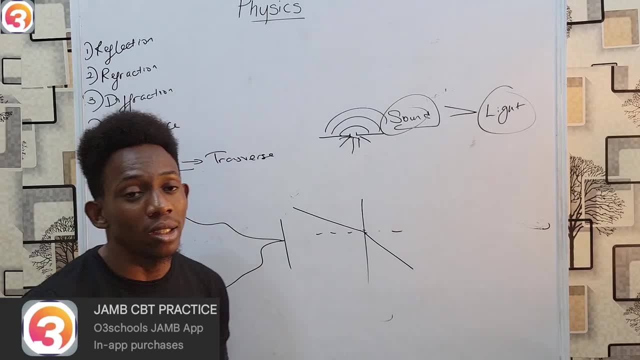 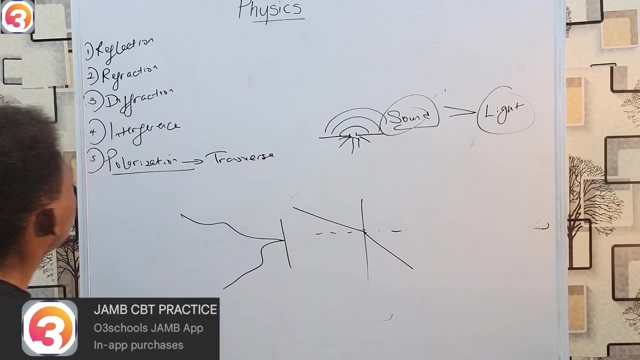 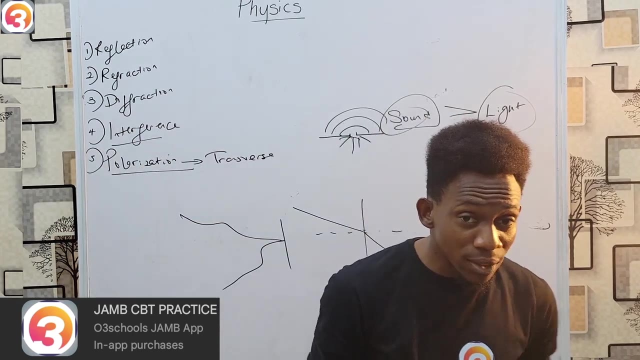 The wavelength of sound is greater than the diffraction of light, Because the wavelength of sound is greater than the wavelength of light. And then we also have interference. What is interference? Interference is in the particle sense. we try to observe interference. 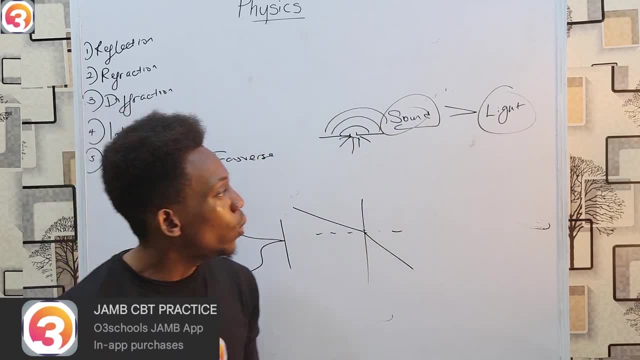 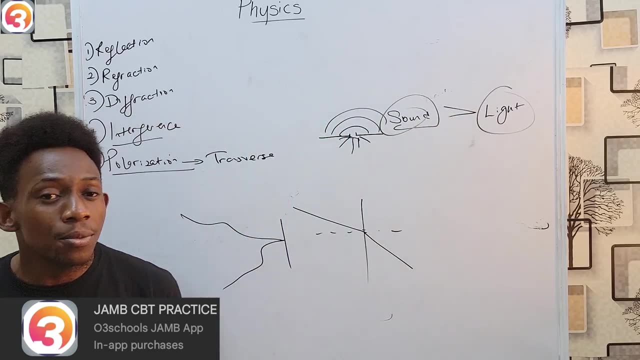 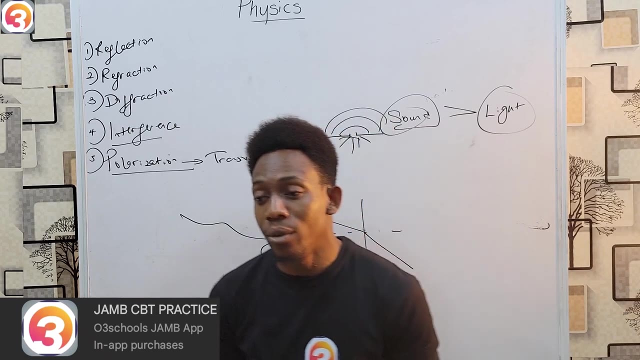 Interference is like a collision between two waves. When two waves meet each other, what happens? However, please note that for interference, the waves must have the same frequency and the same amplitude before they can interfere. So two similar waves of the same frequency and amplitude when they meet each other. 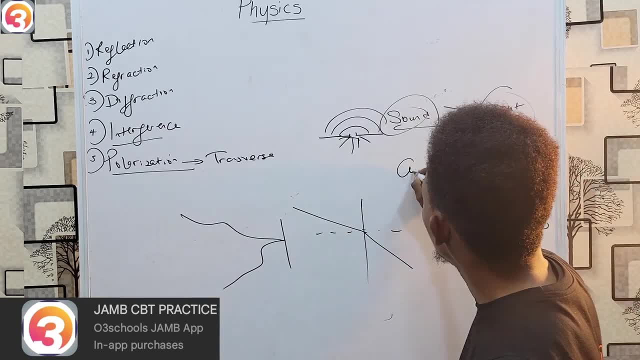 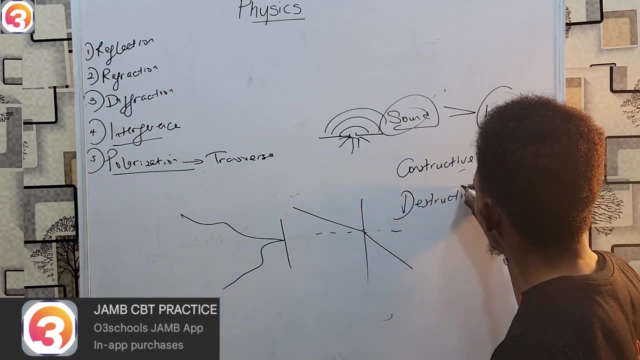 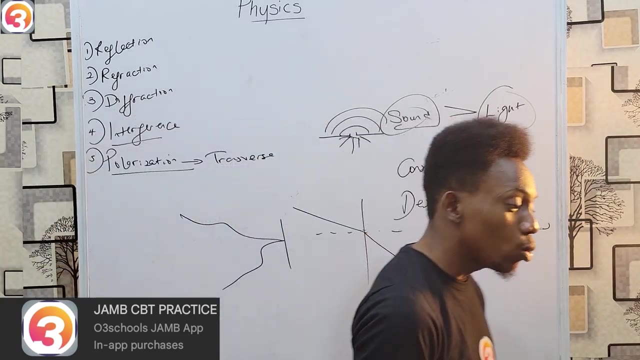 interference occurs, And we have constructive interference And we also have destructive interference. Now, obviously, non-destructive means we are destroying, we are breaking down. Indestructive interference is what happens when two waves meet each other and then they reduce. 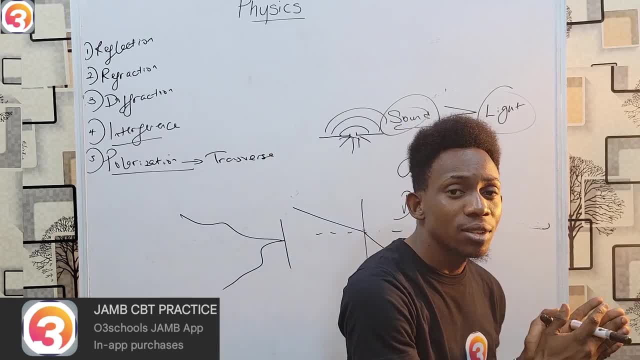 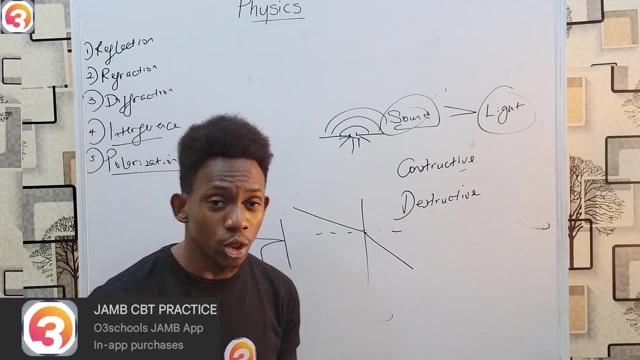 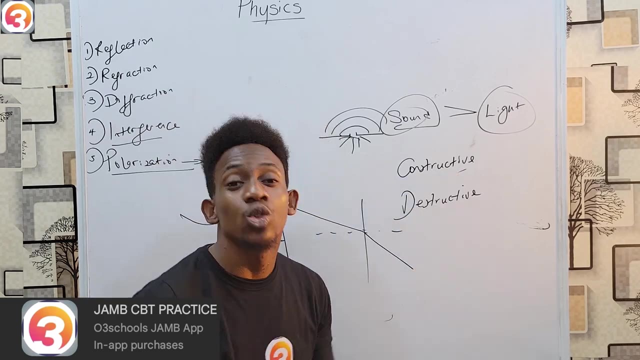 When constructive interference is when they meet each other and they increase. Now, however, what determines whether a wave should be constructive or destructive is the phase angle, Which we shall look at shortly. But just note that if two waves are perfectly in phase, then we get totally constructive interference. 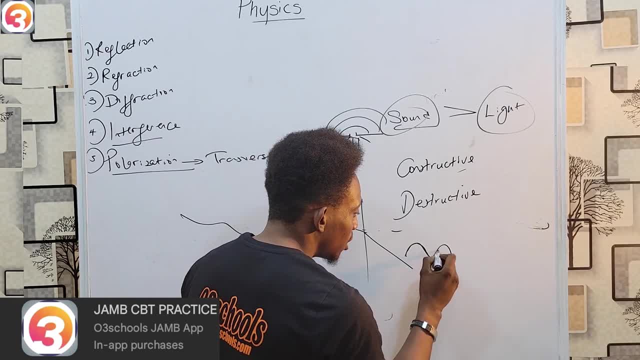 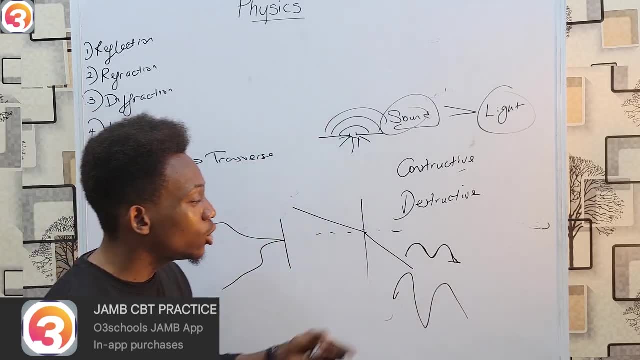 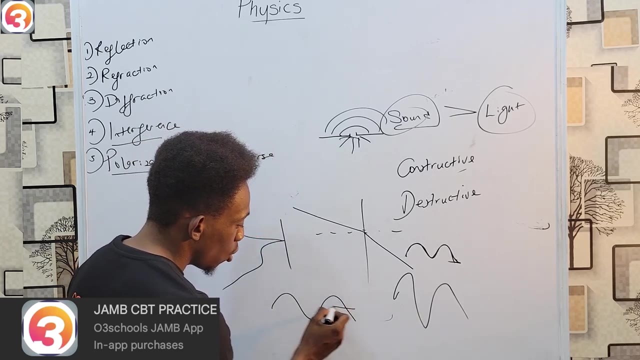 If this was one wave and the other wave was also moving perfectly in the same manner. when they meet, they will form a wave times two of the initial size. Why a destructive wave occurs when they are perfectly out of phase, That is as this one is going up. 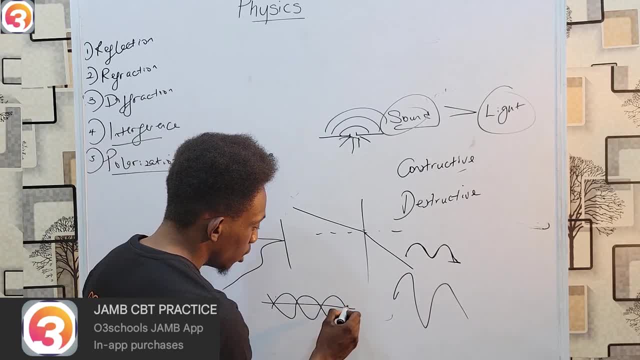 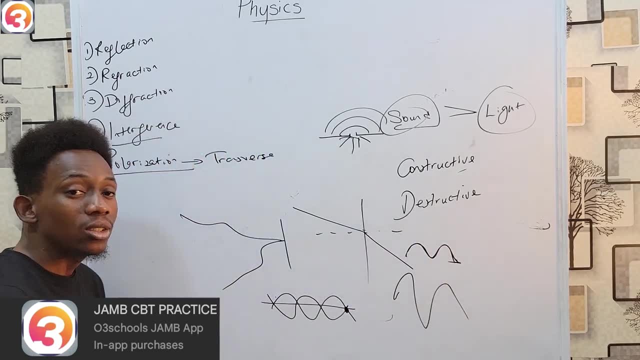 the other wave is going to be coming down. If they meet here, they are going to completely cancel out, And in that case we are going to get a totally destructive interference, While on the other hand, if they are partially out of phase. 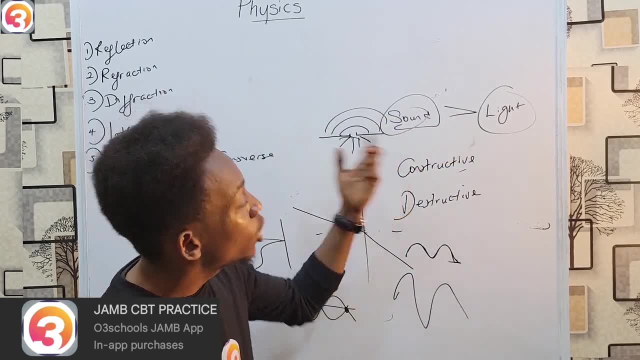 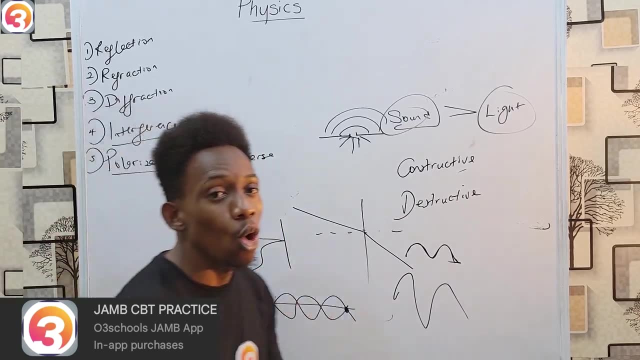 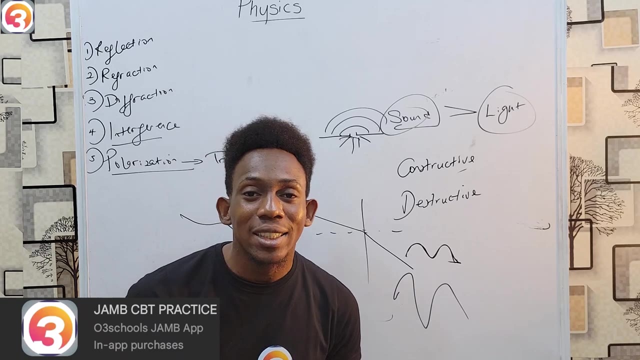 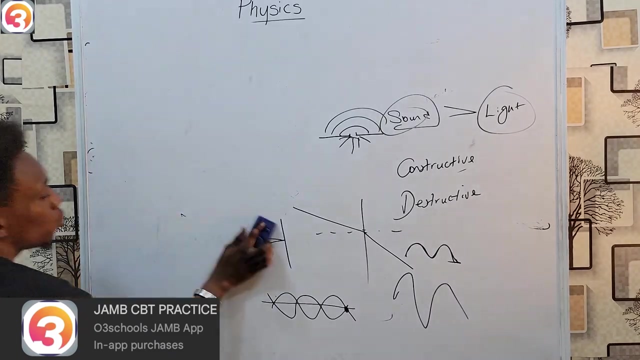 then they end up going somewhere which is partially constructive and also partially destructive. So those are the properties of waves. However, knowing the properties now, when we want to analyze waves, what are the different things we must know when talking about waves? There are several concepts that one must know when thinking or talking about waves. 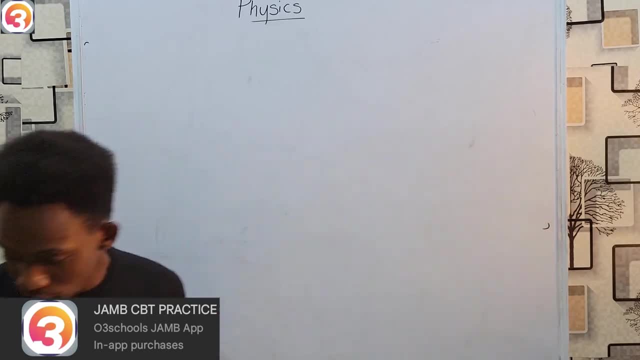 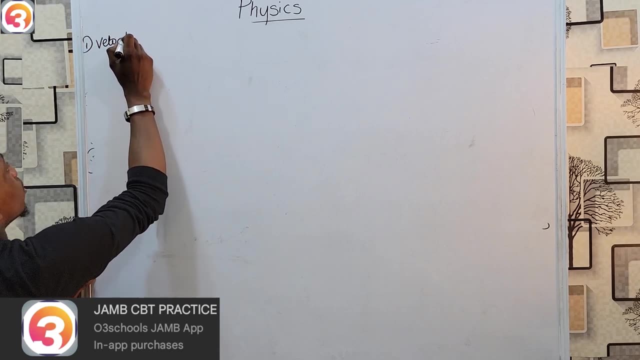 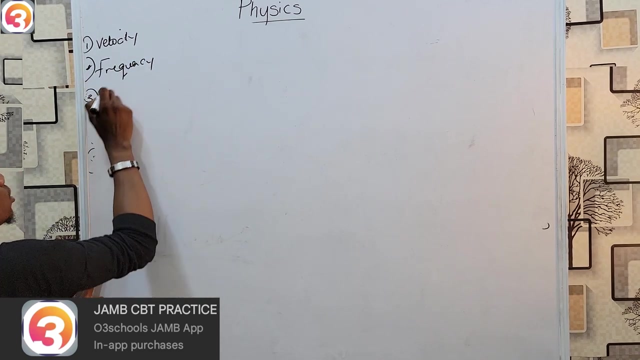 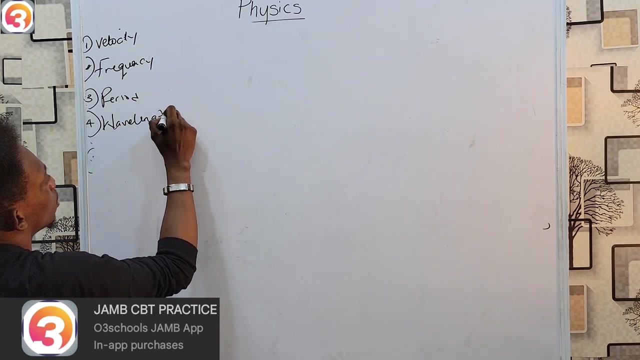 For example, we must know what is wave speed. We must know what is wave speed. There is speed or velocity of the wave, There is frequency, There is period, There is wavelength, There is amplitude, There is phase. We must know the success. 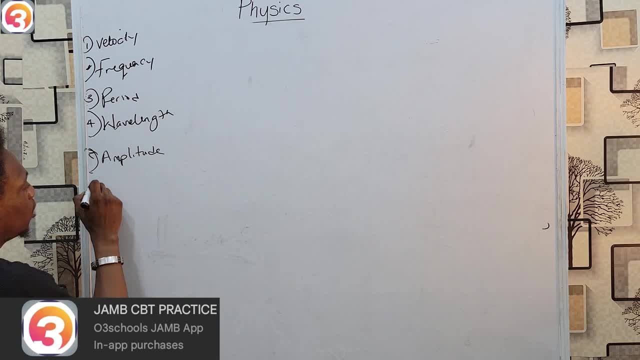 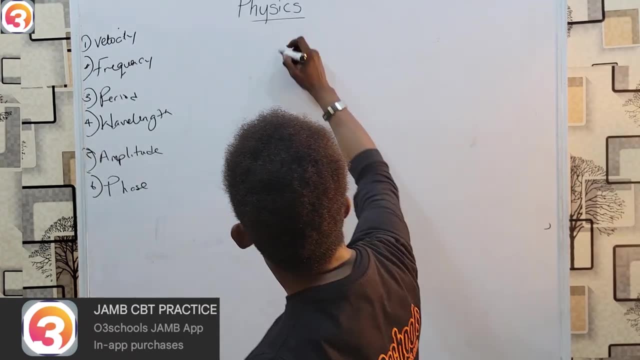 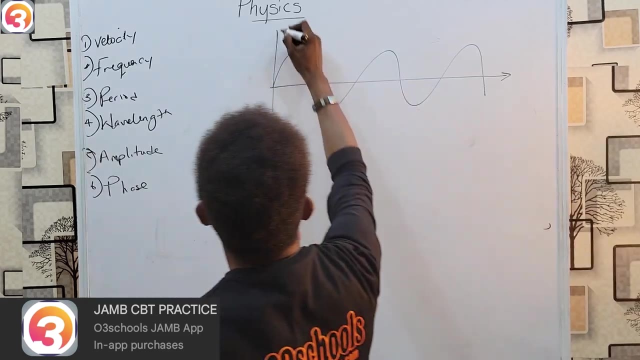 Let's start off by drawing the simplest representation of a wave. If this is a wave, then we must know what is wave speed. We must know what is wave speed. We must know what is wave speed. This is your y-axis, This is both the x and time axis. 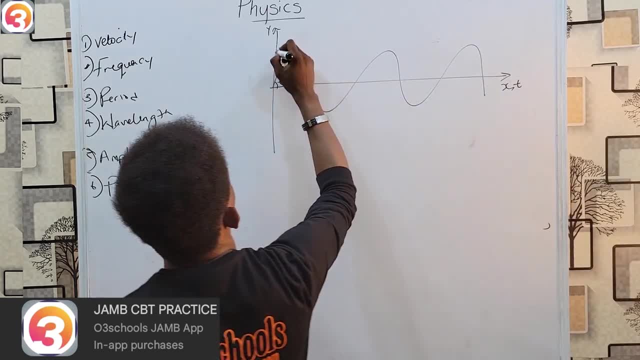 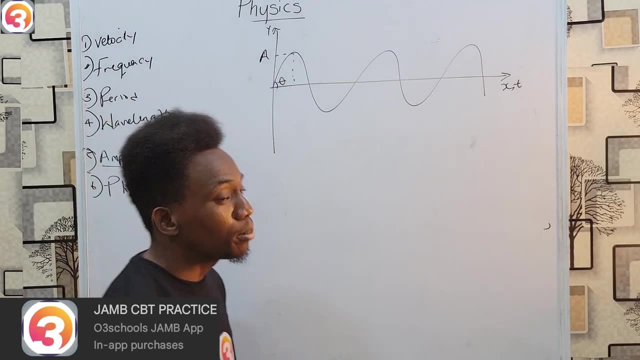 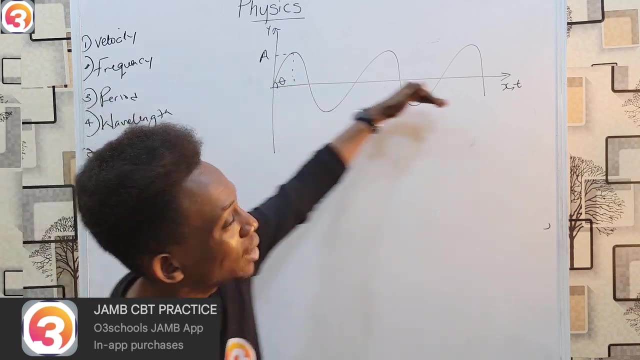 There is an angle here: theta, Then this maximum distance. So let's start off with amplitude. What is amplitude? Amplitude is the maximum displacement of the wave from the equilibrium position. This straight line is the equilibrium position, So the highest point it can go is what we refer to as amplitude. 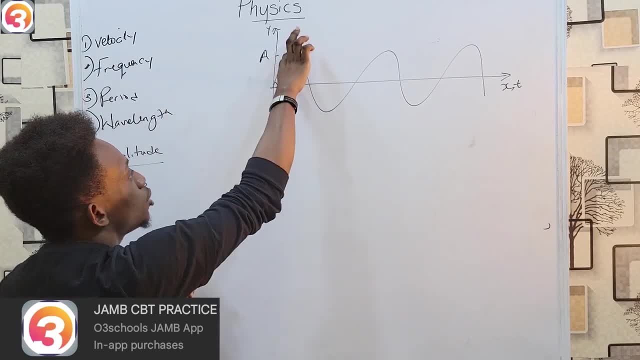 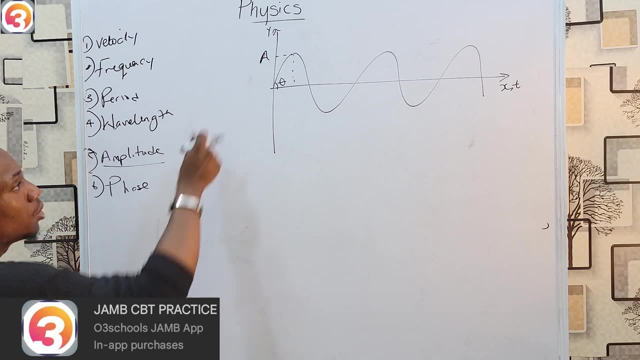 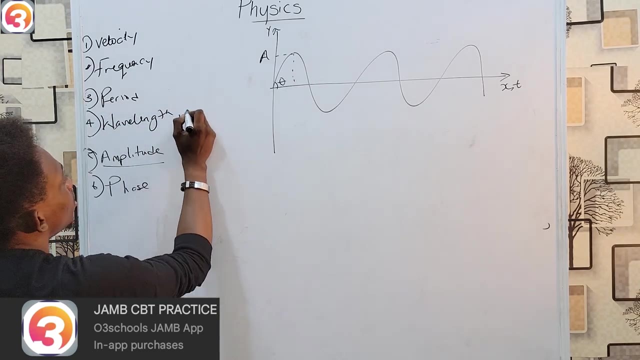 The maximum displacement, And you should note that this displacement equals this displacement equals this displacement. So that is amplitude of the wave Resulted by A. Then we also have wavelength. What is wavelength? This guy? And the symbol is lambda, Lambda. 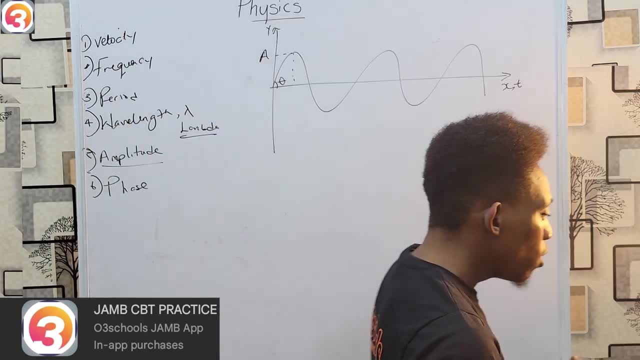 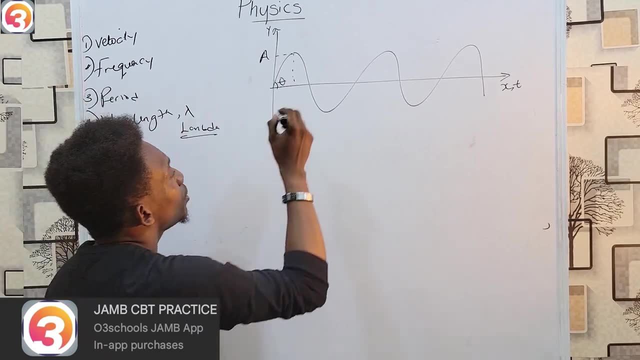 What is wavelength? Wavelength is the distance from one crest to the next successive crest. Crest Sounds like big grammar, I know, But basically we mean, if this is a crest, these top points are crests, The bottom points are called troughs. 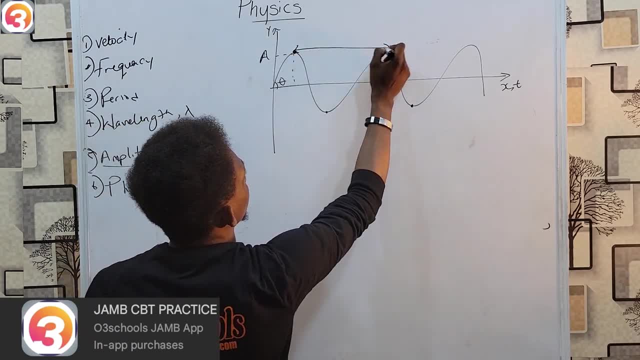 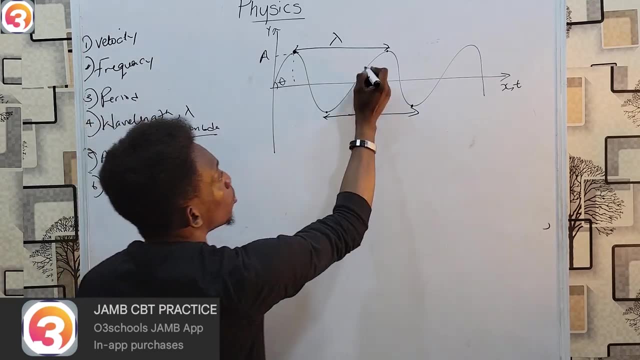 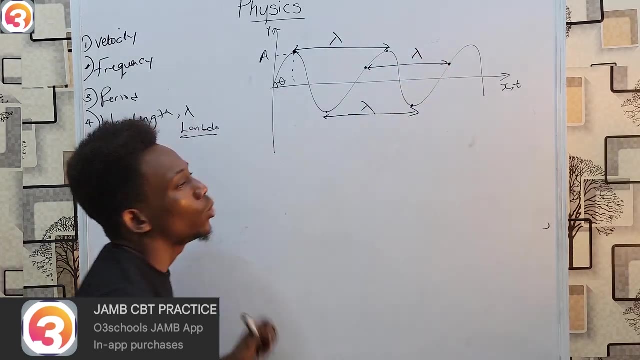 So the distance from this crest to this crest is one wavelength. Here to here, also one wavelength. In fact, I can also pick a point here, From here to the corresponding point, exactly like that is also going to be a wavelength, So that's wavelength. 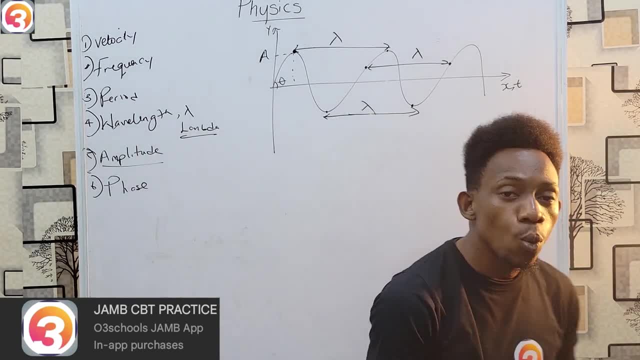 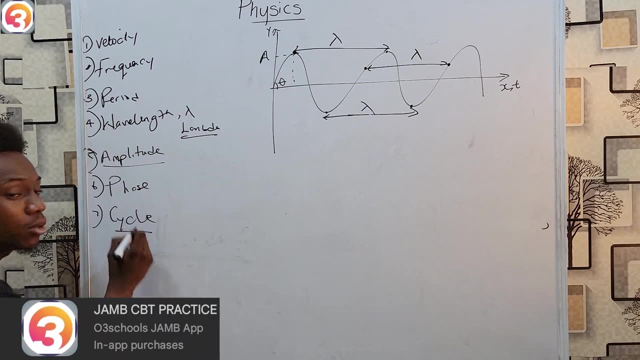 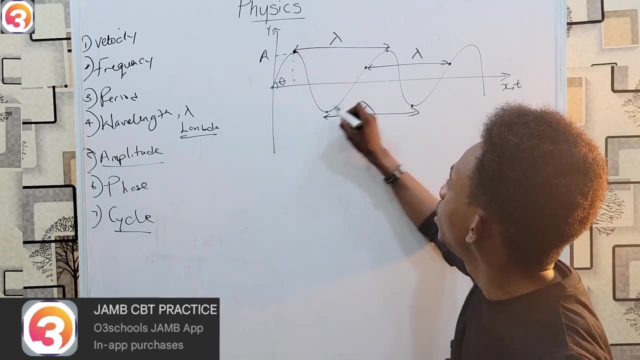 What about period? Period is the time taken to complete one cycle, And I think we should also explore the cycle. A cycle simply refers to one complete revolution, one complete movement of the wave. So from here up down to start going up again is a cycle. 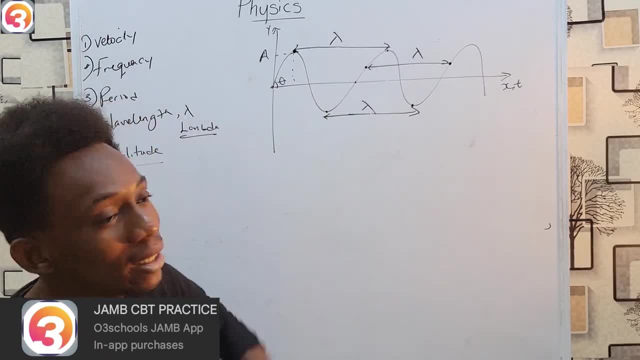 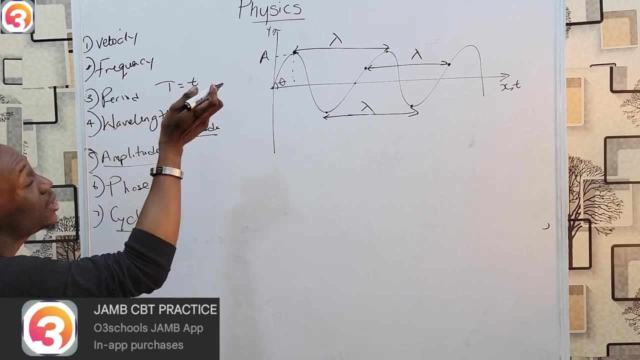 So a period is the time taken to complete one cycle, And it can be similar Period. big T equals to the time taken to complete as many cycles as you want by the number of cycles completed. So time per cycle, That's period. 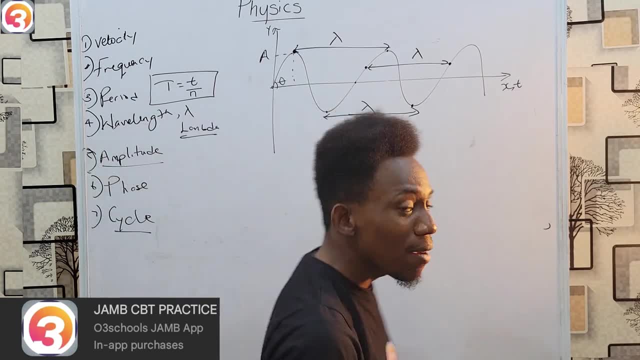 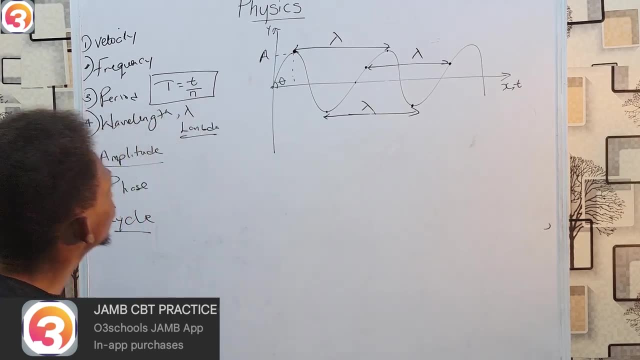 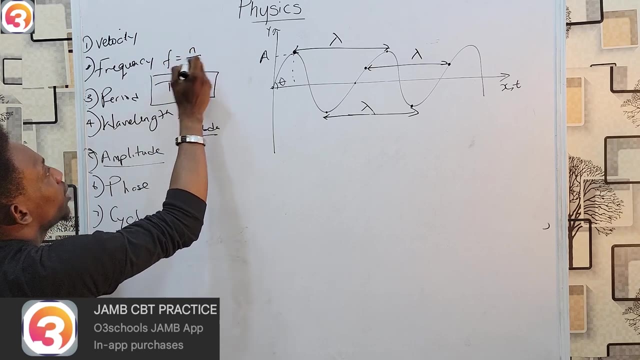 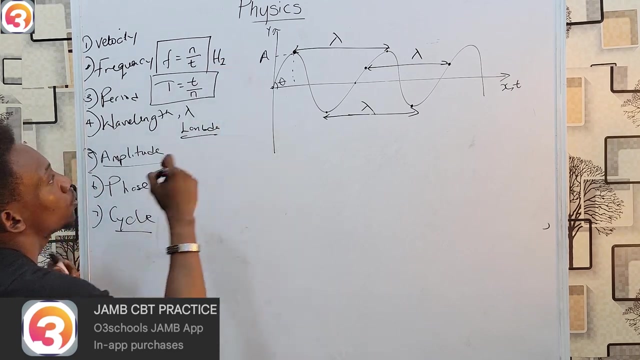 And the unit is seconds. However, frequency is now the number of cycles completed per second. Period was time per cycle. Frequency F is cycle per time And the unit of frequency is heads. HZ is the short form. It should not mean per second, but it is preferred to call heads after frank heads. 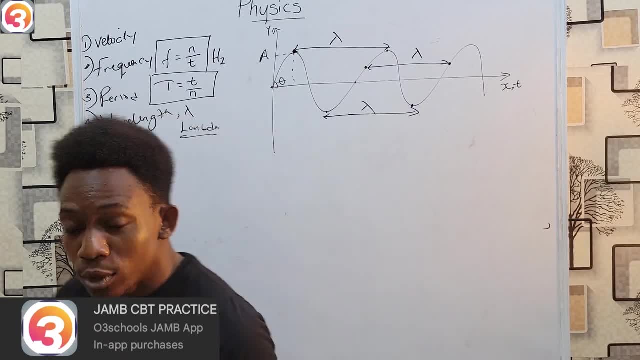 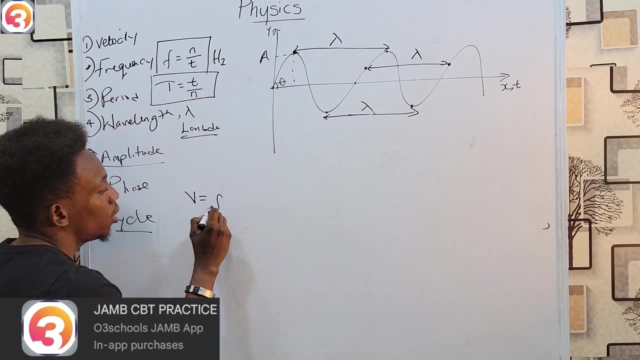 Then we also have velocity of the wave. Velocity of the wave simply measures how fast, obviously, the wave is moving And the form of velocity of the wave. V equals to F lambda. That's the form of velocity of the wave. 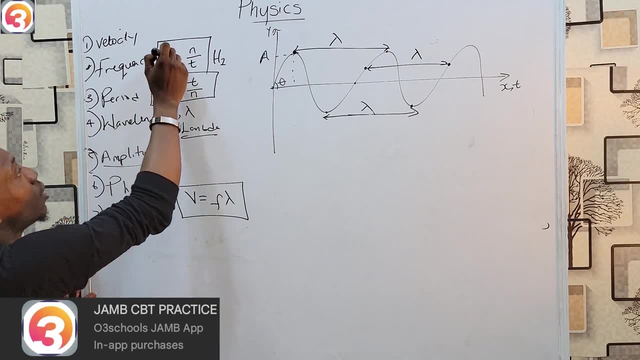 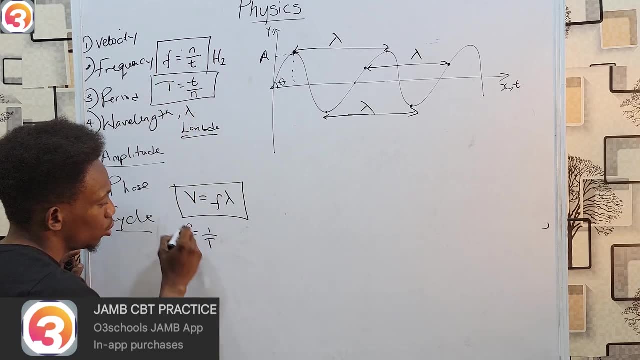 Then the one other thing you should notice. if you look here: F and T, they are almost the same right, It's just that they are reversed. Therefore, you should know that F equals to 1 over T, And that is the next thing we should know for a wave. 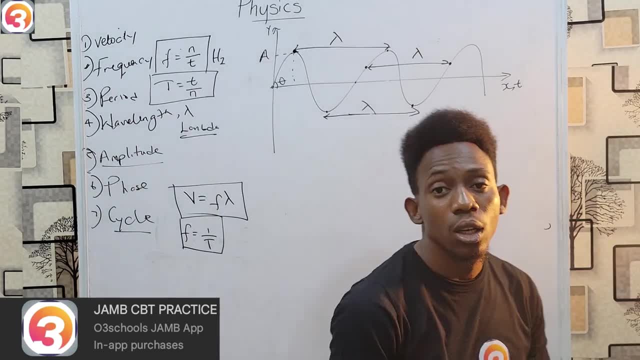 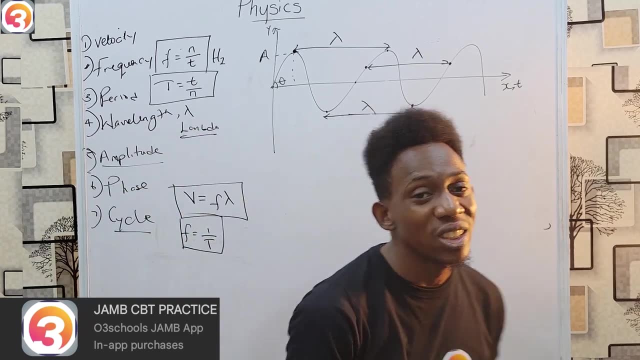 Well, last but not least, we also have phase there. What is phase Now? two waves are said to be in phase, when they reach their peak and their minimum destinations at the same time. That means, as one is going up, the other one is going up. 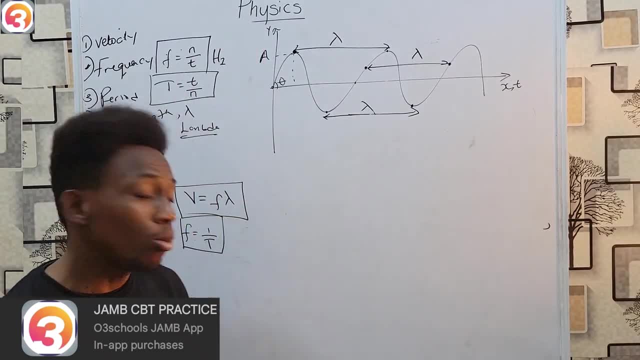 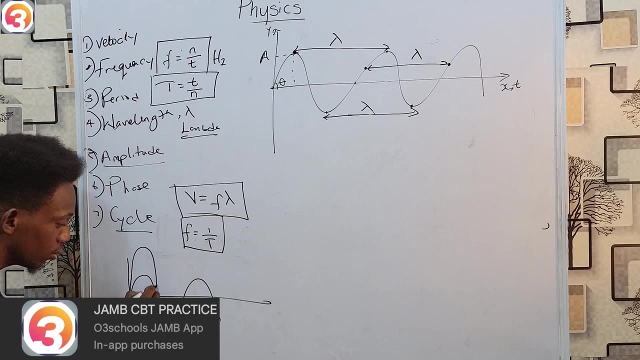 if there is a topmost point at the top at the same time and they also come down at the downward point at the same time, then they are in phase. Something like this: They might not have the same shape, but they are meeting at peak at the same time. 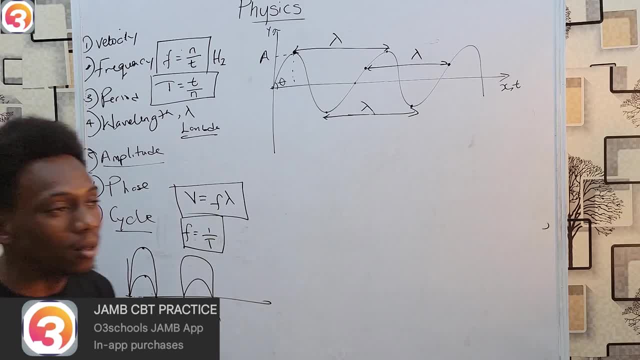 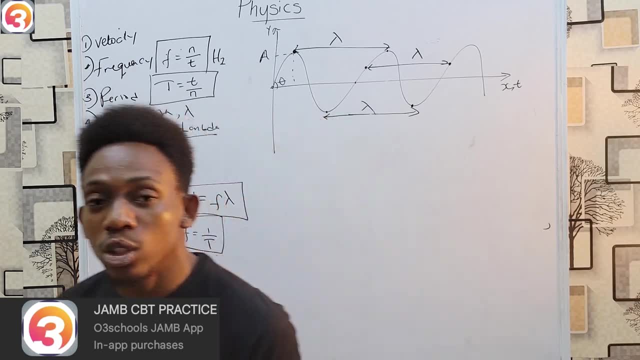 bottom at the same time, equilibrium at the same time, And that is what it means to be in phase. If it's not like that, then they are said to be out of phase. So these are the terms we shall use in analyzing a wave. 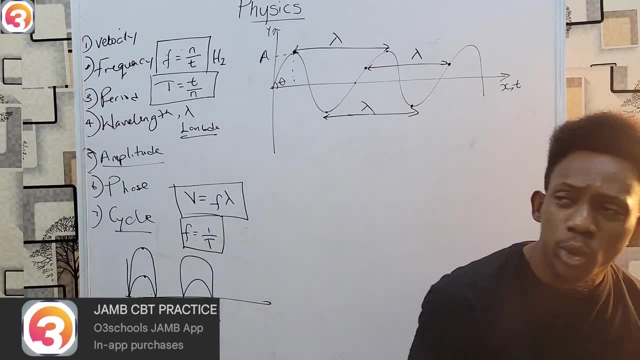 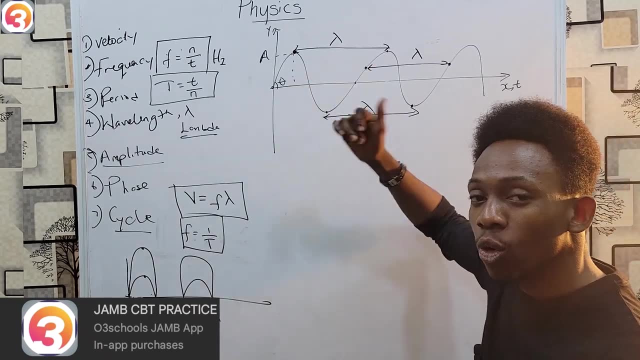 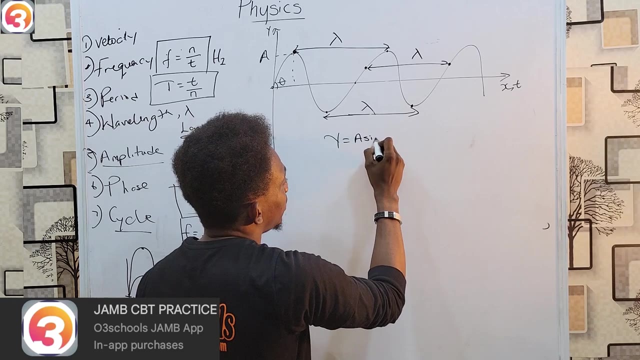 And now this is the simplest diagram for a wave. But to analyze this, if you remember, this looks like a sine graph. in mathematics This can be referred to as a sinusoidal waveform. And because this is a sinusoidal waveform, I must know that y equals to a sine theta. 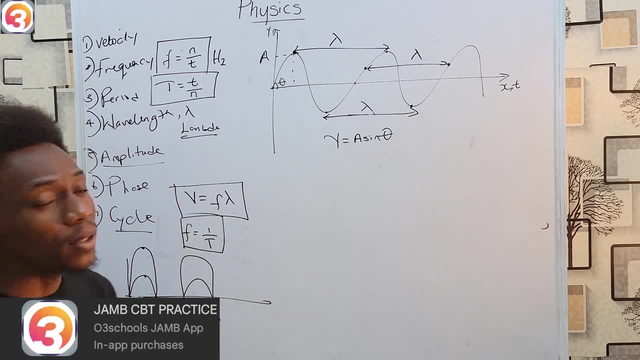 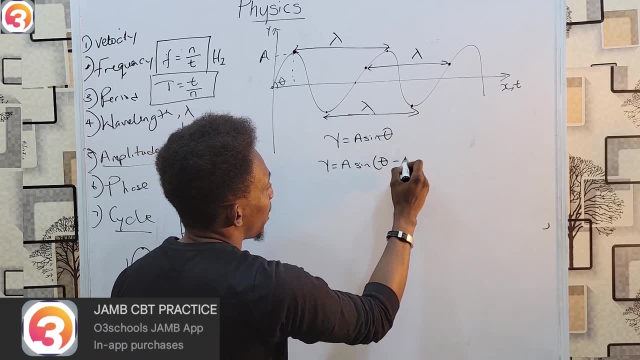 That is the first thing I know. However, what if this wave is a bit out of phase? Then I must introduce a phase angle, a sine theta minus phi. Now, please note, in some test books they use theta plus phi. 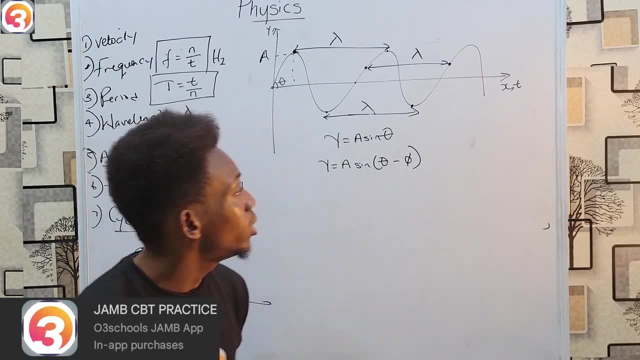 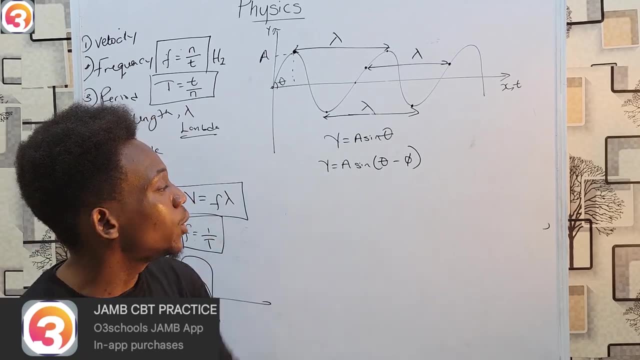 As far as I'm concerned, it doesn't really matter Plus minus. they are irrelevant for the type of solving we are currently doing. Like this is where it's important, but not here. So this is my basic formula for the wave. 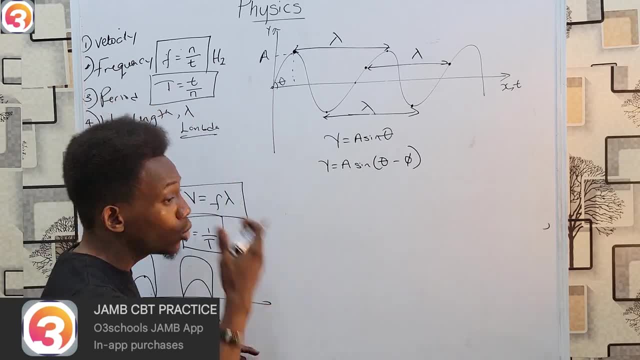 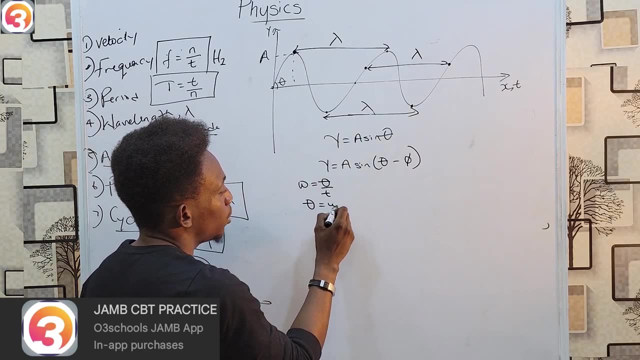 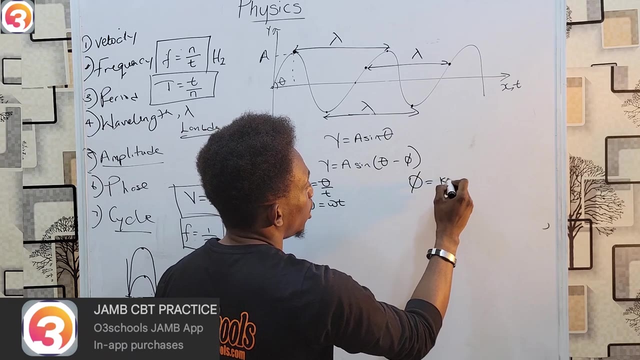 Then if I look at my theta, you should remember from your simple harmonic motion that angular velocity, omega equals to theta over time And therefore theta equals to omega t, While my phase angle phi equals kx. Therefore y equals to a sine. 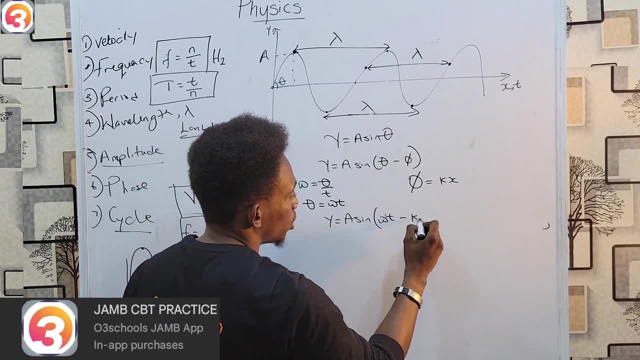 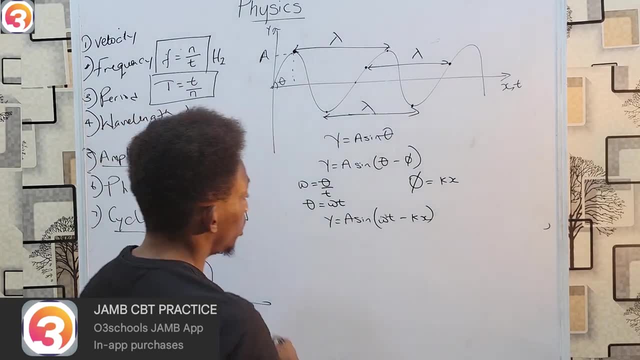 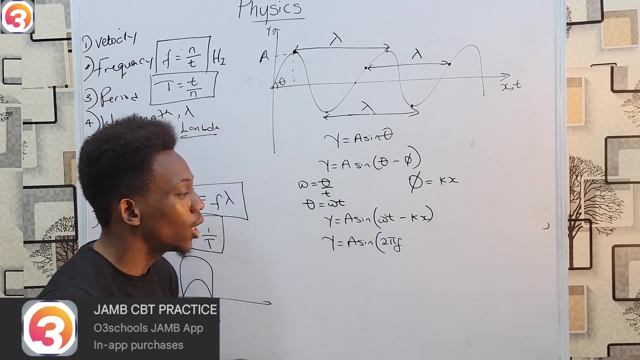 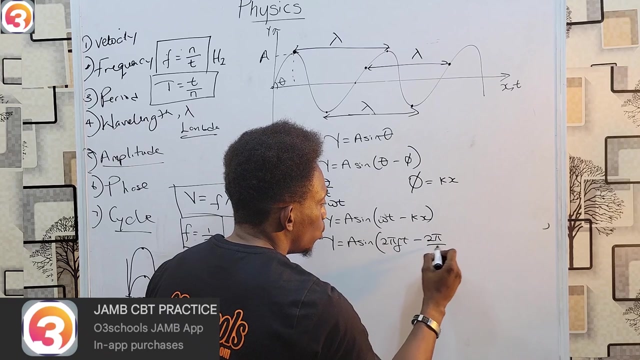 instead of theta, I shall be having omega t minus kx. Okay, Then again, recall from angular velocity in super harmonic motion, y equals to a sine two pi f, which is omega t, While your k constant here is actually given by two pi over lambda. 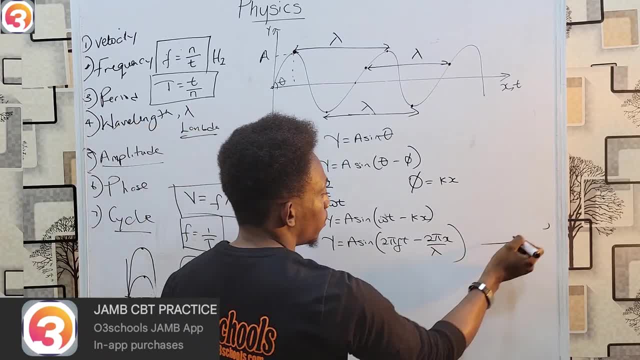 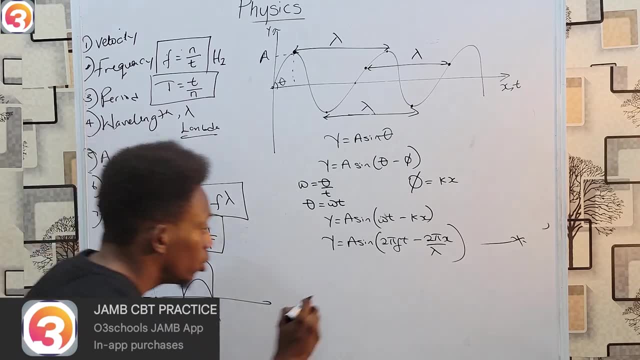 And here is x. So this is one basic formula for a wave, which you should note. But then, if you also recall f, as we have here is one over t, So y could also be equals to a sine. 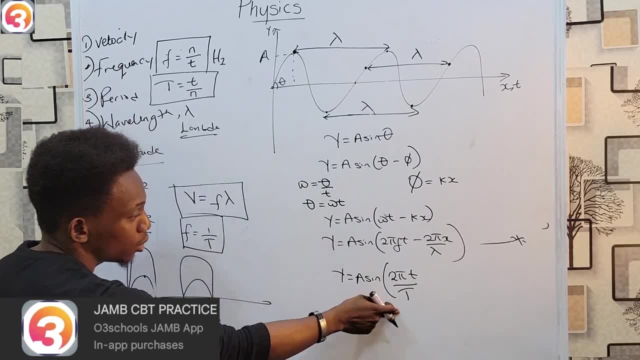 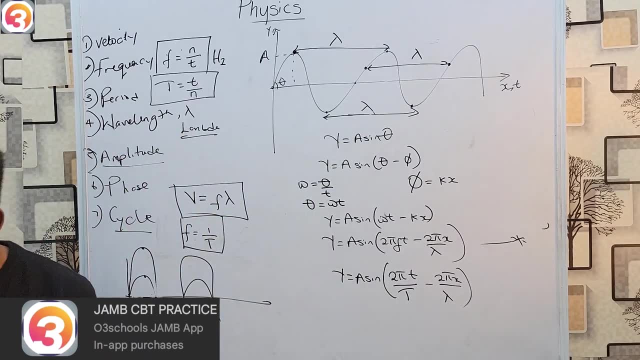 two pi t over t, omega over period minus two pi x over lambda- Yet another representation of a wave. But we don't have to stop there, Ask ourselves: is there any other way we could represent it? And yes, there is. 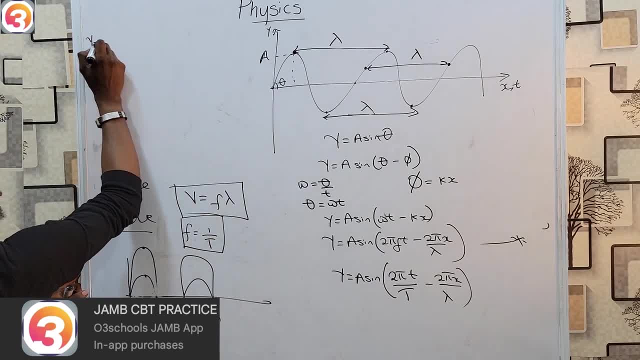 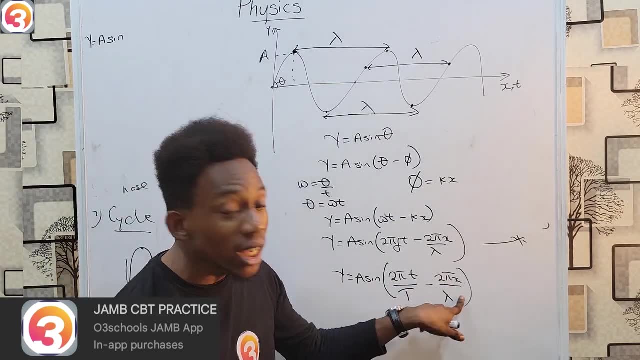 What we could then do is we could say y equals to a sine, and then we factorize out two pi over lambda. This make x stand alone. That would be a sine. two pi over lambda comes out into. 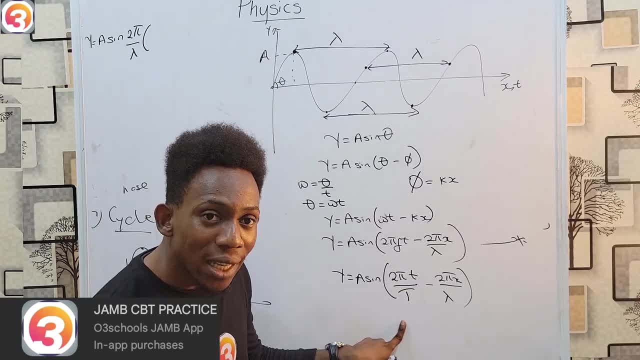 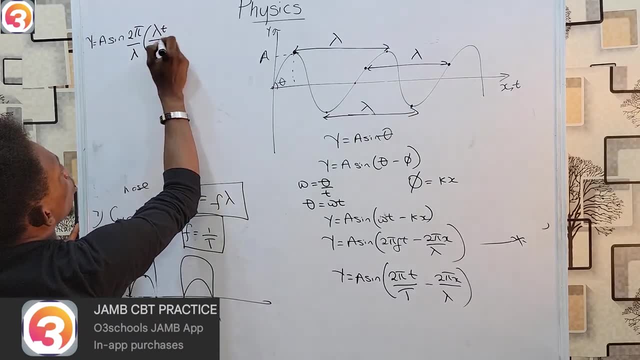 if two pi over lambda is the quantity of this space which does not have lambda down, then lambda has to appear up to cancel it out. So I'll now be having lambda c over period minus two pi over lambda leaves there. 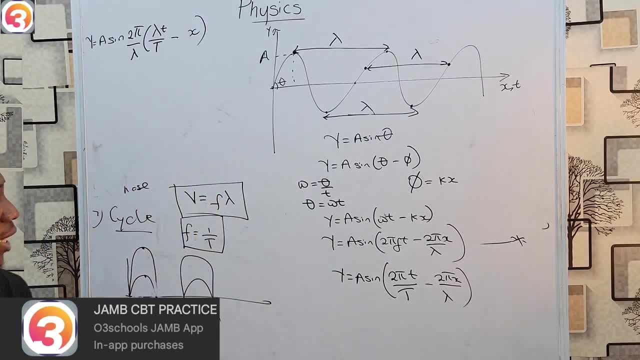 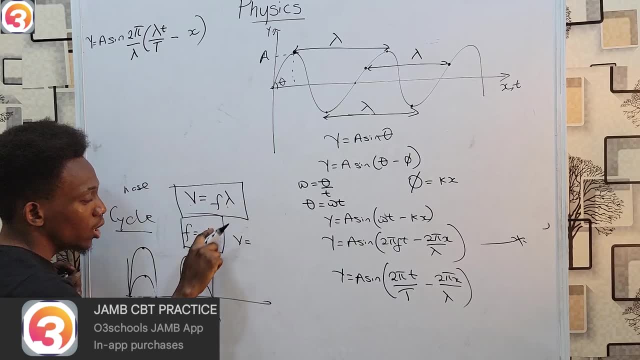 I have x. Now you may be asking: what can I do with this? Simply remember here: if v equals to f- lambda- then v must be equals to 20, f to one over t, that is lambda over t. In fact, where I see lambda over t, 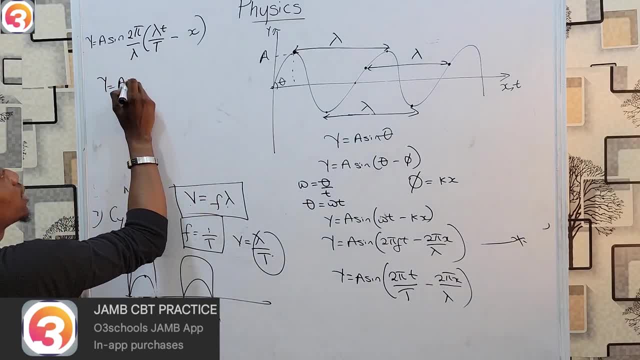 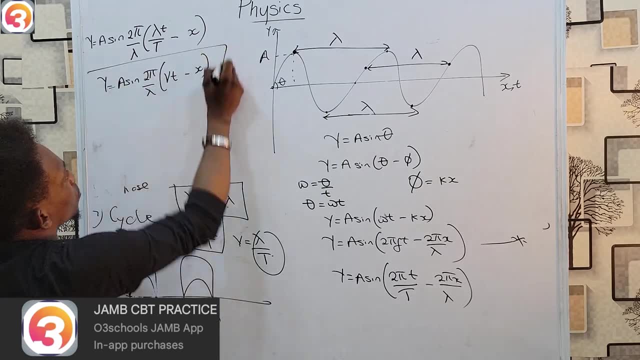 I can put v- So y equals to a sine, two pi over lambda- into vt minus x. I know some of us might be panicking right now looking at this and saying: how am I supposed to memorize all this? 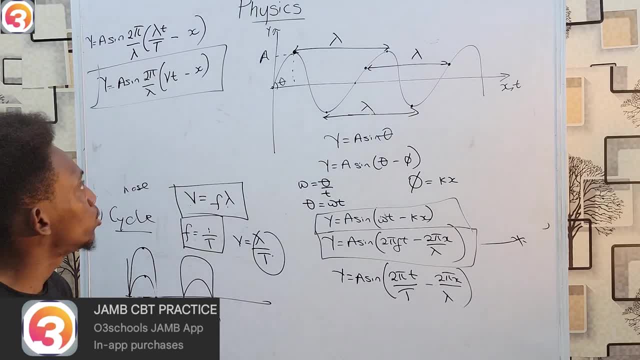 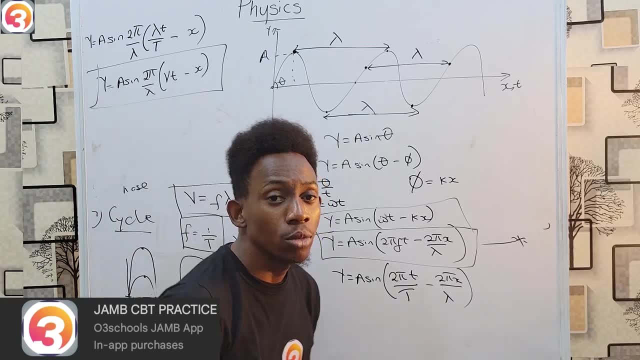 The good news is I don't have to prove this. We're writing jump. I'm not going to be proving a jump. You just have to know one, two and three. How do the questions come? They'll give you an expression. 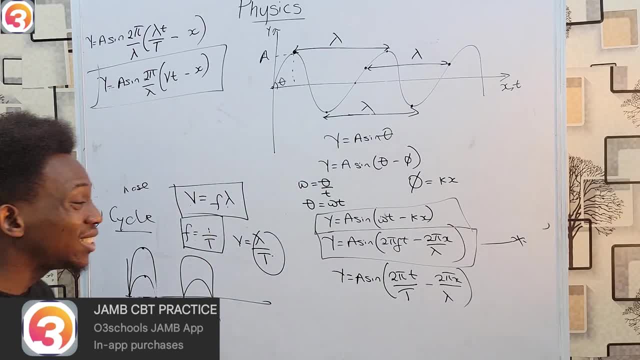 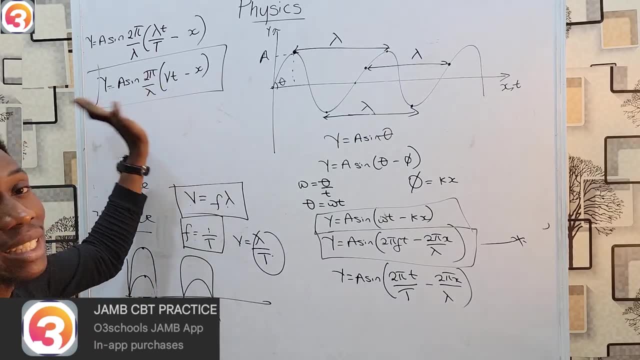 All you simply have to do is ask yourself: what does that expression resemble the most? Any expression. if I give you an expression that has two pi over lambda outside, that has any number outside between your sine and your brackets, you know you are dealing with this type. 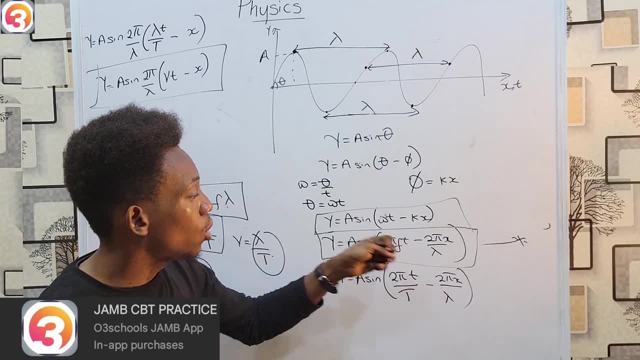 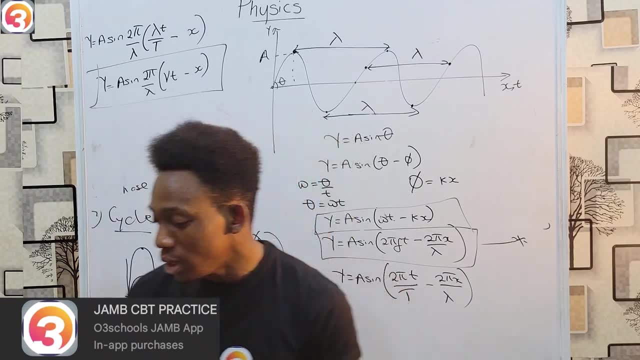 Why, if there's no number outside, you can be dealing with this or this. Okay, remember that they are basically the same thing, And once you know this, you are now ready to open your O3Schools Jam app. 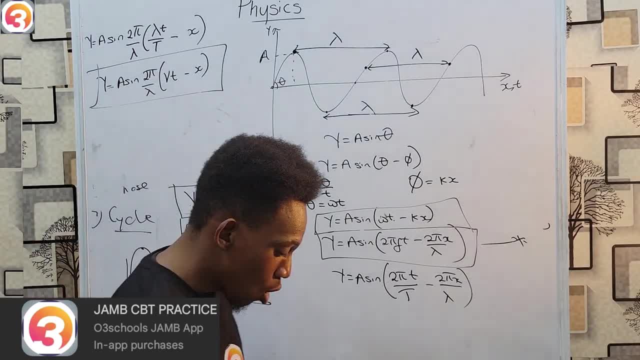 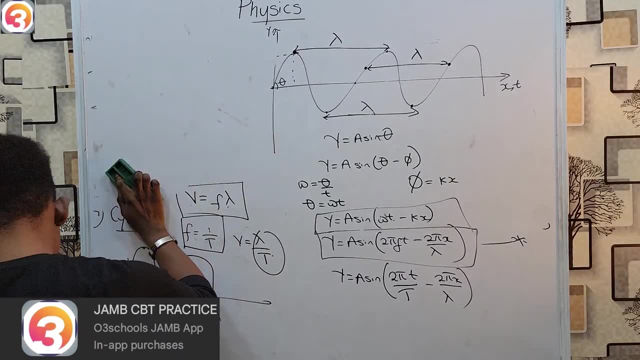 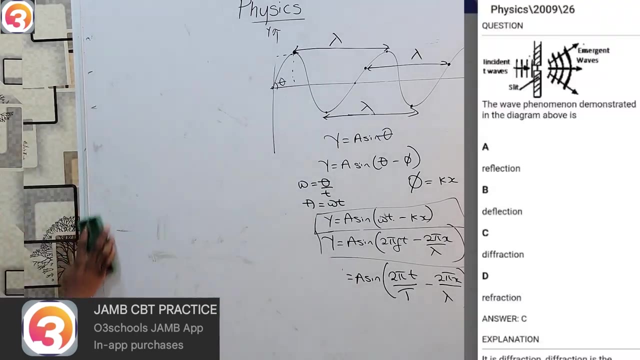 and begin to solve questions on the waves. So let's see. Our first question comes from the year 2009,. question 26.. And yes, you can see the question on your screen on O3Schools Jam app. 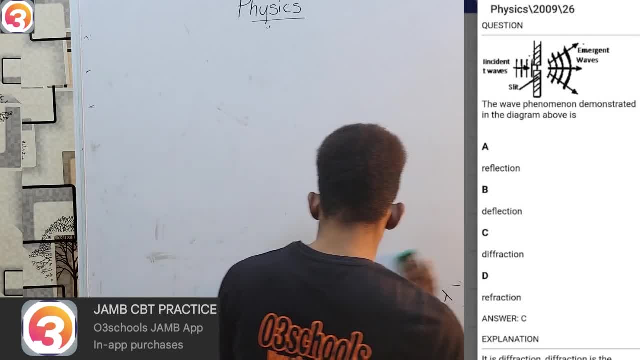 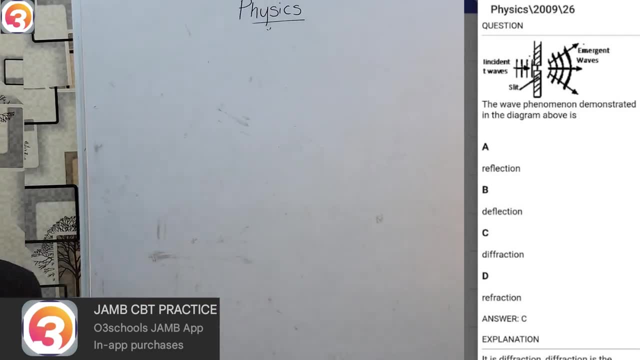 So I will know how to draw it In this question. I've been told there's a slit, a wave passes through and emerges. What phenomenon is demonstrated in diagram above? Now, if you remember what we just learned under the properties of waves, 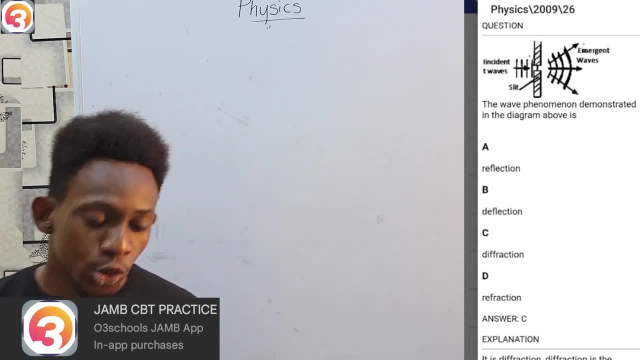 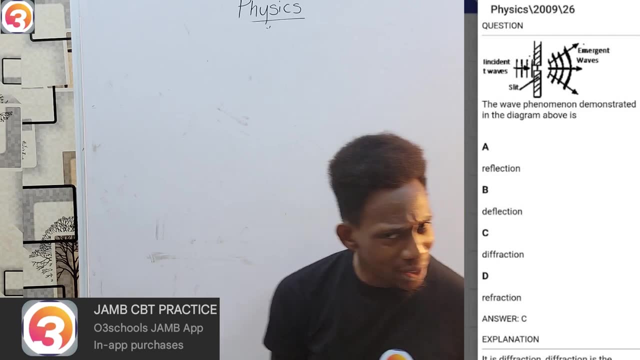 there is reflection. Reflection is bouncing back, not passing through. So that is not it. There is no deflection under properties of waves, So we are ignoring that. I will jump to option D first. for now, There is refraction. 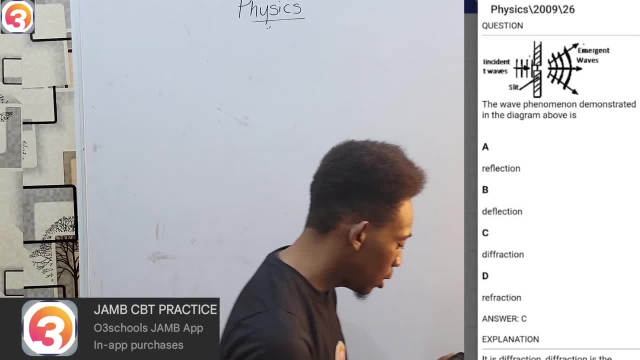 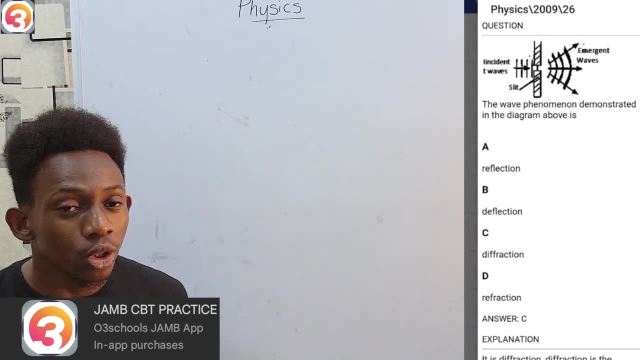 which is a bending as it passes through the boundary. That's what's happening here. Here there is a space and the waves are passing through, And the only property that this is such a phenomenon is obviously diffraction. 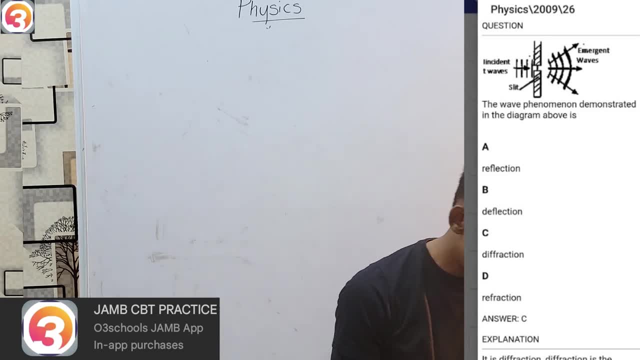 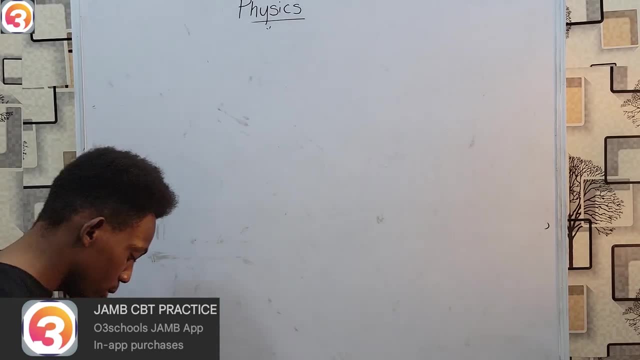 So that is option C. You see, the questions are very, very simple, But now we have one to solve, So let's go with our solving. If a light wave. these are questions to solve if a light wave. 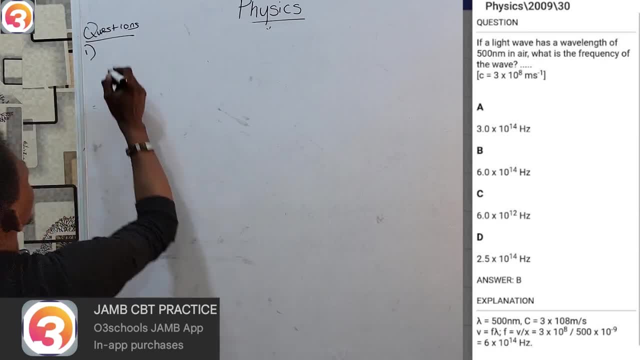 has a wavelength of 500, nanometers. We will also call this Nm. Keep in mind, please, that N here represents nano. This is 500 nanometers. And what is nano? Nano is simply a prefix. 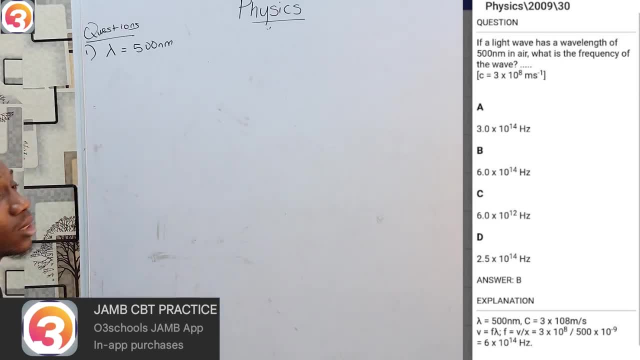 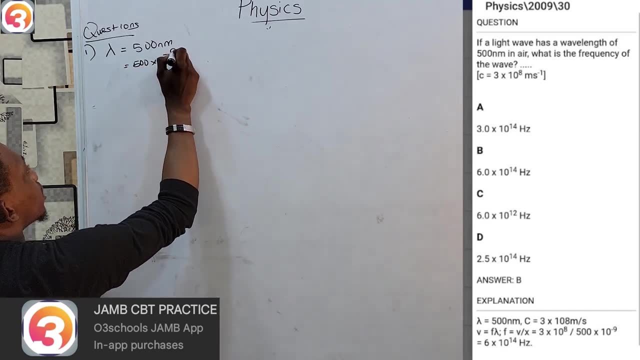 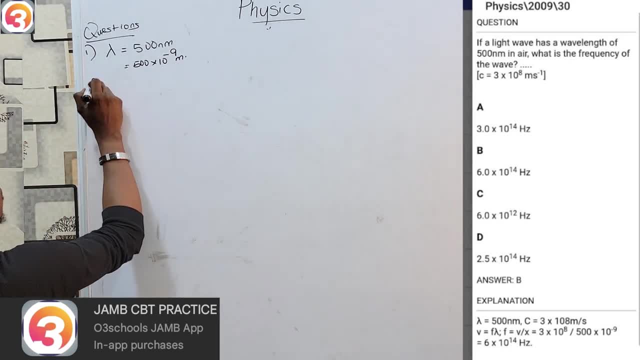 What is this? What is this? I am being asked to find the frequency of the wave, given that speed of light equals to 3 times 10, to the power 8.. Now that is an electromagnetic wave and the speed is quite fixed. 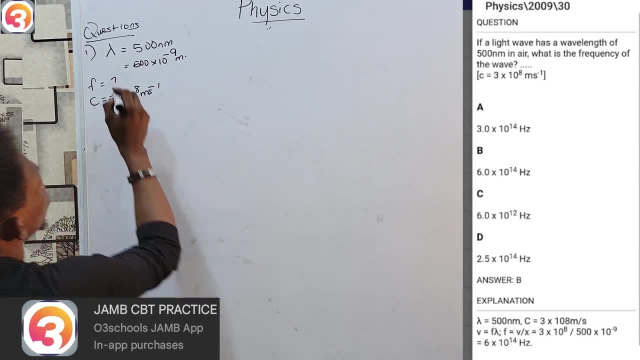 That is why it is related to our c here. So our c is the velocity, which is the same thing as v. We know that c equals to f, lambda, And if I want to find f, f must be c over lambda. 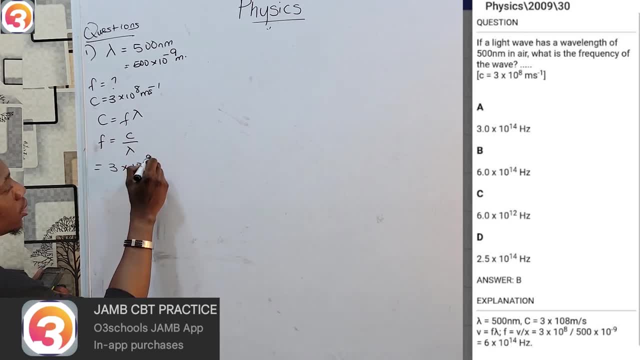 What is my c 3 times 10 to the power 8, and what is my lambda 500 times 10 to the power minus 9.. So what can I do? First things first, let's see if putting this in a standard form 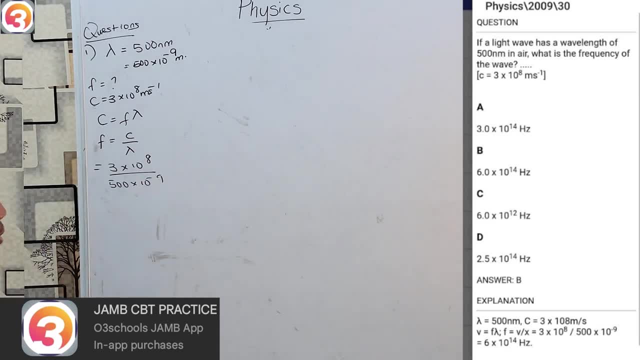 will help me out. This will give me 3 times 10 to the power 8, all over and with my point backwards twice, which is I am adding to here 5 times 10 to the power minus 7.. 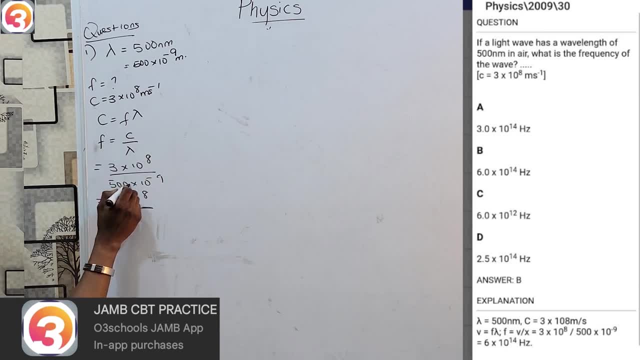 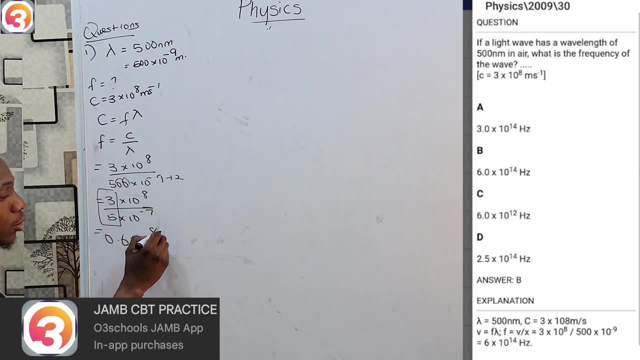 0.6, then 3 to the power 8, divided by minus minus 7.. 0.6, times 3 to the power 8, minus 9, minus 9 plus so 7 is 15.. 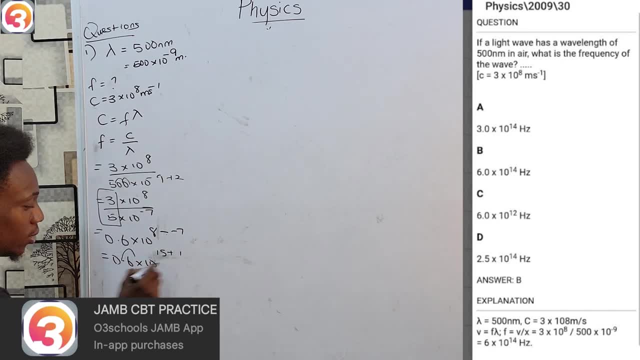 Then I'm going to move by point forwards once and I'll add 1.. So sorry, if I move by a point forwards I am subtracting more, not adding. So that will be 6, minus 3 to the power 14.. 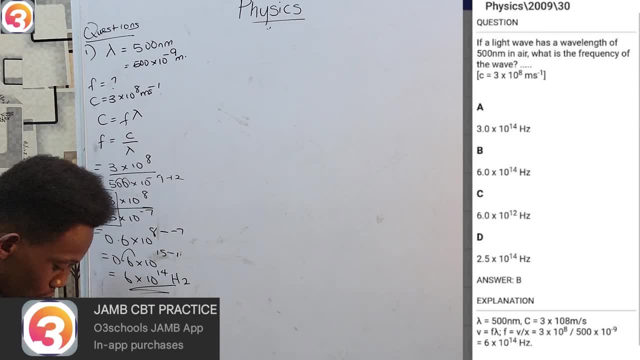 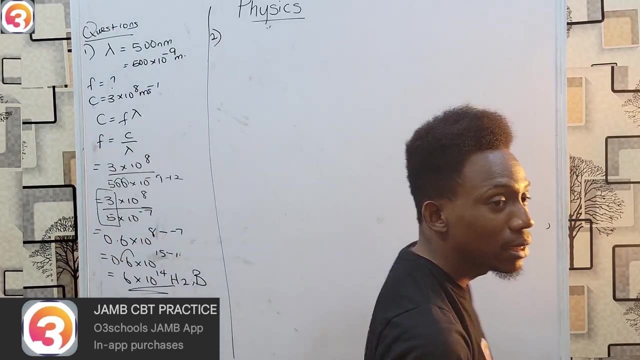 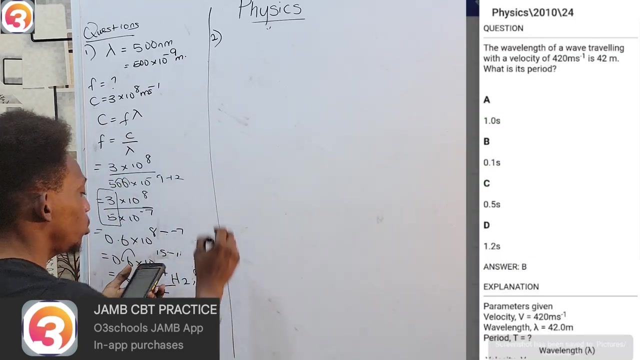 Frequency is measured in, so my answer is obviously option B. see, this question was in the eight or nine question number. sexy. now for the next question. we're going to be a 2010, and now we are looking at question 24. the wavelength of the wave travel to velocity of 120 meters per second is 42 meters. 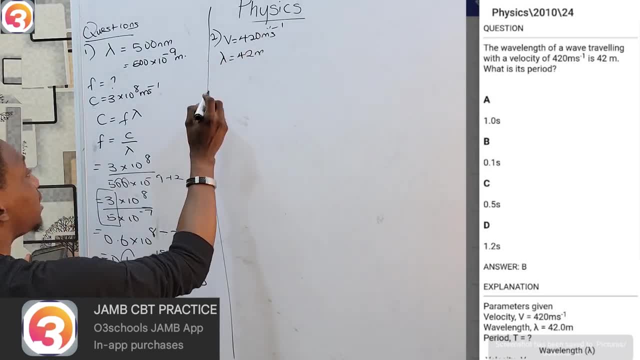 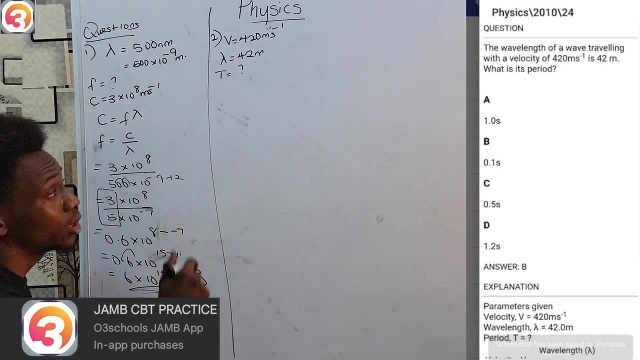 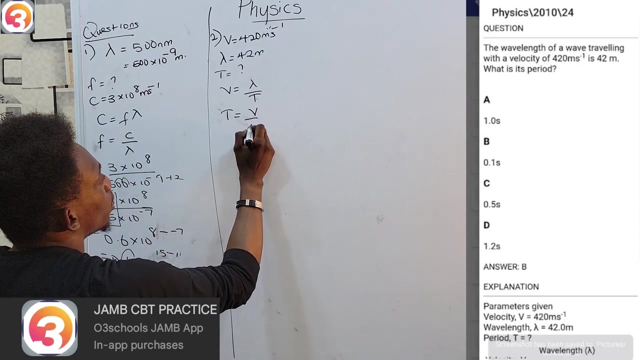 limits for the two meters. where to find the period? did we have a formula relating velocity with that period? yes, noted, our V must be lambda over periods because period is one of our frequency and frequency is one of our period. therefore, to find my period cross multiply, I'm very close to V over faith, equals will be over lambda, I might see will be V or 20. 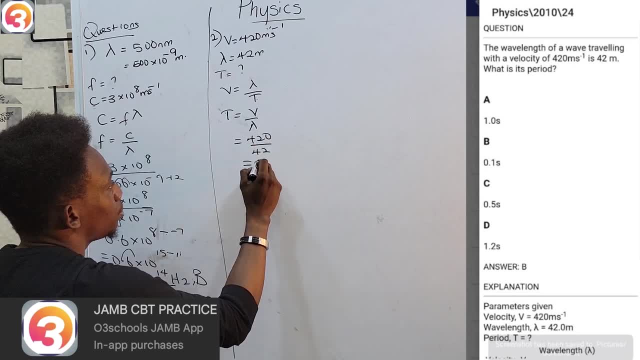 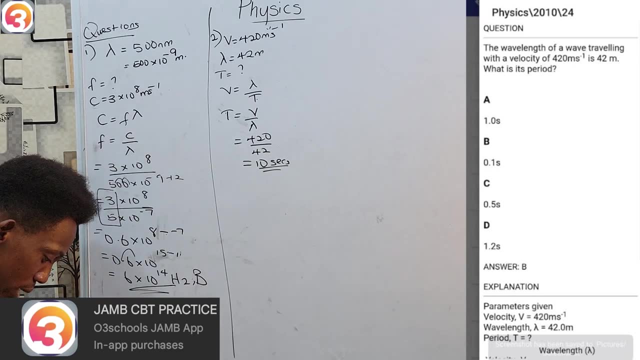 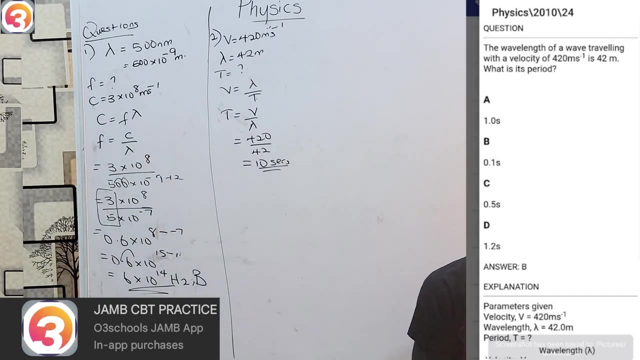 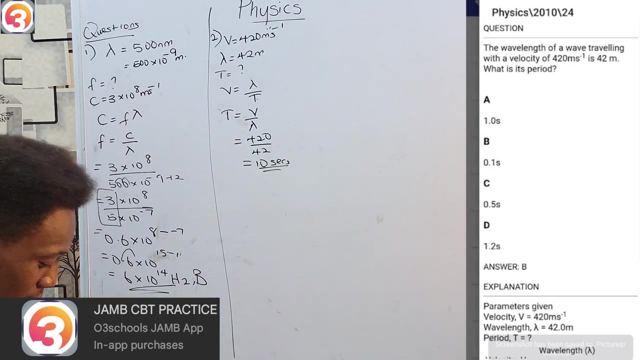 over lambda 42. that is simply 10 seconds JC. another very, very, very simple one. funny enough, do not have 10 seconds in our options, but we're going to stick with that as one answer. what can you do if you have a question like this? I am not quite sure what is wrong. I want to try. 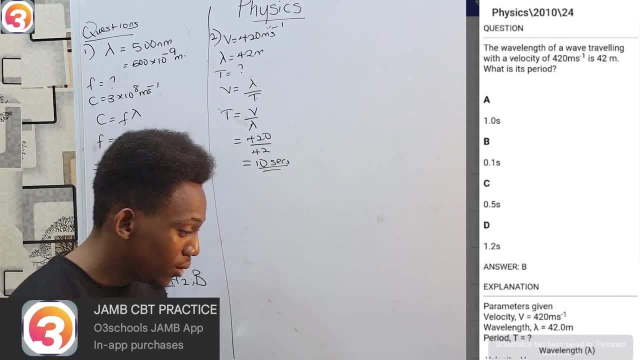 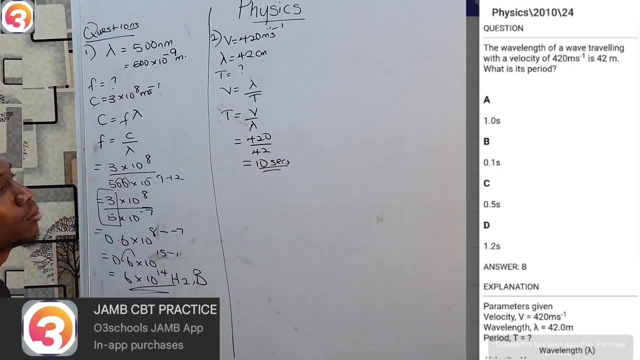 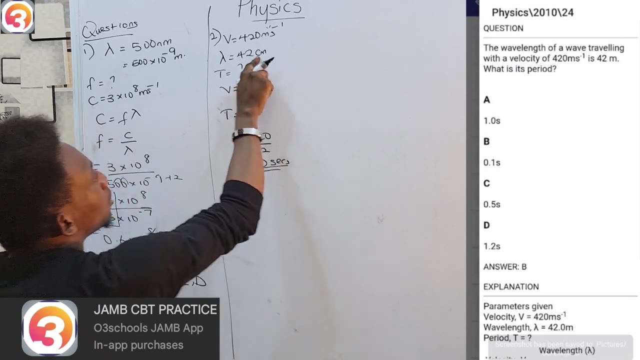 and imagine it was both relative in your jump, what could you do? you could assume, for example: now maybe this should have been in centimeters. if we try that with that work, no, because we convert this from centimeters to meters, that will make Lambda reduce. I'll make my answer increase, but look at the options. all my answers. 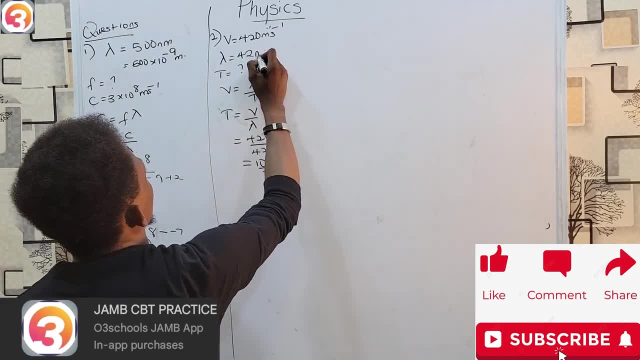 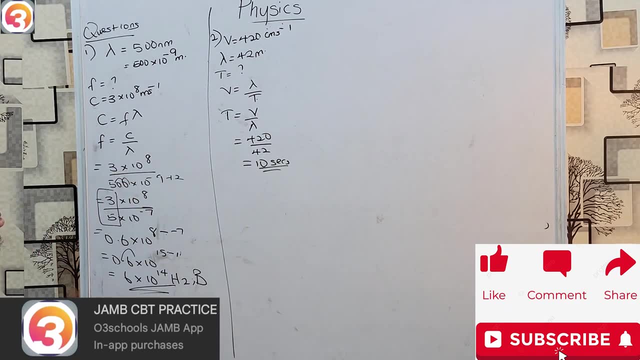 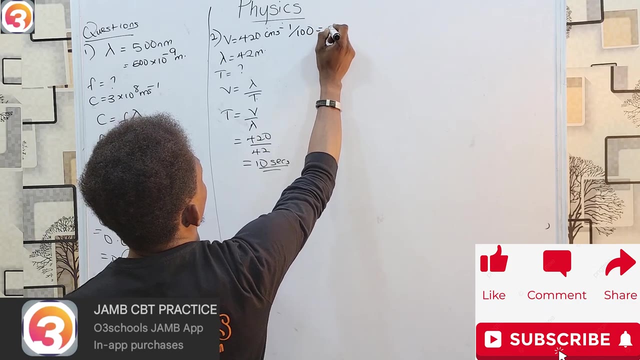 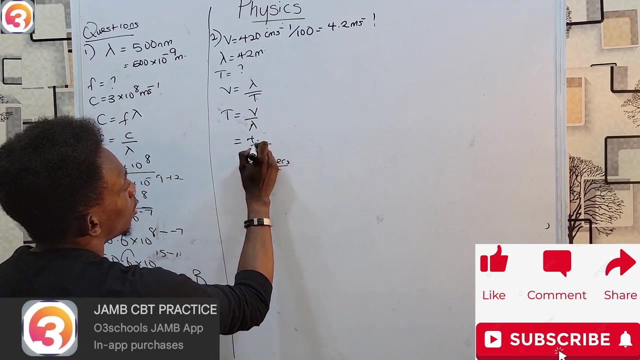 are smaller. therefore I cannot try centimeters. I could then say: okay, what if this, instead was one of the centimeters per seconds? this was centimeters per seconds. to convert to meters per seconds, I will have to divide by 100, which will make it 4.2 meters a second, so that I still, 40 or 20 years, I'll be having 4.2, and 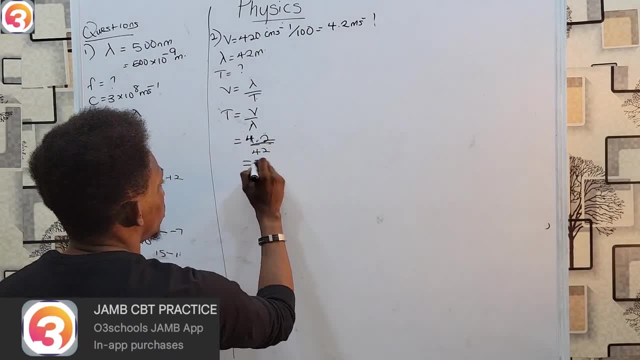 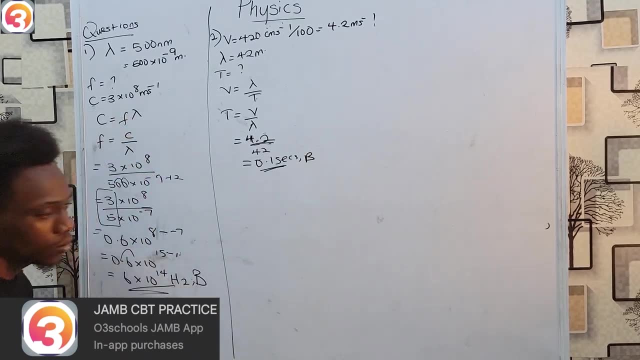 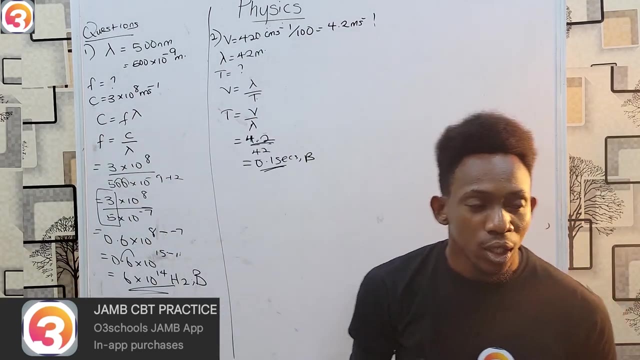 having 4.2 over 20. I then get 0.1 seconds, which is in my options, and that is option B. now please note: I don't recommend you wasting much time trying to correct a question in your exam if you solve and you know you solved correctly, or your answer does not appear in the options. 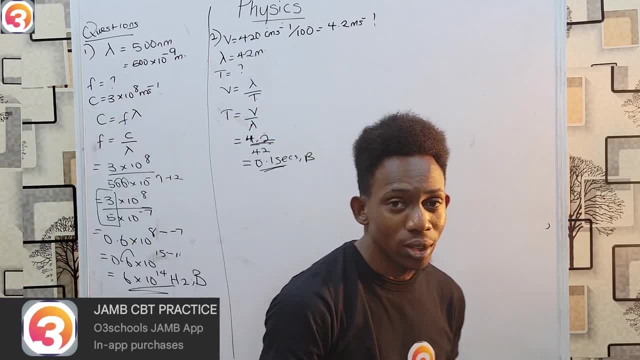 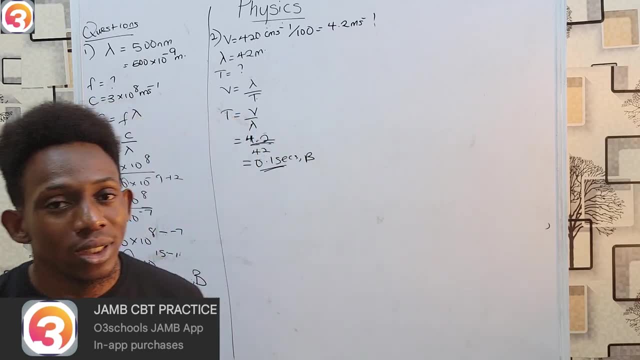 I will advise you to split, guess the closest one and move on or, if you want to, you could leave that question and come back and tackle it if you can finish your exam on time. but do not waste your time when you know you solved the correct thing, already trying to resolve and resolve to get the 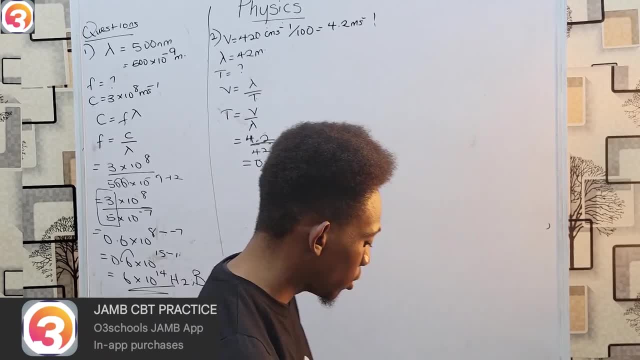 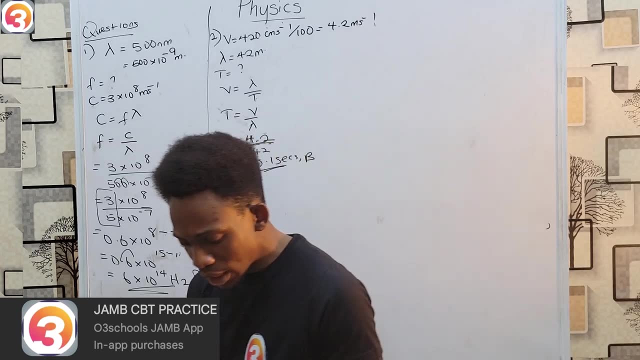 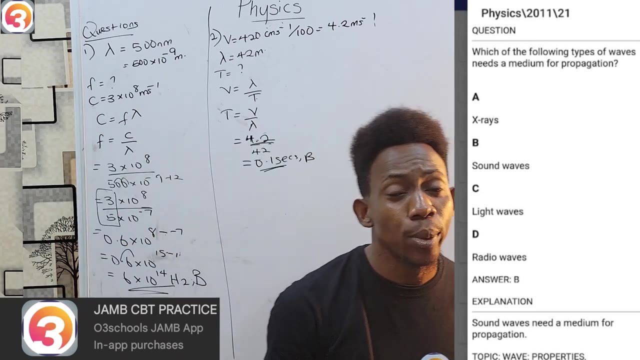 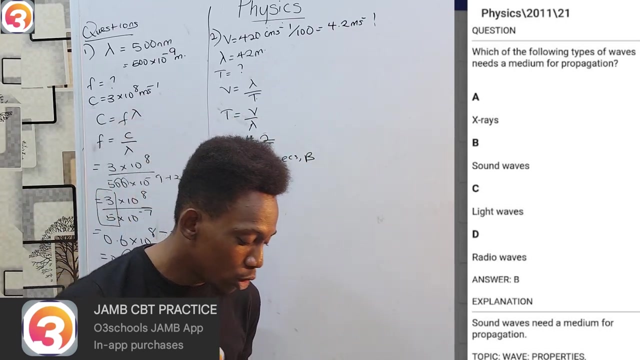 answer as long as you are sure that your first solving was correct. okay, our next question is from the year 2011 and this is question number 21. which of the following types of waves needs a medium for propagation? remember you've tapped that it's medium, ah, mechanical waves- why Wars gravity? Türmal needs power medium, so option a: x-ray. şekkürlar to magnetic. so no sound waves will continue to help. more related questions in this class. we know there will be newer that make the players stronger. you feel strongly interested, know sounds good, so remember to hit the bell button and have a good day. bye now, thank you. see you soon. 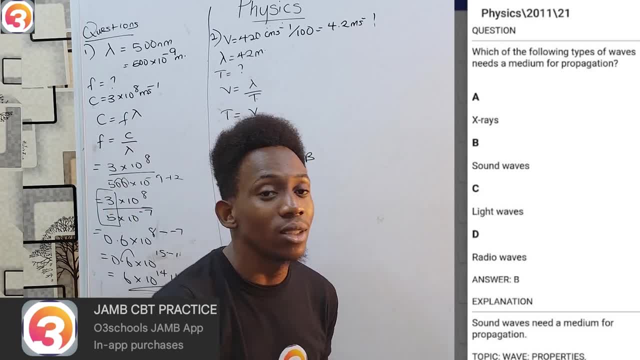 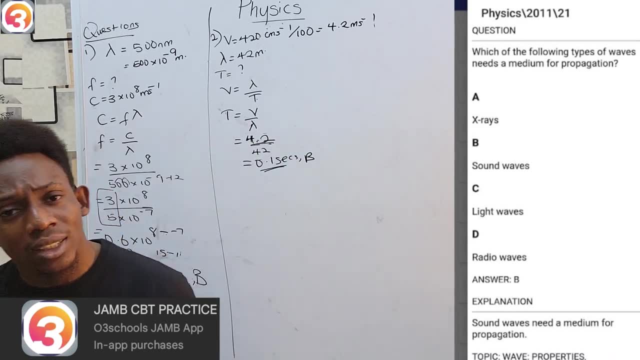 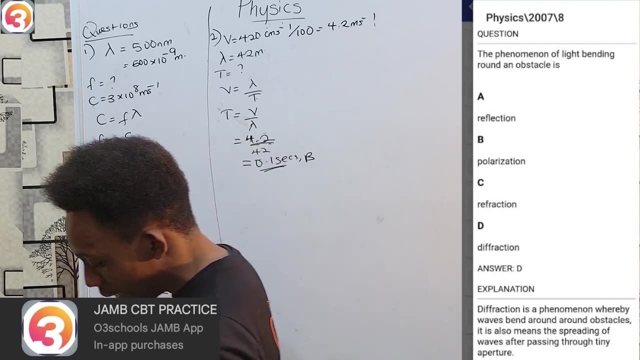 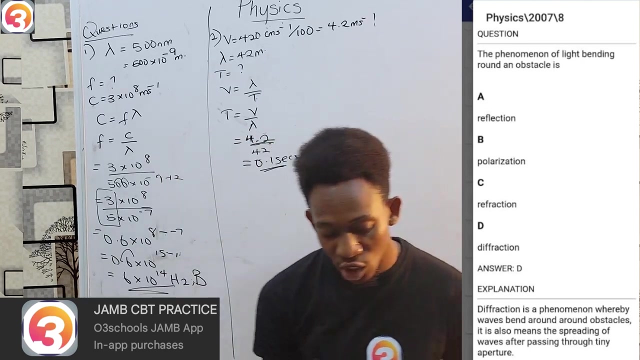 sound wave is mechanical. so that is my answer. mechanical waves are the ones that require material medium. then um, the next question, 2007 question eight. also theoretical, the phenomenon of light bending around an obstacle is known as diffraction. see, that's like bending around the obstacle, which is the spreading out after passing through a tiny space. diffraction option d. 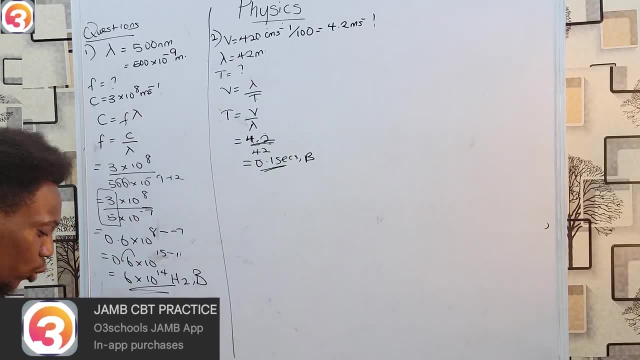 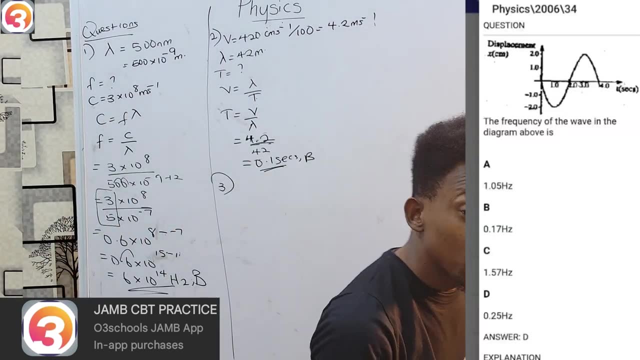 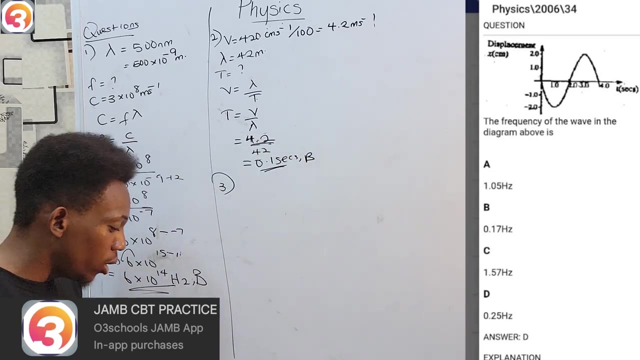 next we have a diagram. this one is quite interesting. this is from the year 2006, question 34.. now there's a diagram which you can see. obviously, when the auto risk goes up, then in this diagram i have a wave. right now this wave moves, and the last time we noticed on the 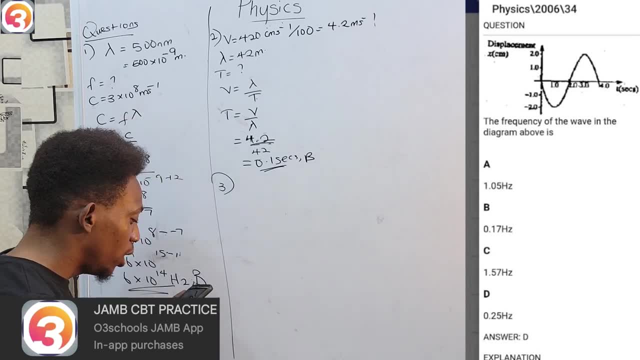 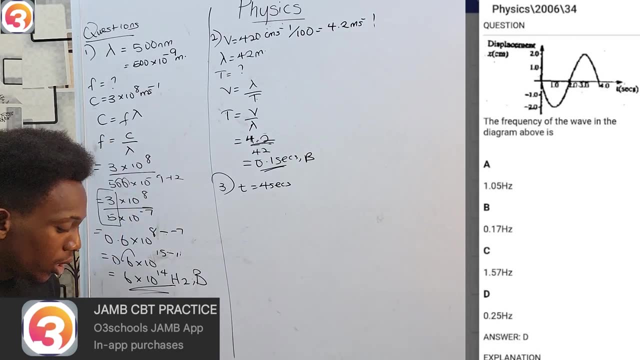 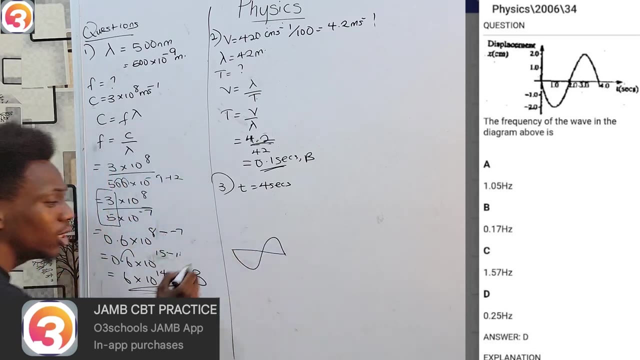 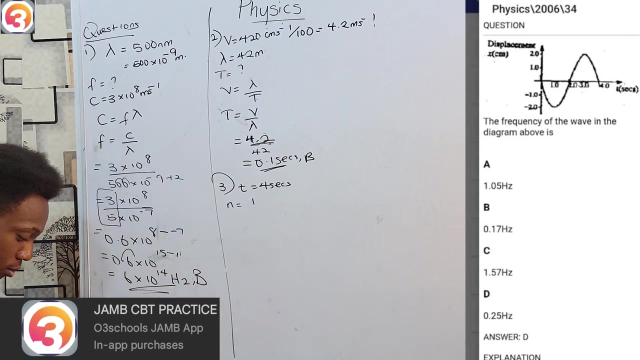 time at the horizontal part of the graph is that the time it used was four seconds. however, in that four seconds, how many cycles has it completed? you noticed it went simply like this: this one cycle go and come. therefore, number of cycles is one, and what is your wavelength? wavelength is the distance from peak to peak press to. 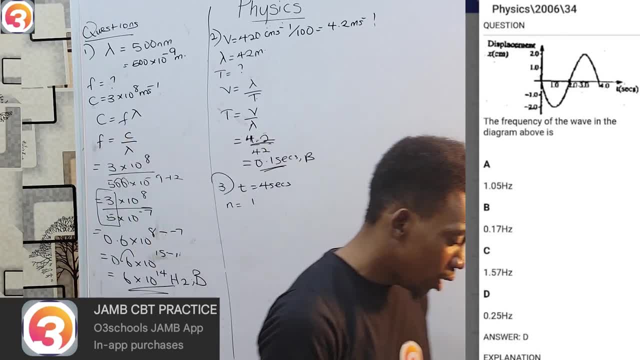 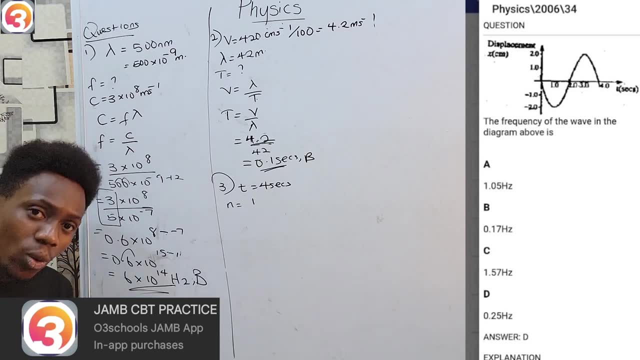 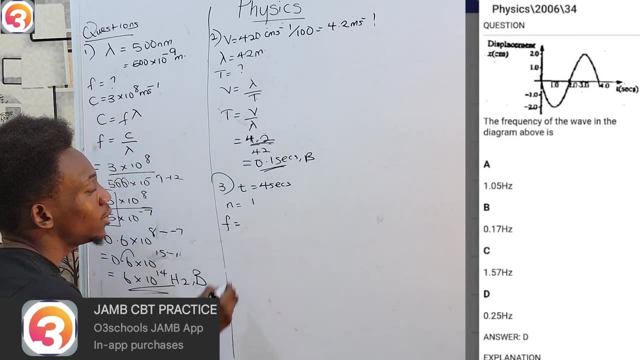 crest or trough to trough. also, you could say wave x is a distance from middle to middle. so do i need the wavelength right now? no reason why i'm simply asked for frequency. but let's talk about wavelength. i just need to know that for frequency. frequency is number of cycles over time. how many cycles? one, how long? four seconds and one over four? 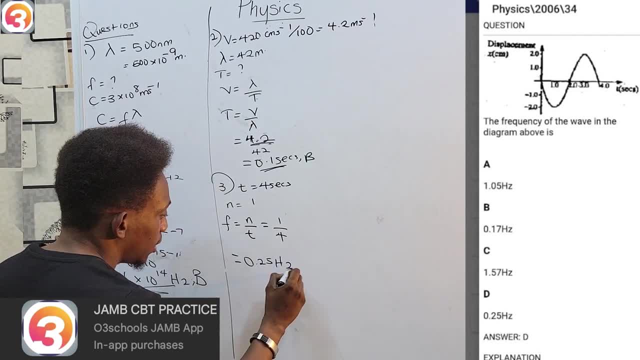 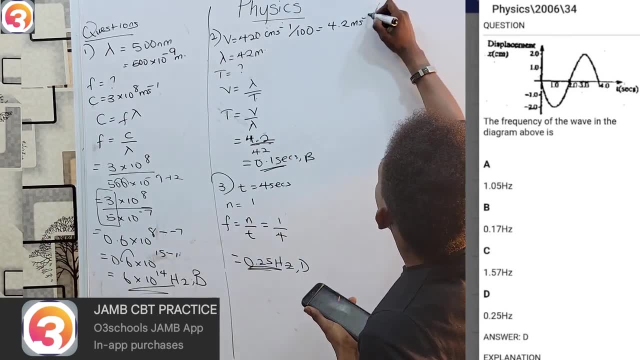 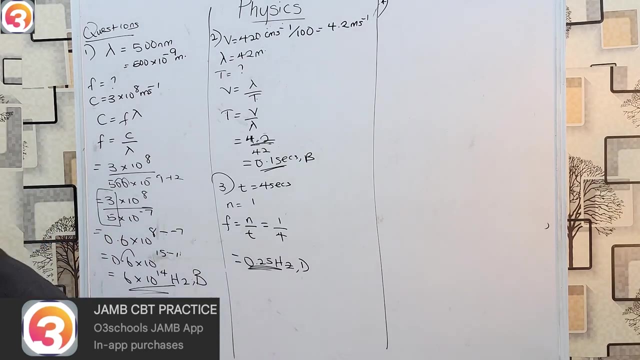 must give you 0.25 x. see, my answer is option d. so as long as you know your basic steps, you should not be having any issue. okay, question four. for question four again, this is theoretical. let's look at the answer. this is from the 8004. 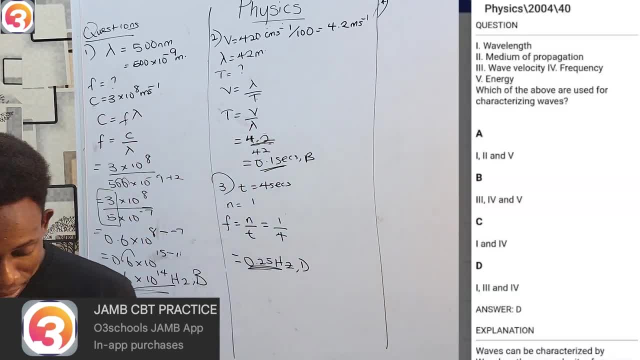 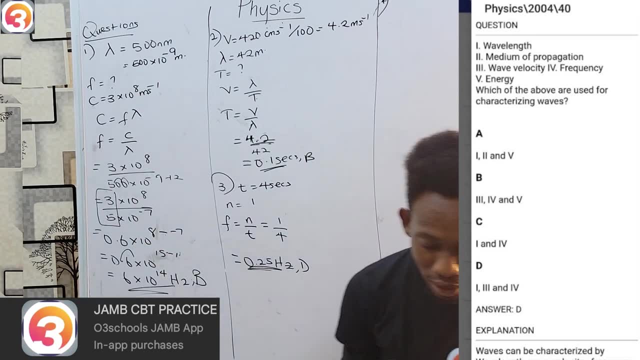 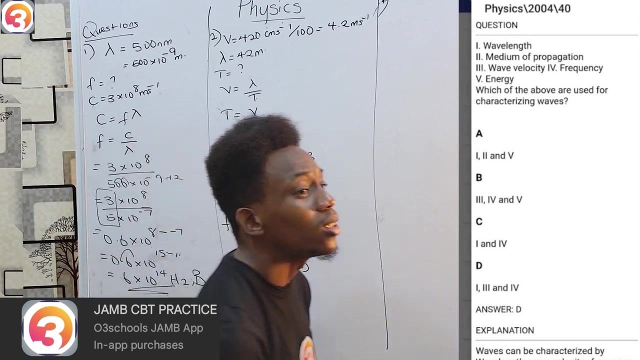 question number 40, 2004 number 40.. then we are told one is wavelength, two is method of propagation, three is wave velocity, four is frequency and five is energy. which of the above is used for characterizing wave? which of the following are things used when describing waves? do we use wavelength? yes, of course. so we know our option. 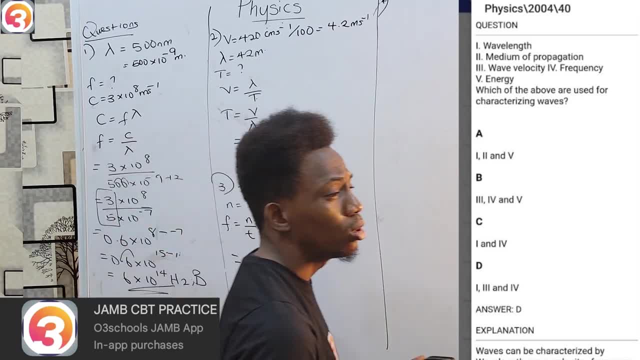 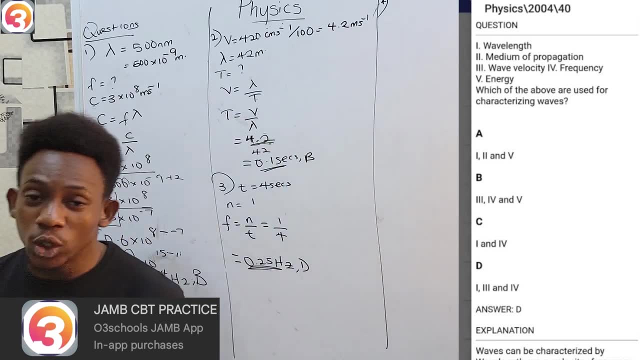 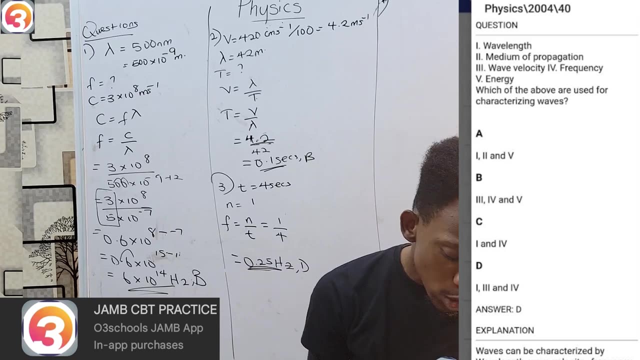 must have one. do we use medium propagation when describing the wave? no, that's on that path, so don't use describing the wave. do we use the wave velocity? of course. so one and three, right. I don't have to continue analyzing. look at my options. only option D. 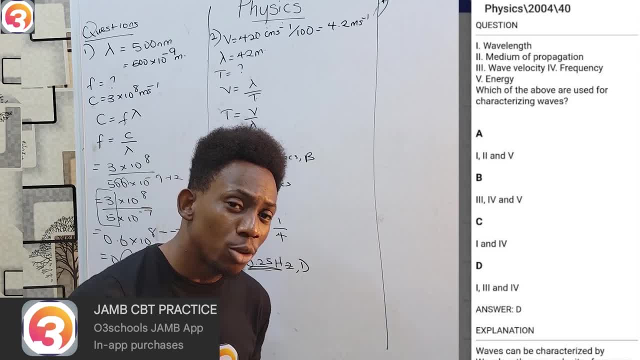 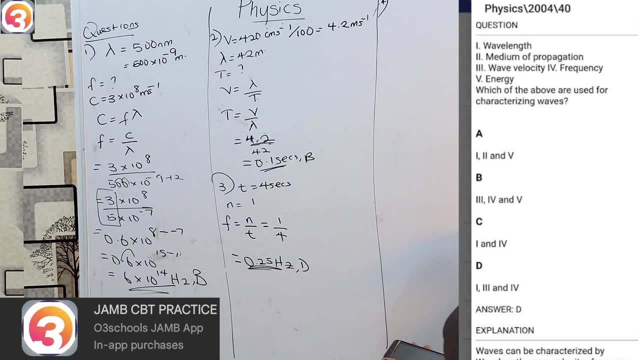 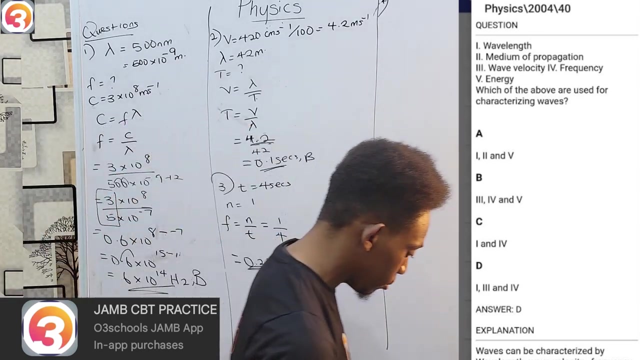 contains one and three. therefore, I know my answer must be D, which is one, three and four, because, remember, when describing wave, you must look at, like the terms we described, you must look at the velocity, the frequency and the wavelength. so those are things to use describing wave: 1, 3 and 4. okay, next up, we're in the year 2004. 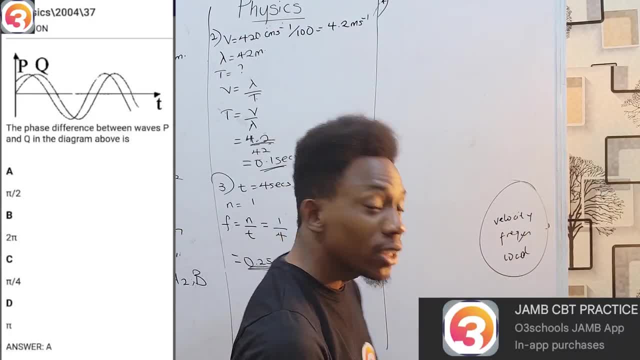 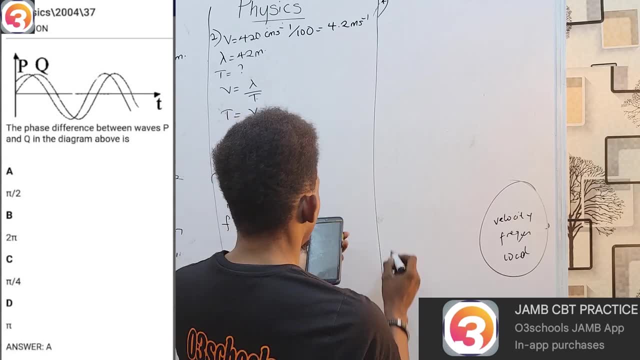 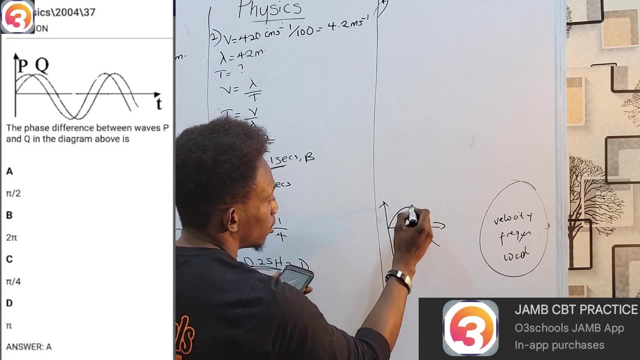 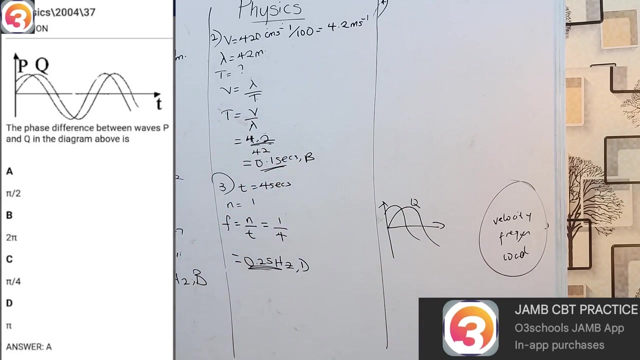 now question number 37. again, you can see this diagram. the phase difference between waves p and q is what? now? look at this diagram, something like this. we're gonna drop a simple version here. wave Q is like this, wave P is- maybe that more like this. so, if you notice, wave q is at its bottom, while wave p is still behind. now this one's. 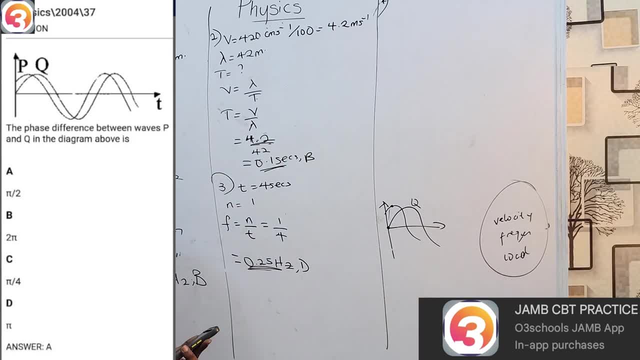 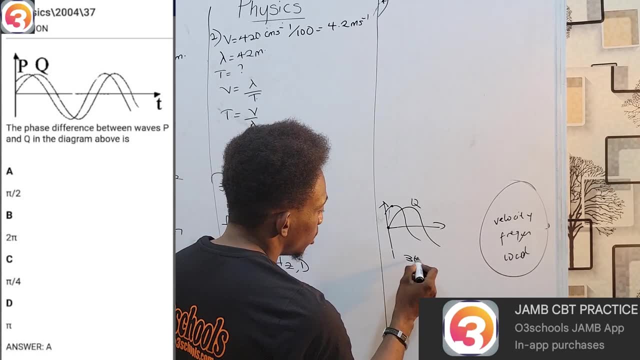 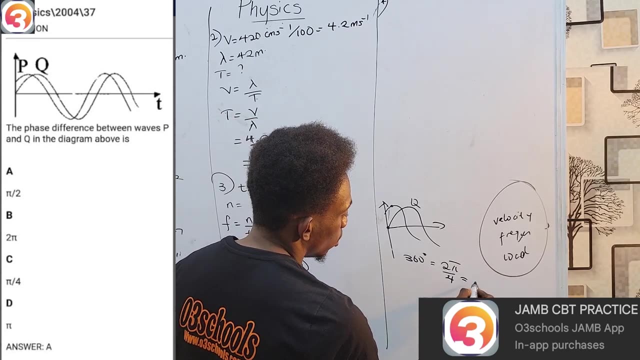 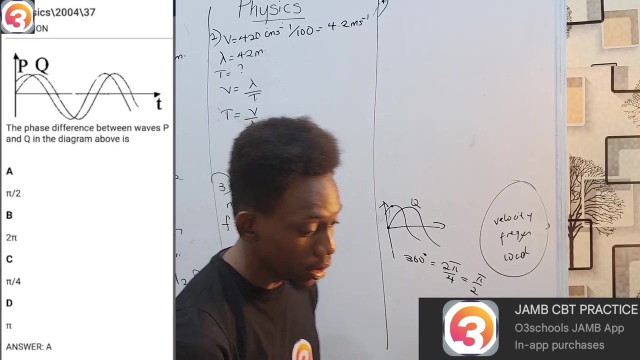 peak is where this one's bottom is. therefore, it must mean that it's basically a quarter of a cycle. behind his cycle is 360 degrees, or two pi. so what's the quarter of that? two pi over four, which is pi over two. see my size a. this is more mathematical than physics, just trying to have 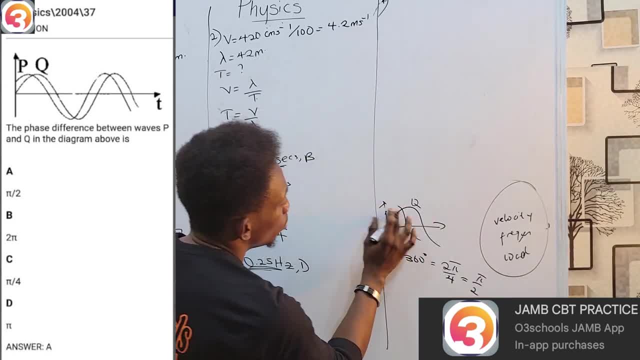 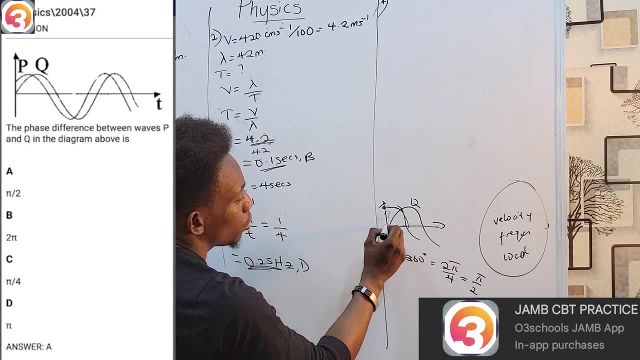 a good handle of your mathematics, just because i know this wave is having a speaker right. one is here. therefore, by the time this one has reached here, this one that was already gone, five again, so there'll be. there's a gap between them. therefore, that gap is pi over two radian. 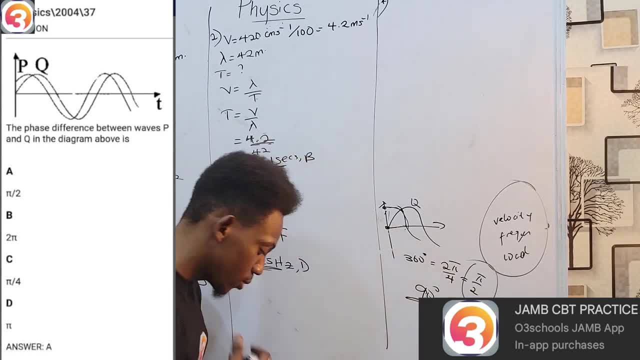 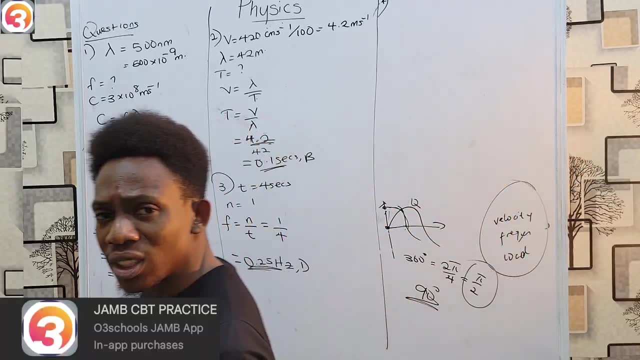 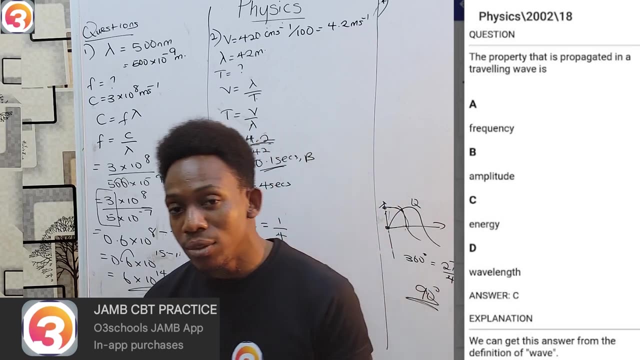 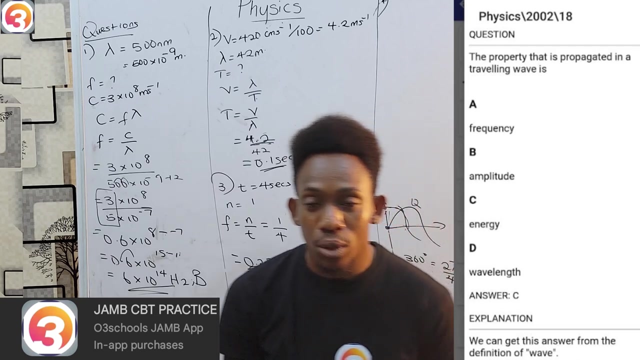 or it wasn't degrees, it was maybe 90 degrees. so that's that, okay. um, next, again theoretical. from the 2002 question 18: the property that is propagated in the traveling wave- we've actually been propagated in the wave- is what? frequency, amplitude, energy and wavelength. and if you recall, even from the definition, we set a wave of the disturbance. 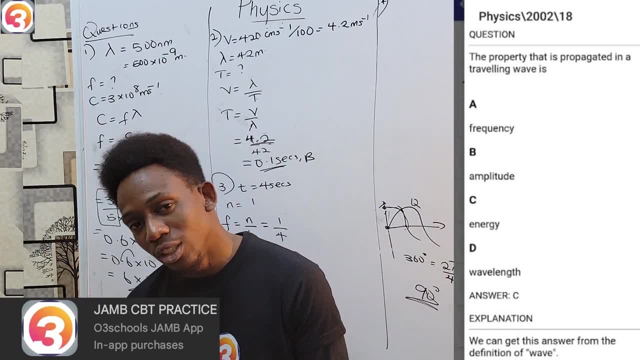 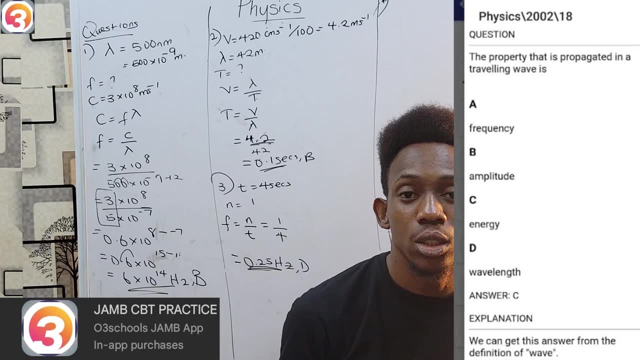 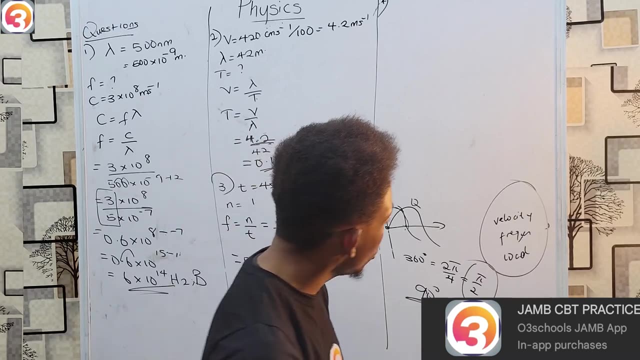 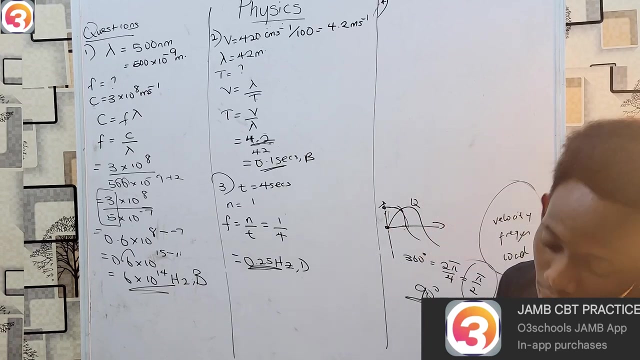 which travels through a medium by getting energy. we are trying moving energy. therefore, the property being propagated obviously must be the energy, and that is option c. so okay, we now have a question. this one will require a bit of solving. a traveling wave moving from left to right has an amplitude of 0.15 meters. 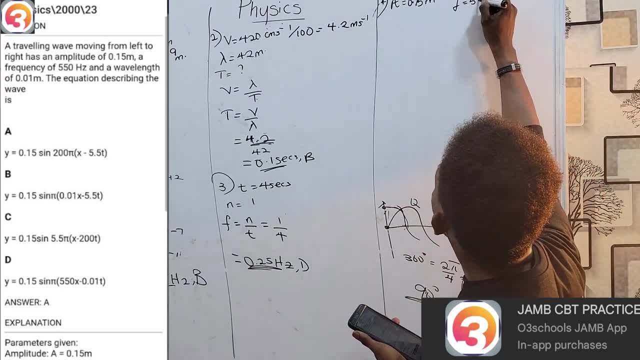 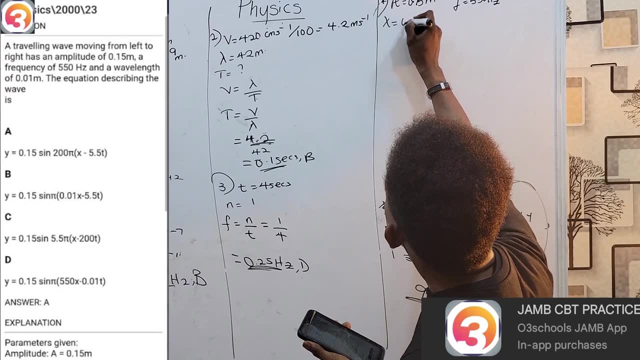 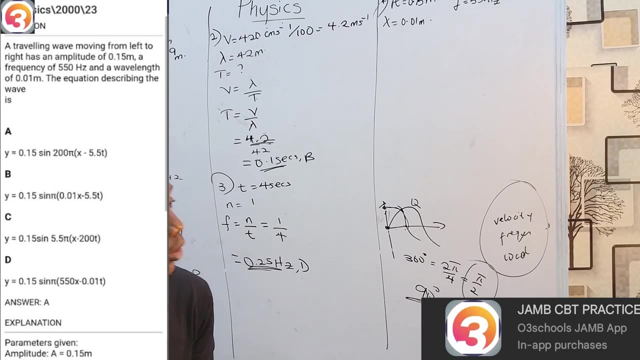 a frequency of 550 hertz and a wavelength of 0.01 meter. the equation describing the wave is what? now, obviously, we know. the general format is that y equals to a sign, blah, blah, blah. but if i look at these, my options, in all of them i'm having a number after my sign. 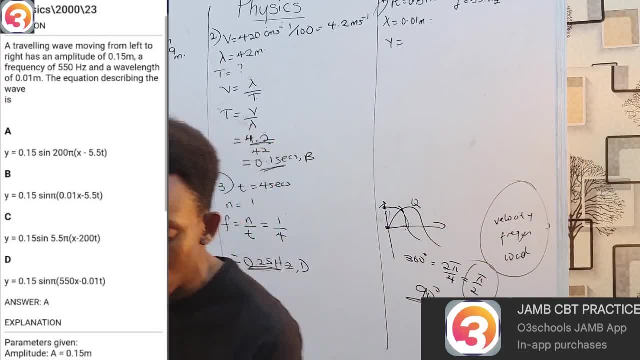 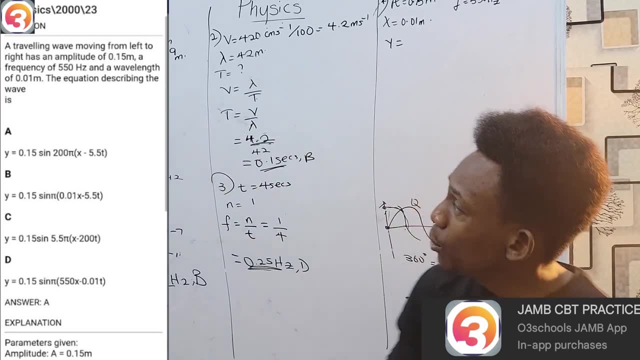 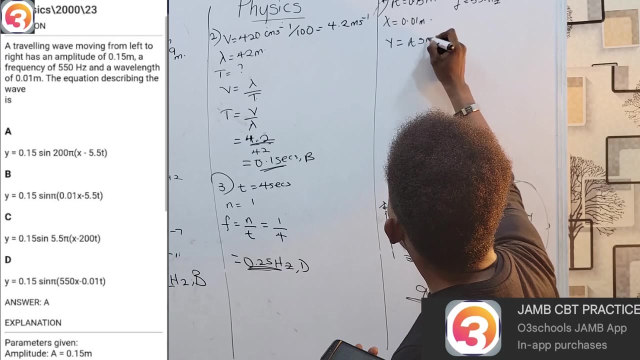 notice: option a is to sign 200 pi, option b is sin pi, c is sin 5.5 pi and d is also sin pi, which implies if your number is coming out, like we said before, therefore, that must mean there's only one type of formula to have a number outside. if you remember, that would be a sine 2 pi over. 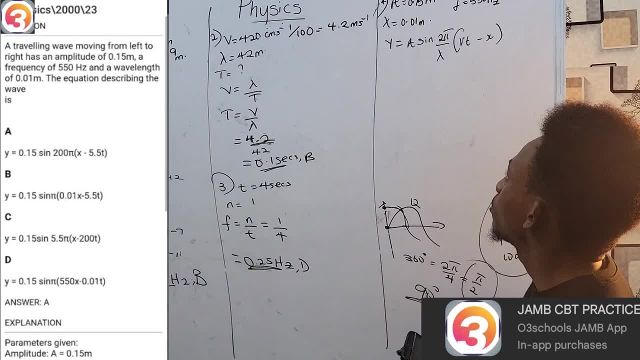 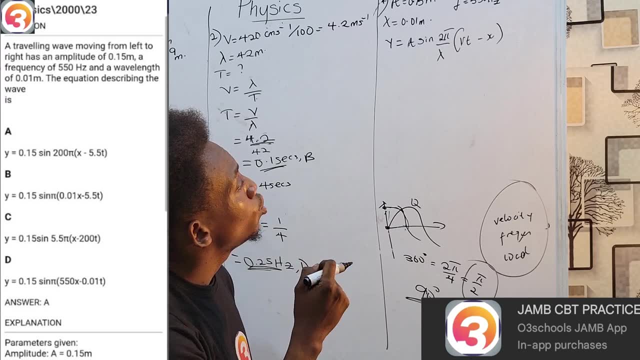 lambda into vt minus x. so that would be a sine 2 pi over lambda into vt minus x. that would be a sine 2 pi over lambda into vt minus x. that means for my wave to be described in one of the options. that must be it. what can i do? it may start to get everything i need. i must know v. 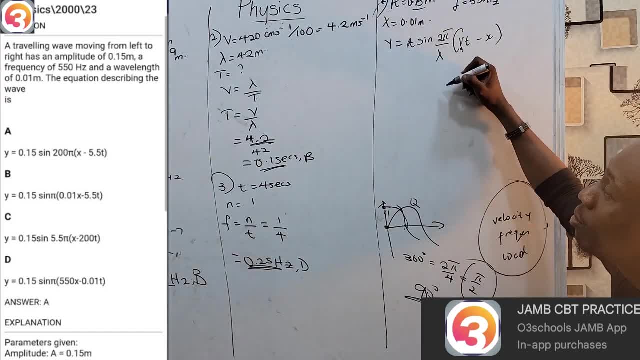 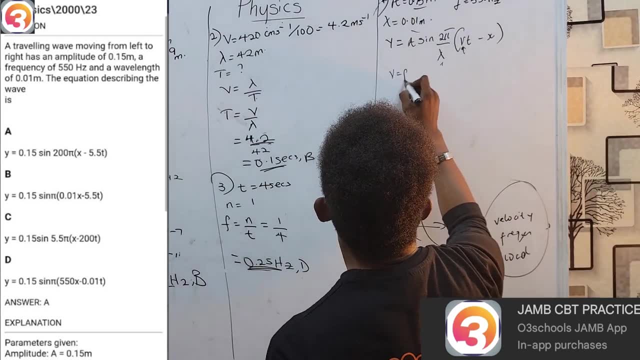 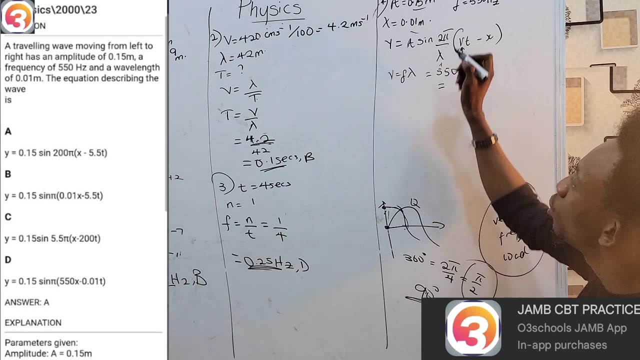 and that basically i need to know. i know a is given to me directly, i know lambda also gives me directly, but can i get v? yes, v equals to f lambda. that'll be 550 times 0.01, and 550 times 0.01 is 5.5 and therefore, quite simply, y will be close to the amplitude a- 0.15. 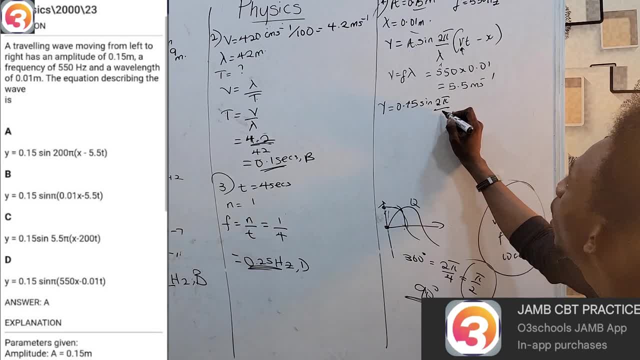 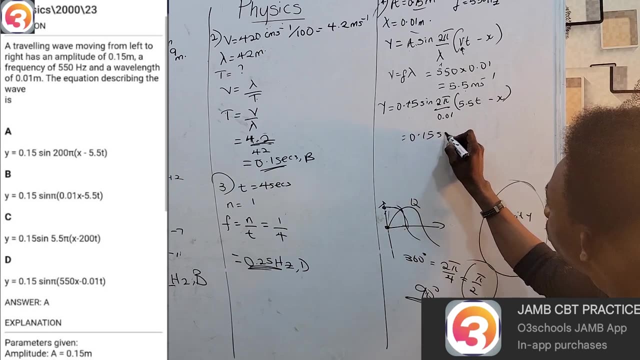 sine 2 pi over what is lambda, and that is 0.01 into v, 5.5 c minus x, that will be 0.15. sine 2 by 0.01 is 200 pi into 5.5 t minus x, and that is option a. 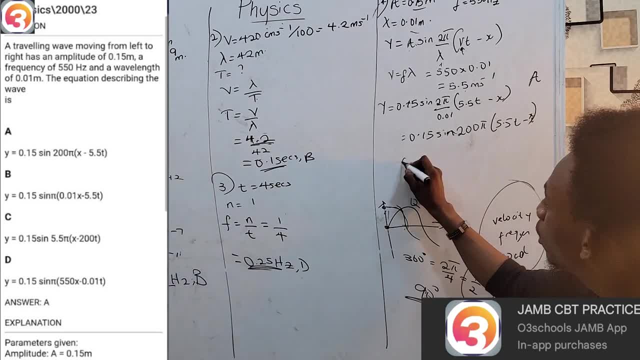 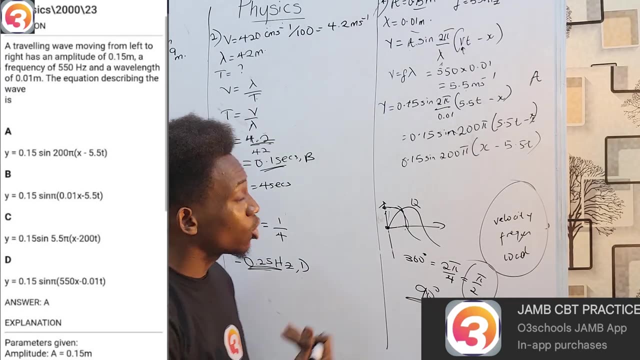 if you look at option a, there's a small difference. option a is actually 0.15 sine 200 pi into x minus 5.5 t. now if you cry, i told you, the big difference you care about is that i in mind even if x coming first, or the t on coming first, even if it's plus. 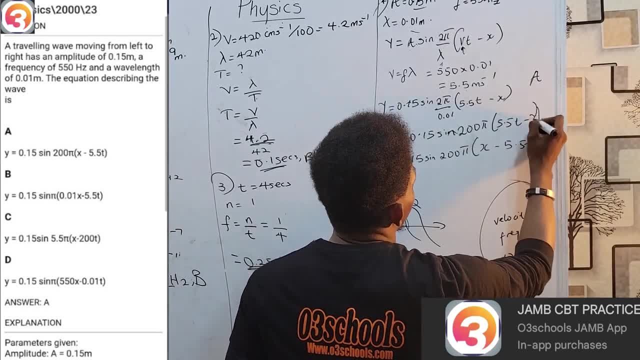 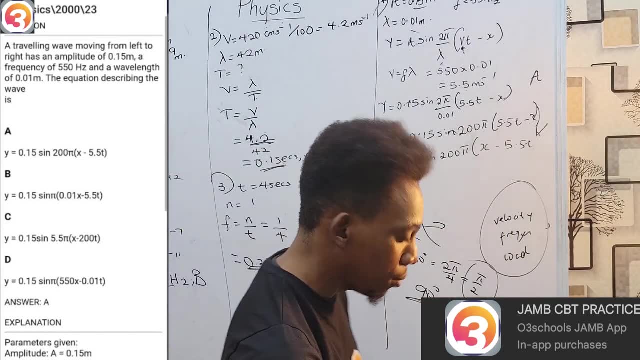 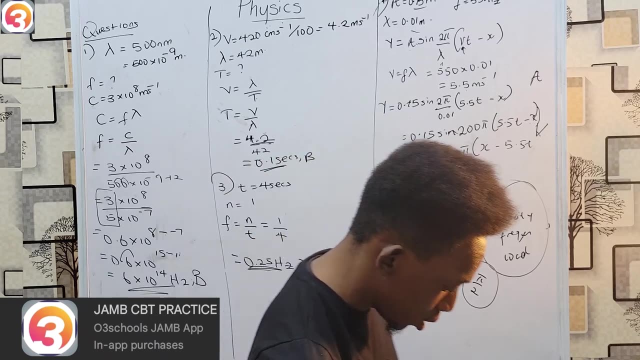 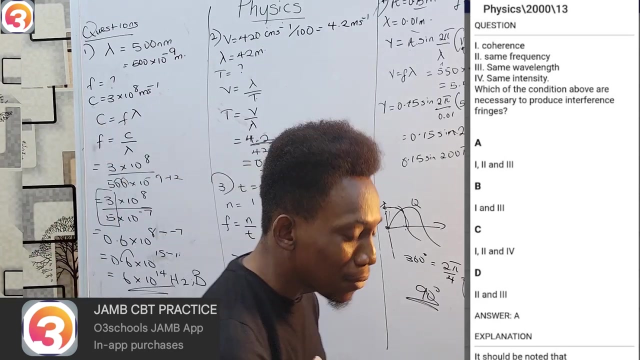 by simply focusing on the numbers inside. so this is my answer. is that, okay? the steps are very, very, very, very simple, okay? um, the next question we actually have now is asking us a very simple thing. it says which of the following conditions are necessary to produce interference ranges: 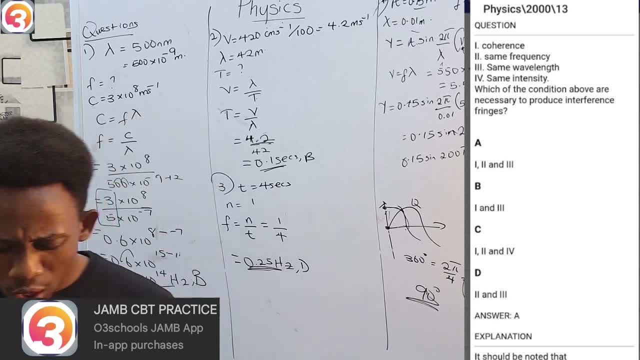 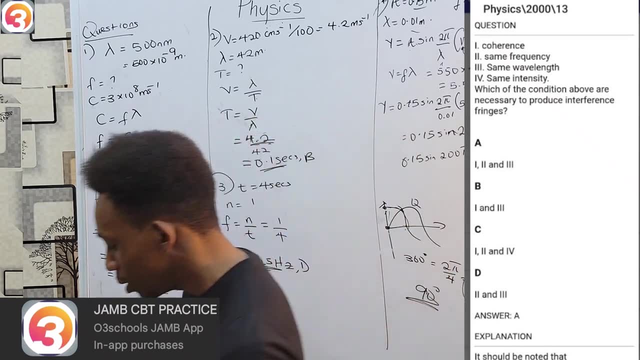 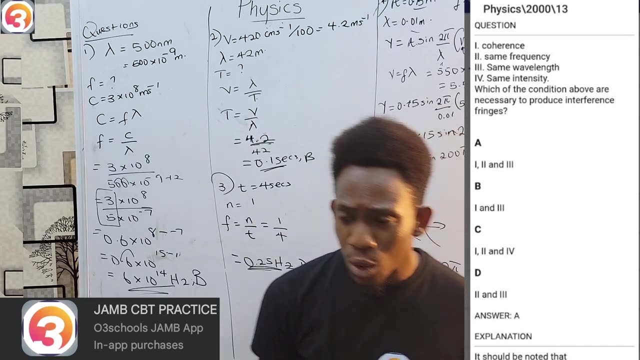 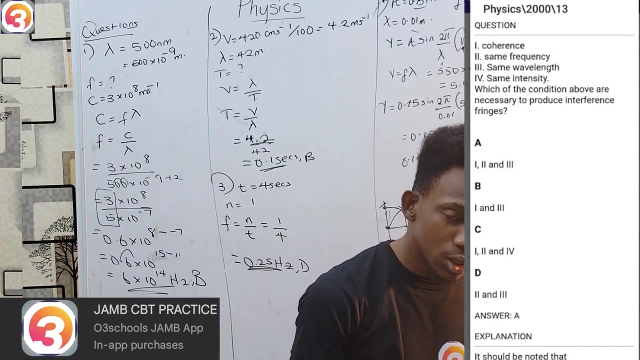 for two waves to interfere with, interference will occur. what must begin? the wave? option a, rather, we have numbers now. the first one is coherence. this one is same frequency, same wavelength and same intensity. now, if you remember, when we explained what is is meant for interference, we didn't measure intensity at all. so that's out of it now you. 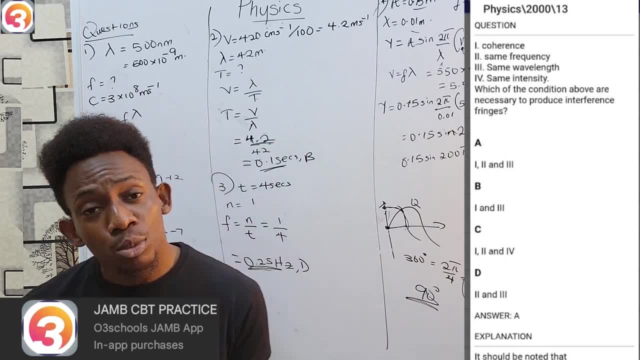 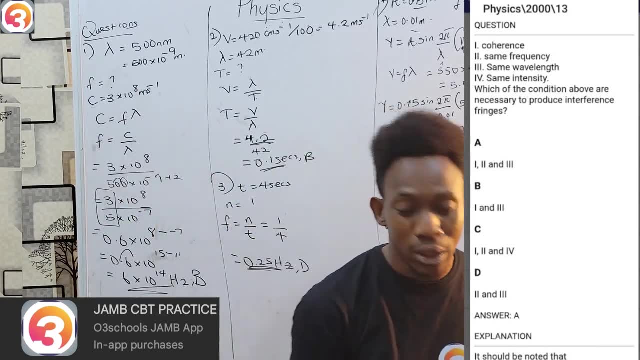 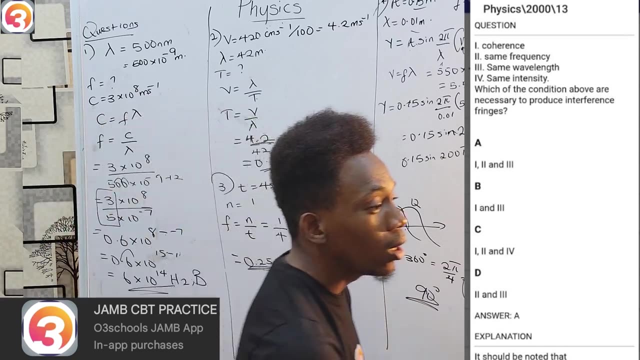 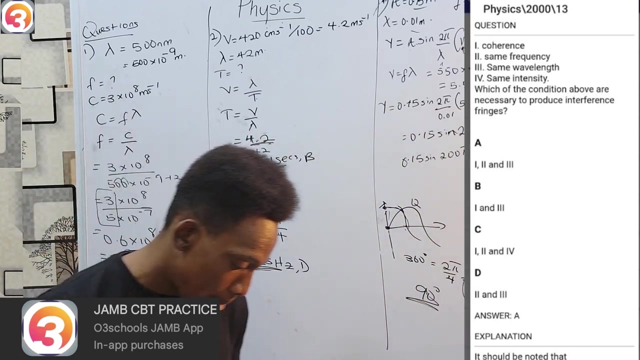 may also say with no major coherence, but we said the waves must be moving similarly to each other for interference to occur. same direction, double coherence means they have the same form, same frequency, yes, and they have the same wavelengths. therefore, any way with those properties can undergo interference. that's that. this is from 2013.. now, from the year 1997. question 47. 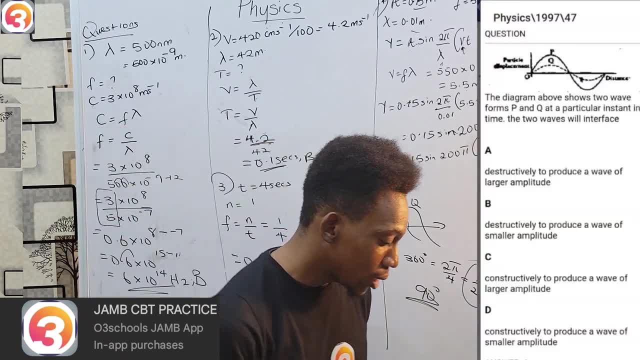 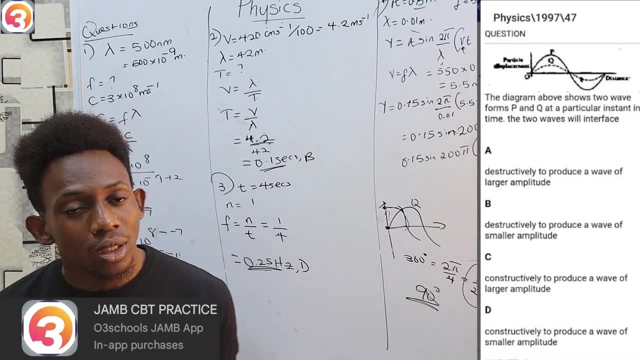 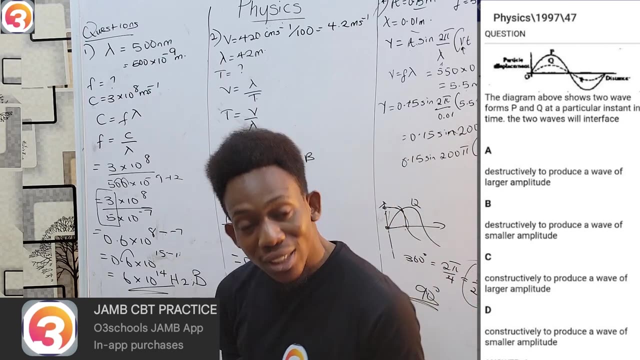 there's a diagram. questions be asking us. basically, they are going to interfere, but what kind of interference will occur? now, if you look at these two waves, they both go up together and come down together. they are in phase and because they are perfectly in phase, what we undergo is constructive interference. i'm going to join together to 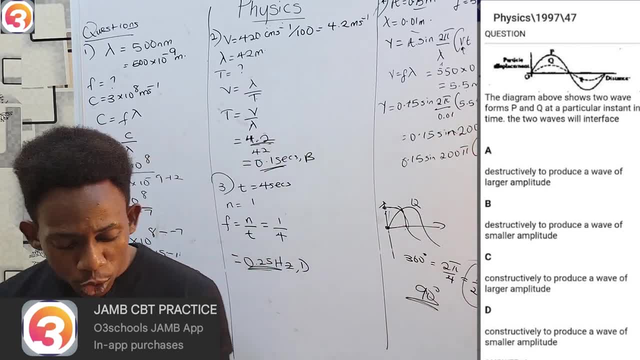 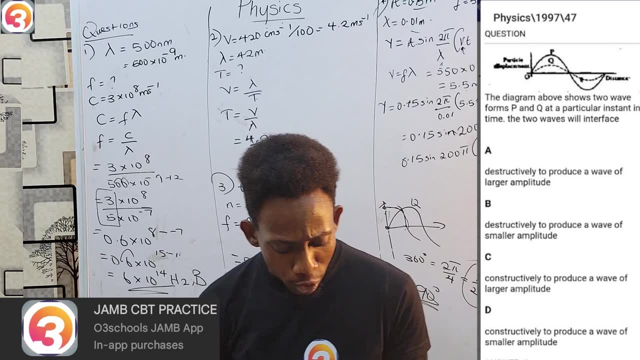 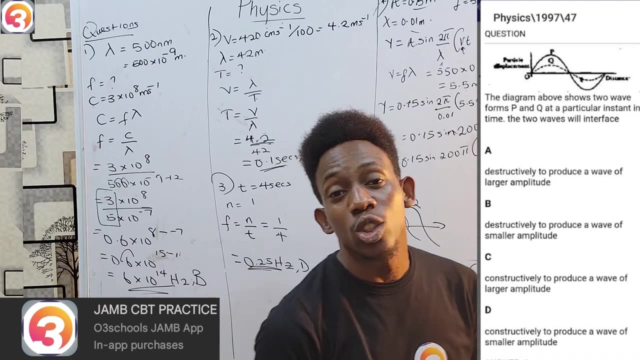 form a bigger wave. therefore, my sum of the options: c it is constructive, but c and d, d is saying they will construct from a wave of smaller amplitude. y, c saying they concerted from the wave of larger amplitude. i cannot join two things together and they are both positive and get a smaller thing. 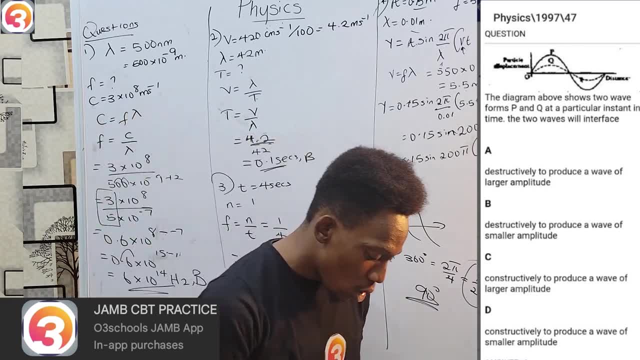 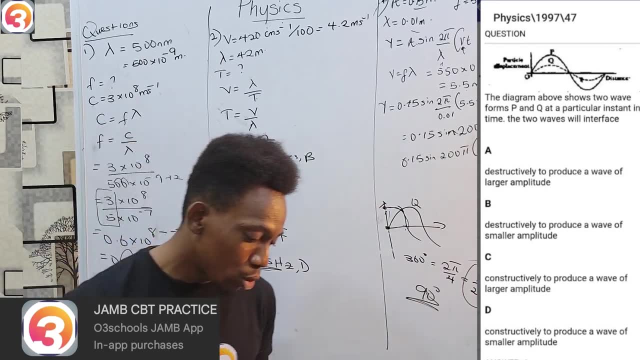 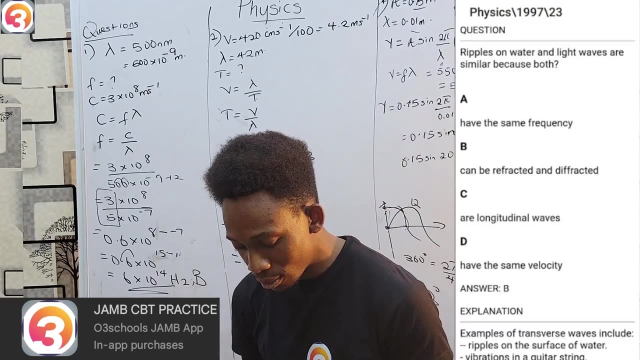 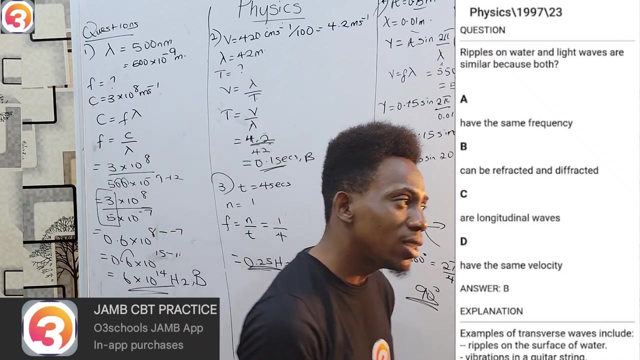 so we really go construct, I get the wave of larger amplitude. see, that's, that's ocean sea. and then, last but not least, last but not least, from the year 1997, question number 23: ripples on water and light waves are similar because boats, what? what is the?